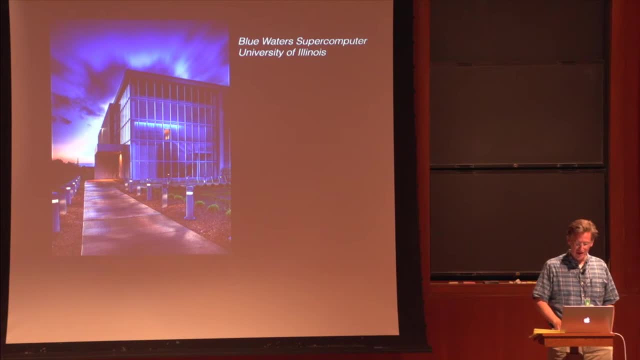 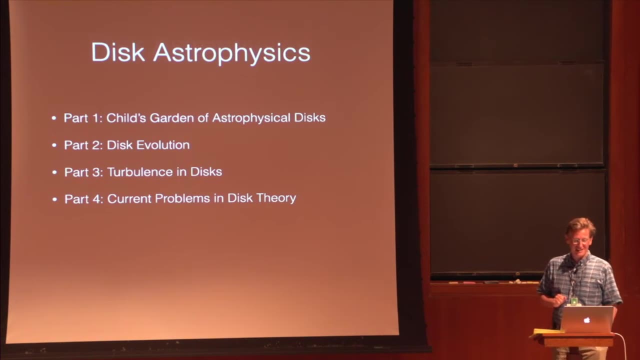 they can tell you the story at coffee. Okay, so the assignment is disk astrophysics, and here's the plan. I'm going to start out with some phenomenological motivation and go through a series of a list of interesting disk systems that motivate some of what I'm going to talk about. 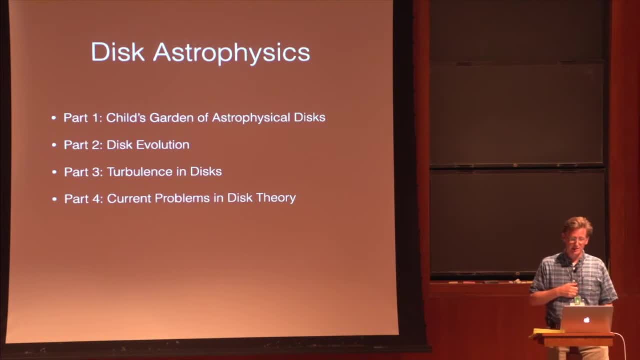 calculate many of the lectures that you've heard over the last week. Then I'll go on and talk about disk evolution, which is all about evolution of angular momentum, And I've been told I have to. let's see, I have a pointer here somewhere. I have to talk about the magnetorotational instability and dataset. 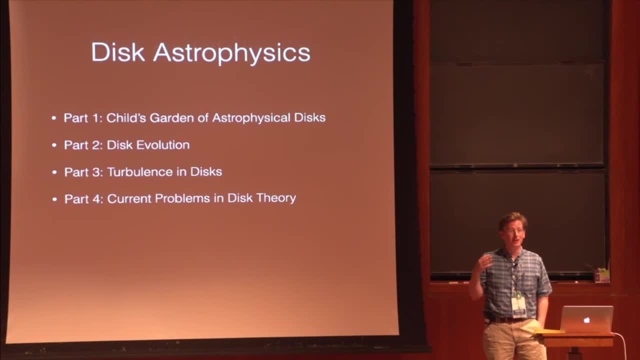 and then, if there's time, at the end I'll give a bit of a complete model study where you can take a look at all the issues versus most cried over time, And then I'll give a brainstorm and chat. That's interesting. I don't know about many of you. have anything left to do at this stage. We're in the centre of the 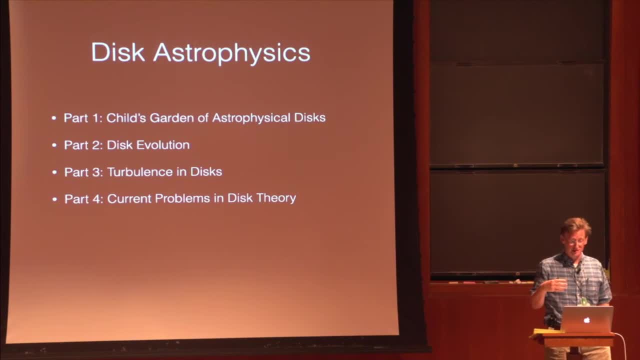 brief discussion of current problems in accretion disk theory. Okay, so first up a list of astrophysical disk systems. and again, the motivation here is that: the disks. the takeaway message is that disks are at the heart of many of the most interesting problems in theoretical astrophysics. Okay, so let me start with 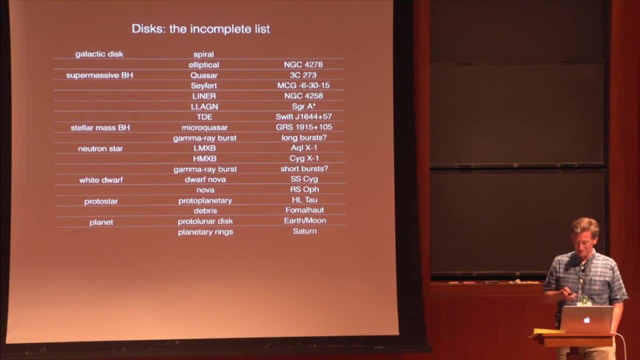 an incomplete list of disk systems ordered according to, with the exception of this, the central object around which the disk sits, And you can see that there. you know, we're very familiar with spiral galaxy disks, which should not be excluded from this list. They're unique in that they're very well. 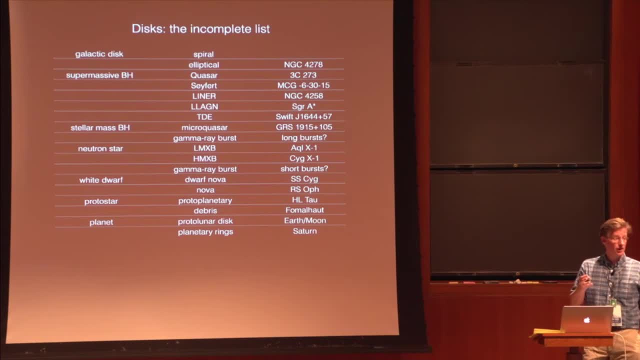 resolved disks. There's a lot of information about these disk systems and we can learn a lot from them that may be relevant to other disk systems. So, in particular, the disk of our galaxy has a approximately thermal magnetic field embedded in the interstellar medium and has a hot gas layer which extends up kiloparsecs. 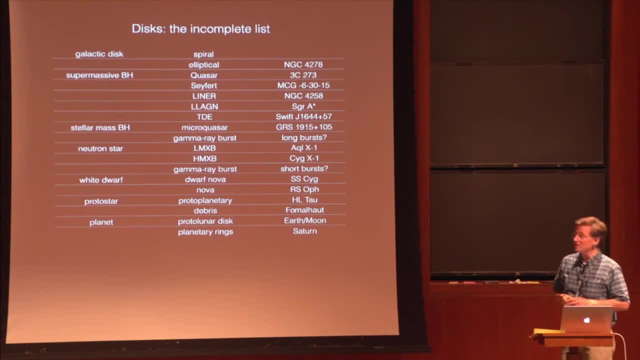 above the disk, and this may be a feature of other disk systems as well. There are also cold and warm disks in elliptical galaxies. As we now know, there are black holes in the center of almost all those galaxies, which give rise to a variety of 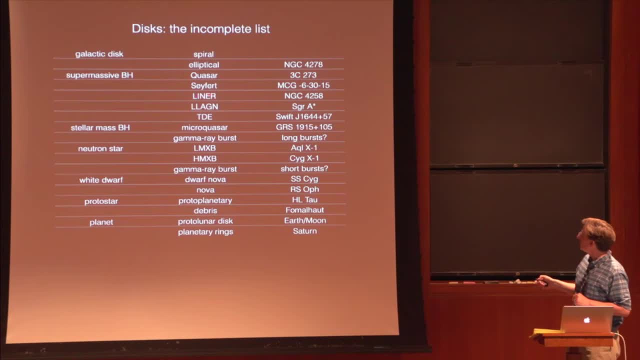 phenomena, from very luminous objects down to very low luminosity objects like the galactic center, the center of the Milky Way, Sagittarius, A star. There are also disks in a accreting stellar mass black hole systems, when there's enough gas, provided that we can. 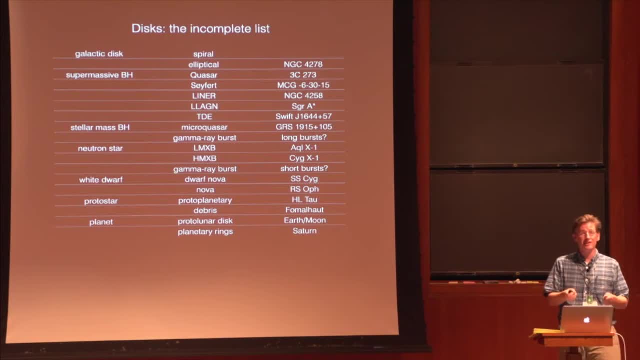 to the accretion flow around the black hole that we can actually see the accreting black hole And again that gives rise to a variety of phenomena. Neutron stars in binary systems also produce luminous disks, One of the best studied disk systems. 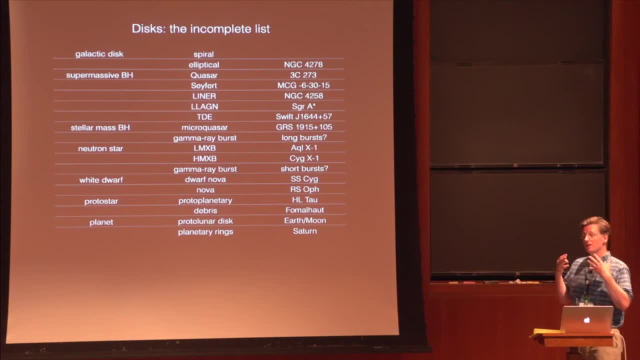 is the dwarf nova system, So interacting binaries with a mass-losing secondary or primary star that produces accretion through a disk onto a white dwarf, And I'll talk about an example of such a system in a moment. Protostars, protoplanetary disks. 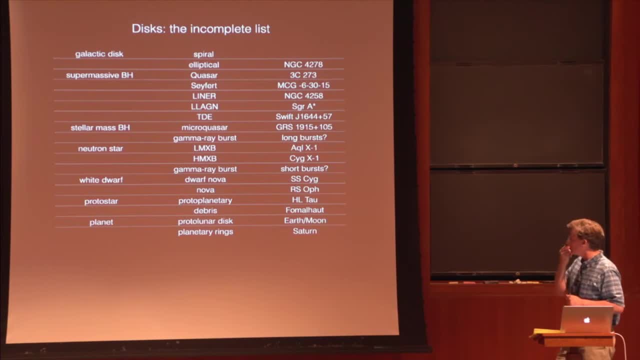 like the famous HL tau disk, also produce luminous disks, although, you know, it's not necessarily that they produce luminous disks. So in some cases the disks are observed not because they're generating energy through dissipation of internal turbulence. 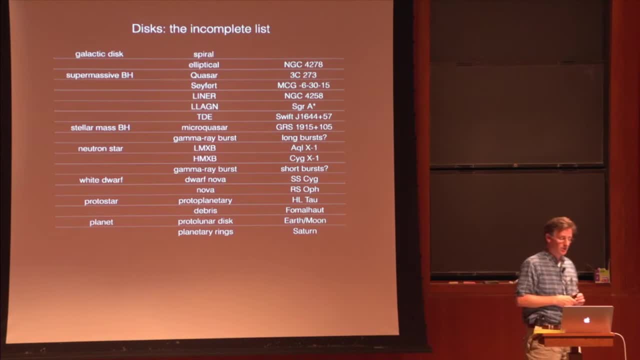 but because they are illuminated by their central star. There are also disks around planets, of course, and the protolunar disk is an example, the one that formed the moon, and debris disks such as Saturn's rings, which are not gaseous. 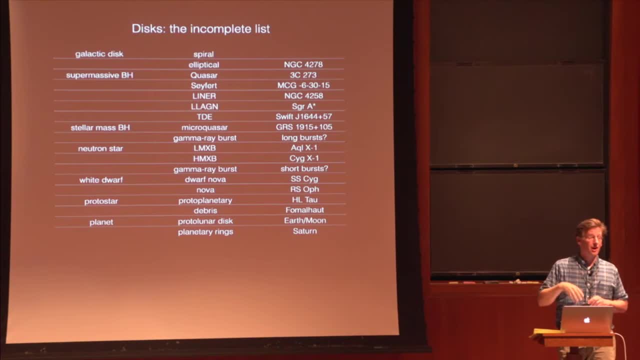 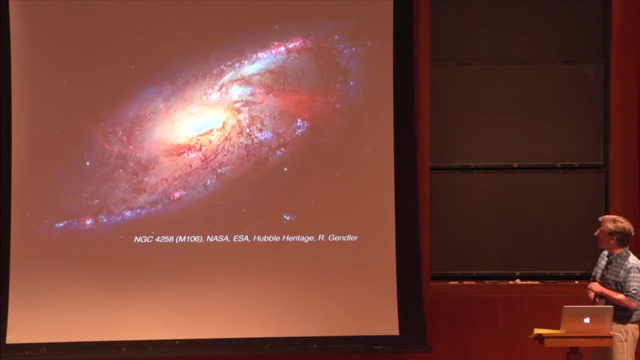 but which have many other features of disk systems, including, in the case of Saturn's rings, density waves which are found in several of these accretion disk systems. Okay, so let me talk about some specific examples. So this is the galaxy: NGC 4258,. 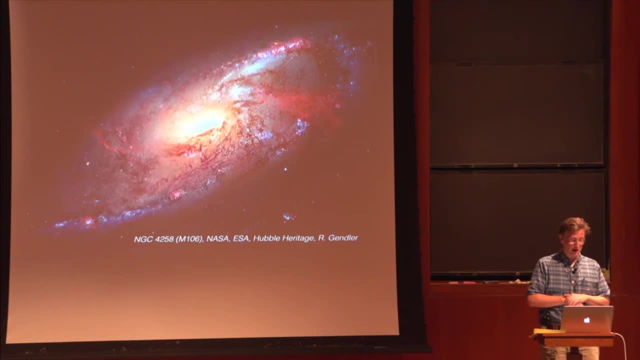 which is fairly nearby. This is the galaxy NGC 4258,, which is fairly nearby. This is the galaxy NGC 4258,, which is fairly nearby. Spiral galaxy. This is a Hubble Heritage image and it looks like a fairly regular spiral galaxy. 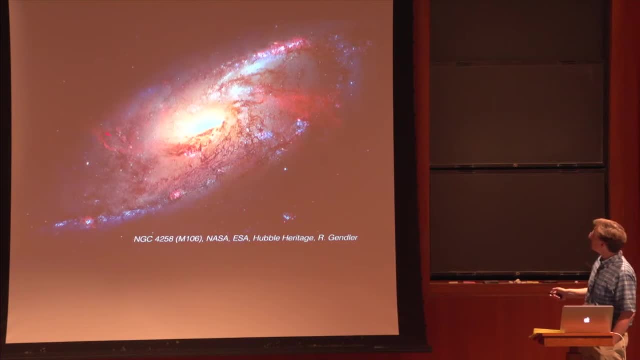 except there are a couple of features here which are seen- I believe this is in H-alpha- which were known for many years as anomalous spiral arms, And it turns out that those are a feature that results from emission of a jet from the nucleus. 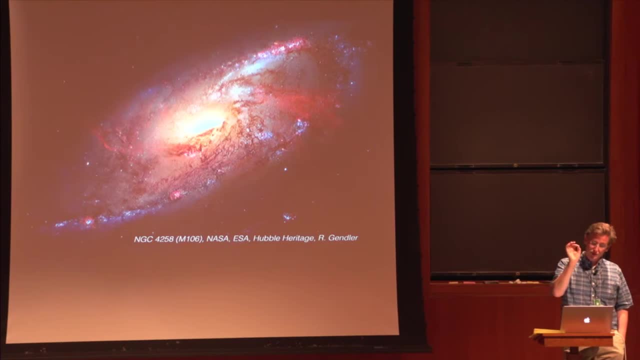 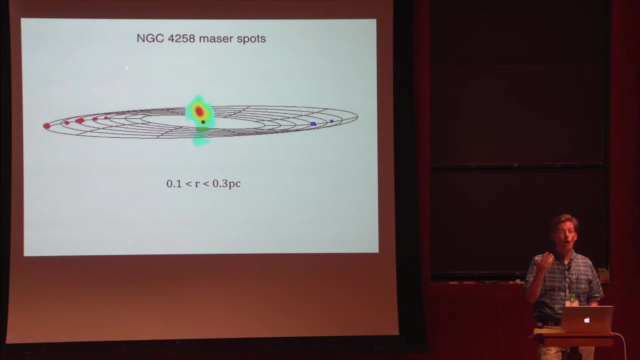 of this galaxy. Okay, so if one zooms into the center, through about 11 orders of magnitude in angular scale, one can observe, using very long baseline interferometry, a set of water maser spots on the sky. So this is from a nature paper from the late 90s. 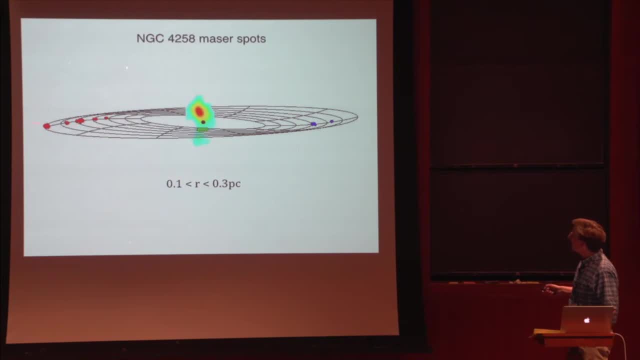 And the spots are here on the receding side. There are a few spots here in the center, and then there are a few spots here on the approaching side, And then the color here shows some radio continuum emission which is also picked up in the course of the VLBI. 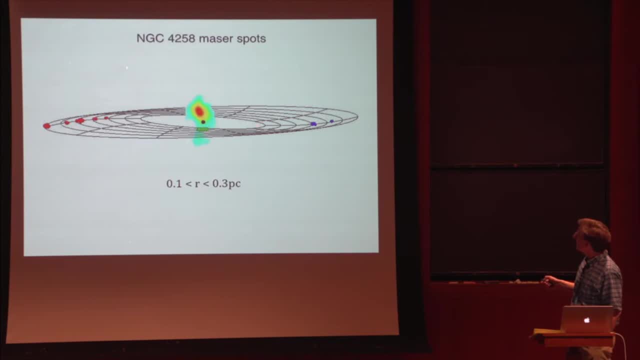 observation And the scale here. the physical scale is about .1 parsecs to about .3 parsecs, So very, very close to the central black hole, which has a mass of about four times ten to the seven solar masses measured very. 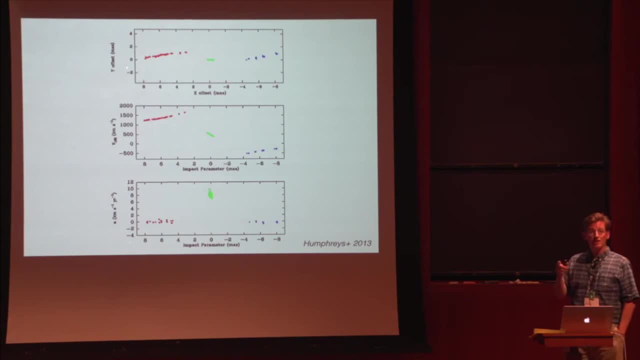 precisely through these maser spots. So the measurement- and this is from a more recent paper by Humphreys et al- is made using the positions of the maser spots on the sky. It's made using the velocity of the maser spots which turn. 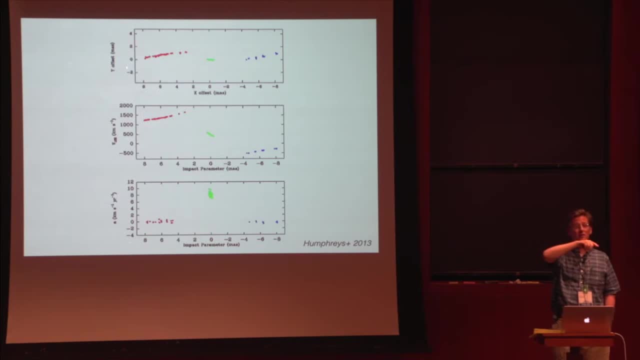 out to fall very precisely on a Keplerian rotation curve. So that tells us that this is a low mass disk around a central object, And then and actually also a thin disk, And then we can also measure the acceleration of the central maser spots. 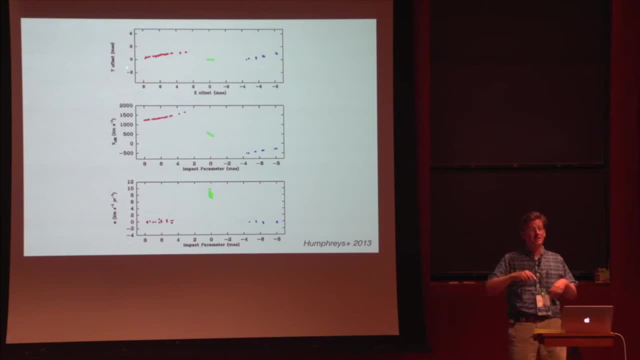 And then we can also measure the acceleration of the central maser spots. And then we can also measure the acceleration of the central maser spots, And the combination of the acceleration, the velocity and the and the angular positions on the sky allow one to infer the central mass and the distance to 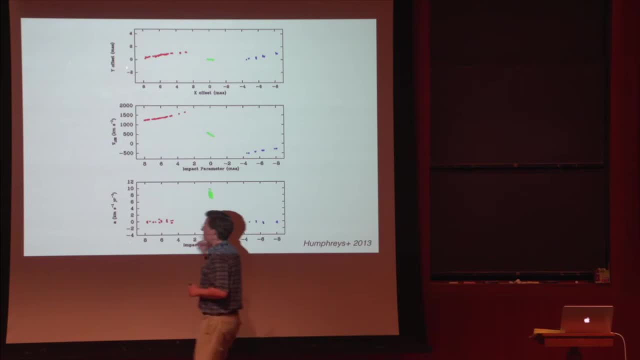 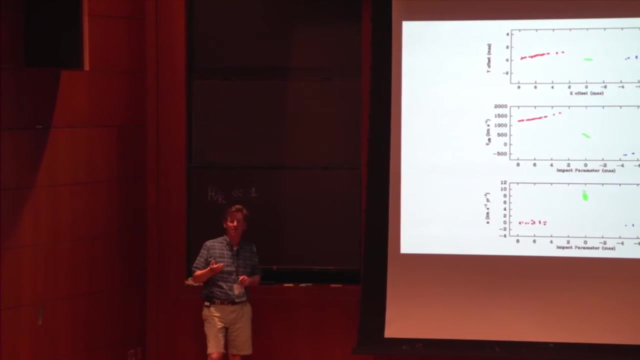 this object. So this turns out to play an important role. this, this system, turns out to play an important role in setting the the extragalactic distance scale and measuring the Hubble constant. So so this, this allows me to introduce a first dimensionless parameter for disks, which is the ratio of 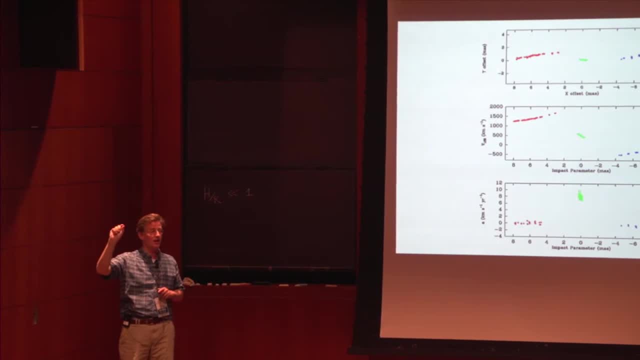 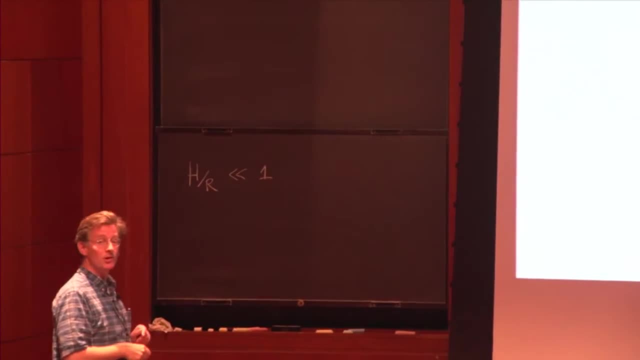 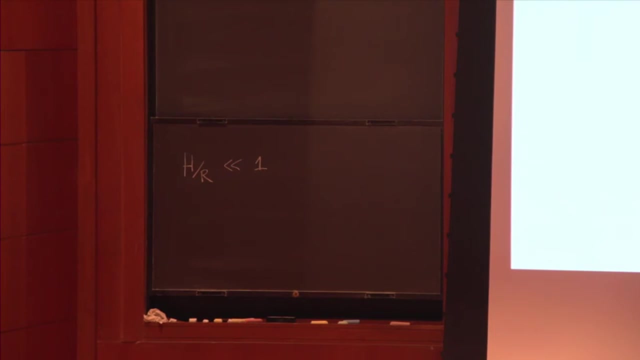 the scale, height of the disk, the thickness of the disk, characteristic thickness h to the local radius And in. in this system that ratio is of order 10 to the minus 3.. So the, the ratio is proportional to the, the sound speed in the disk divided by the. 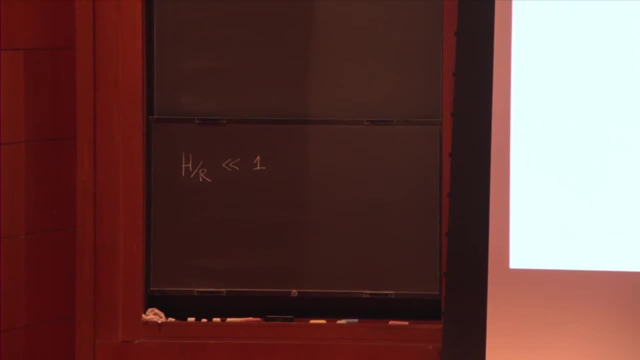 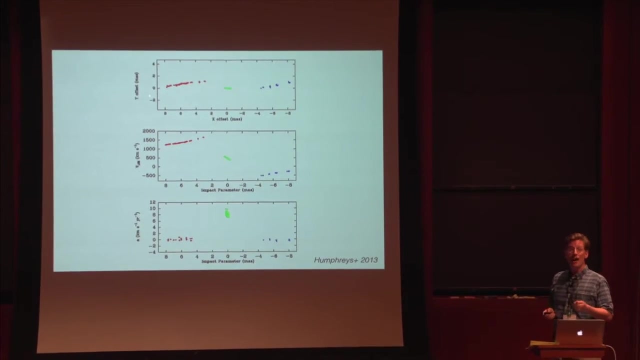 rotational velocity, And we know that the sound speed is a of order of a few kilometers per second, or a kilometer per second, And we can see that the rotational speed is of order 1,000 kilometers per second. Okay, So this is a a proof of the existence. 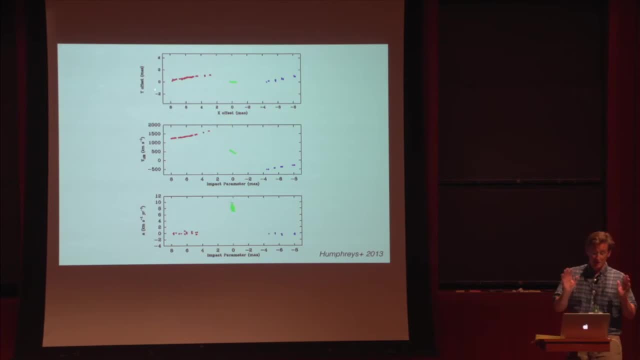 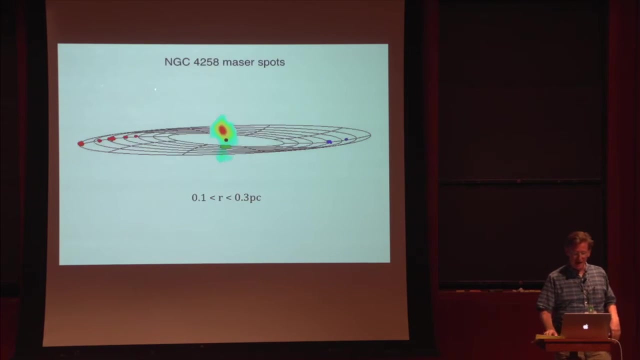 of thin disks in in a resolved system. It's also an example of a system where the disk is not lying in a a plane. It's not as one might expect in naive disk models. but just to go back to this illustration, 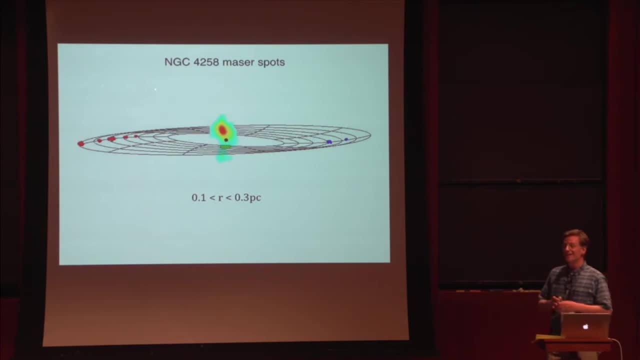 where there's a grid laid on top to guide your eye. the? the disk is made up of a series of rings which may be tilted and warped. So the? the warp is quite well constrained here. So another important feature of disk systems warps. So thin disk, warped disk. 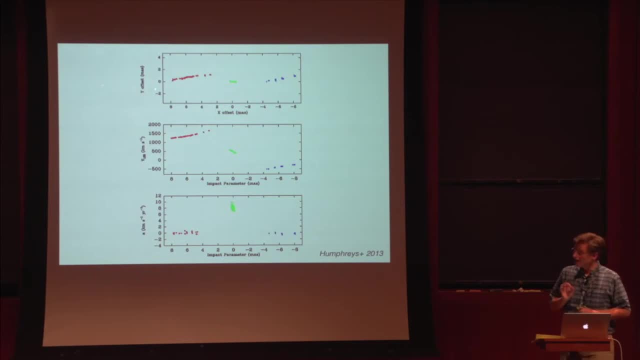 Okay, Another interesting feature of NGC 4258 disk is that we're seeing the maser disk far from the central object, So this far out. the accretion energy dissipated per unit area in the disk is very small and most of the heating of 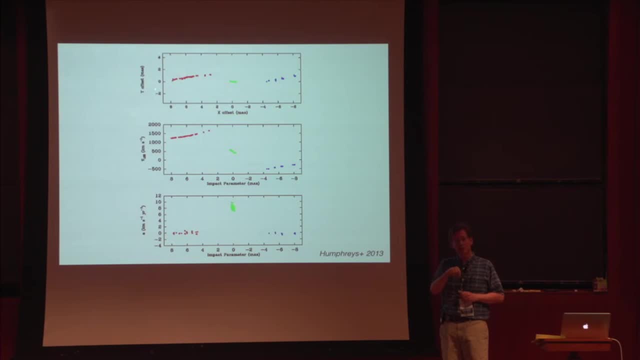 this disk comes from illumination, from the central accretion flow, So that's very important for understanding the thermodynamics of the maser emitting gas. Okay, Yeah, so the story is that you get maser emission along lines of sight where the velocity is coherent, along a significant path on the line of 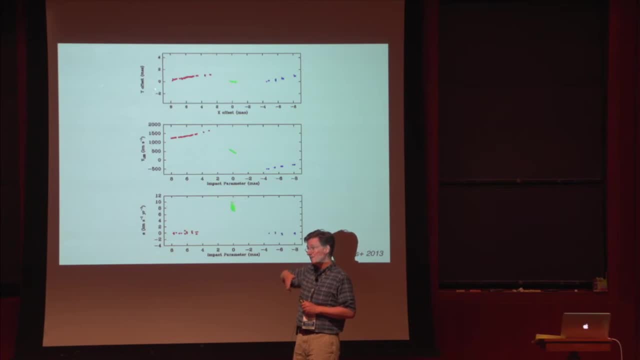 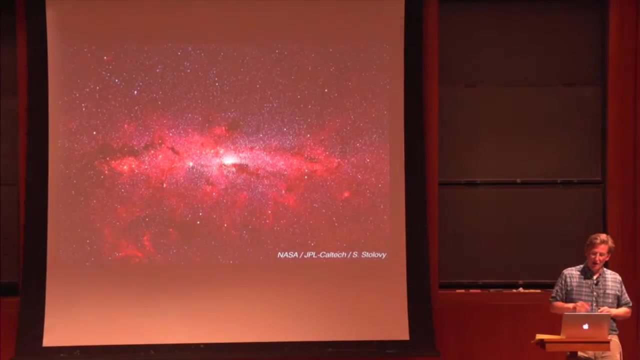 of sight, and that happens at the so-called tangent points, so along the the receding and approaching edge of the disk. yet there's also maser emission in the center, and that may be as a result of seed photons, for the maser produced by the jet that we don't see. okay, okay, next up is the center of the. 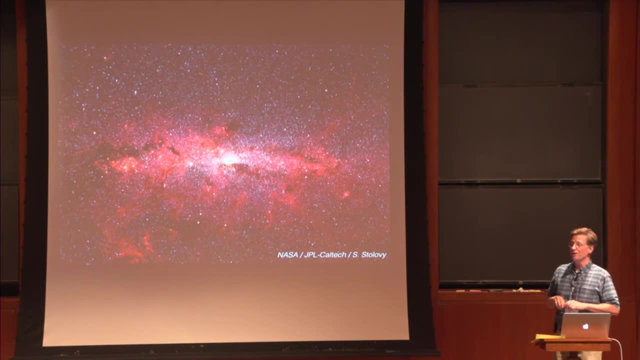 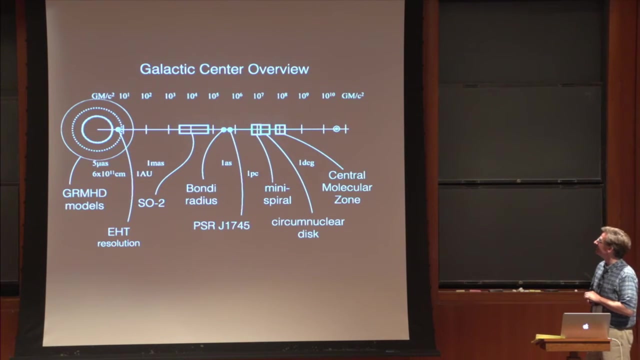 galaxies. this is a beautiful spitzer mosaic of the uh inner few hundred parsecs of our galaxy and if, if one zooms in. so i have a galactic center map here which gives the scale of things in units of gm over c squared the size of the black hole. 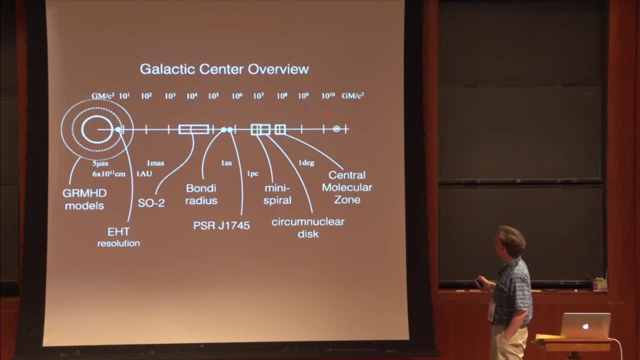 and, and we're out of here at a few 10 to the 10 gm over c squared. this, that image you just saw, is it about here? and then, if you zoom in by nine orders of magnitude, you get to the uh, the black hole, and uh, we know that there's uh an accretion flow around this central black hole that produces 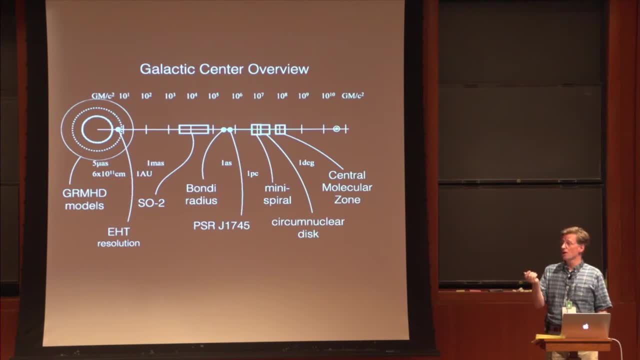 millimeter wavelength emission uh through synchrotron process and uh that synchrotron emitting accretion flow is a target system for the event horizon telescope. so i saw event horizon telescope mentioned in some of the notes but i don't know if anyone got to talking about it. can. 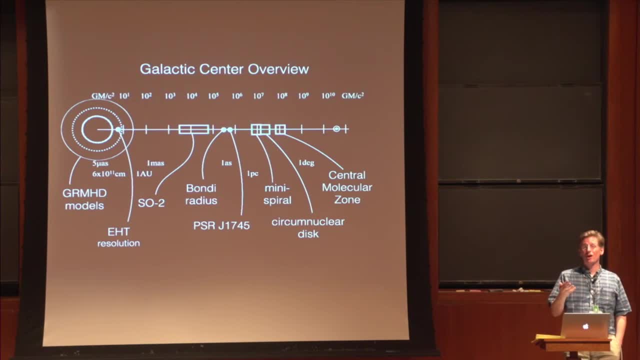 have you okay, very good. so event horizon telescope is a millimeter vlbi experiment. uh, so that will link together millimeter antennae from around the globe, the south pole alma in chile, south pole um sites in Hawaii and elsewhere, and it will be able to produce images of the accretion. 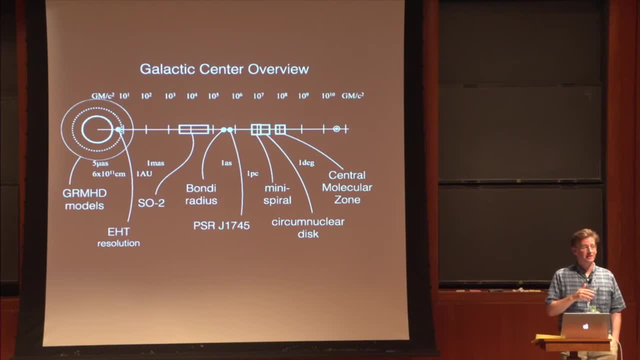 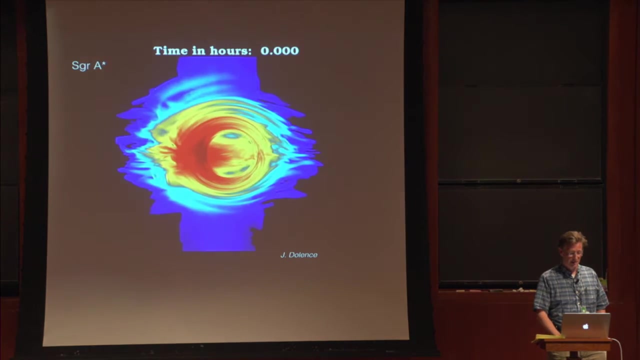 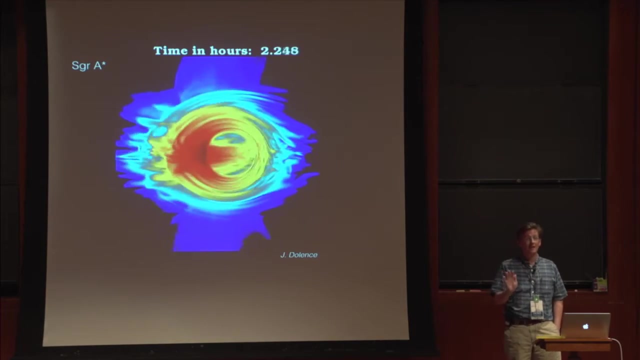 flow in the galactic center and in M87 at the horizon scale. So many people have been making models of these systems and I'll show you one model that came out of our group some years ago. So this is a millimeter wavelength movie of accretion onto the central black hole. 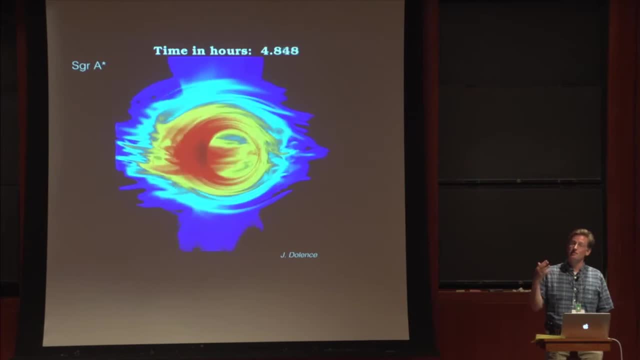 So this is a very interesting disk system, These resolved images, which won't be this nice, you know. if anybody wants to discuss it at coffee, I'm happy to tell you the saga of Event Horizon Telescope, but there will be information in the EHT images. 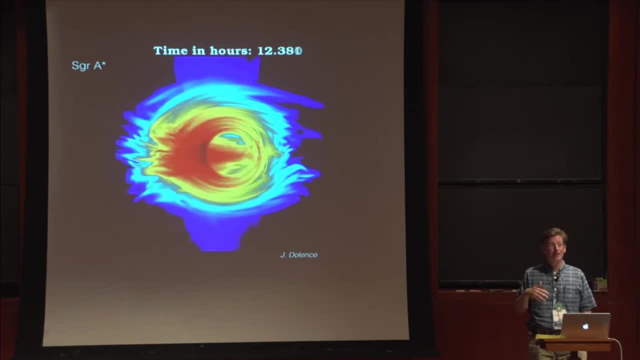 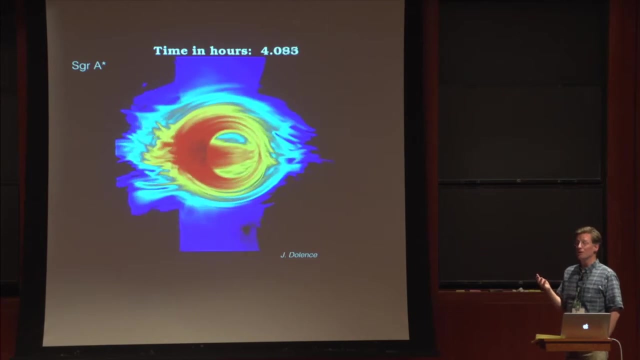 So this is an image about this accretion flow that will allow us to constrain, possibly, the characteristics of the emitting plasma. So where in the accretion flow is most of the emission produced around the jet? or in the disk? What do the fluctuations in the accretion flow measured by EHT tell us about turbulence? 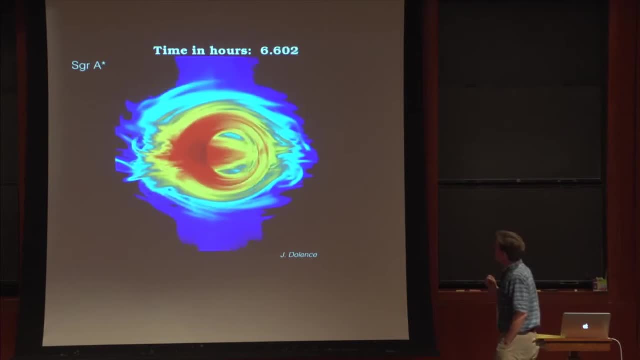 in disks. Okay, So this is probably collisionless plasma, So a plasma at temperatures of maybe 10 billion degrees, at very low densities sort of number density electrons around 10 to the sixth, And under those conditions the mean free path to Coulomb scattering is very large. 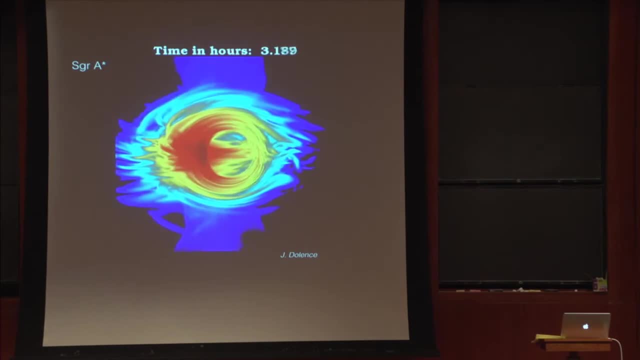 And this allows me to introduce another dimensionless number, which is the Knudsen number, which is the ratio of the mean free path. Okay, To the scale of the system, And in Sagittarius, A star in our best models, this ratio is around 10 to the 5.. 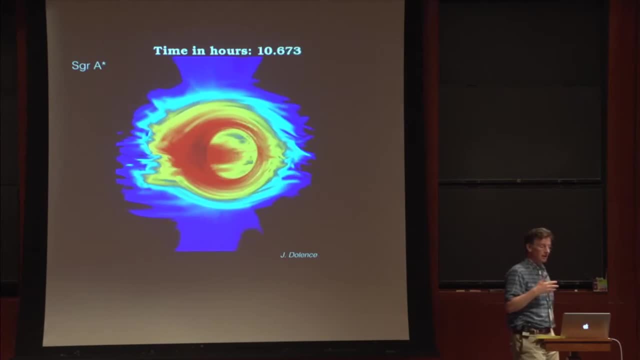 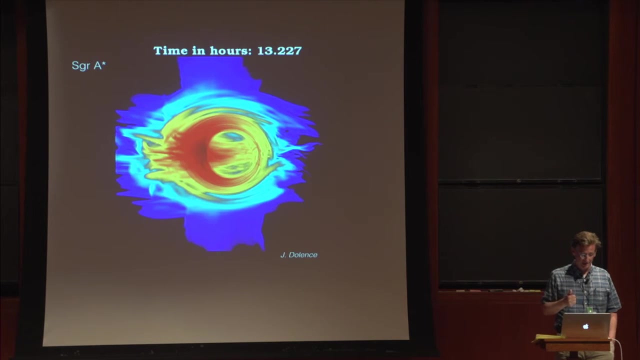 So this is an interesting system for applications of work that Matt Kuntz and others are doing in studying the evolution of turbulence in collisionless plasmas. Okay, So this is also a system where the Alfvén speeds are relativistic, And so it's also a venue for applying relativistic MHD, as you learned about from Lewis Lehner. 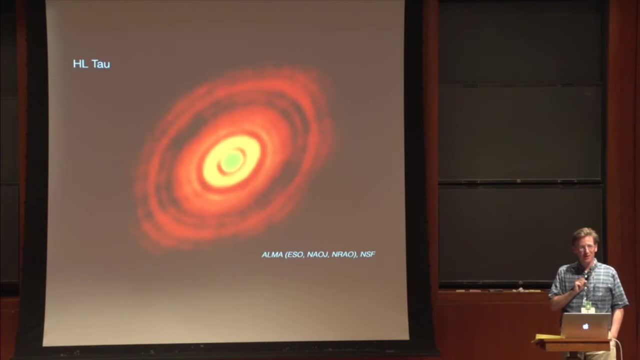 Okay, I've got two more disk systems to go, So this is the famous HL tau disk. HL tau is a disk. Okay, It's a disk. that's a nearby protostar. it's about 140 parsecs away. that has been imaged. 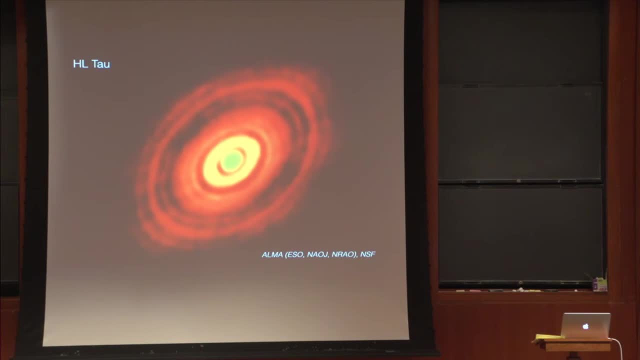 in millimeter continuum emission by ALMA, And what we're looking at here is thermal millimeter emission from dust that's embedded, presumably, in a gaseous disk. So the central star here is somewhat less than a solar mass, And the disk may be perhaps a tenth to a few tenths of the mass of the central star. 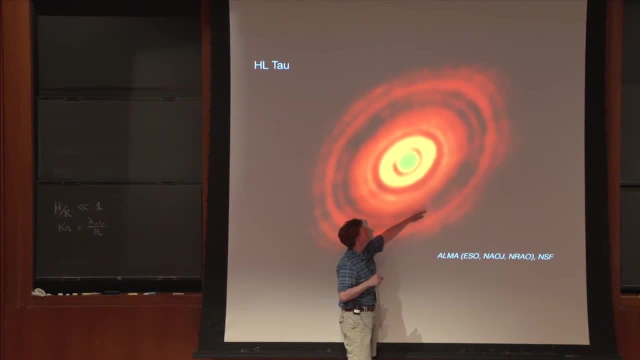 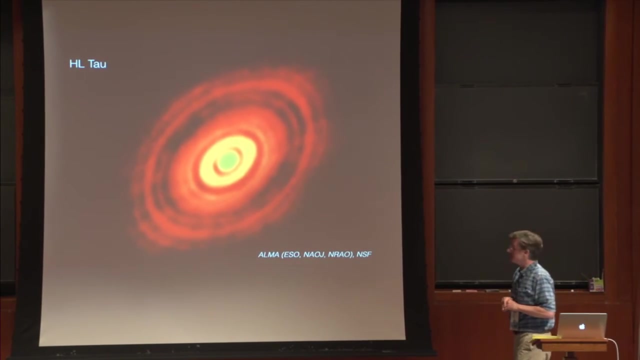 And to give you a sense of the scale, I think the first big dip in brightness here is at about 50 astronomical units. Okay, So this is a disk system that may be forming planets and that may be gravitationally unstable, Okay, 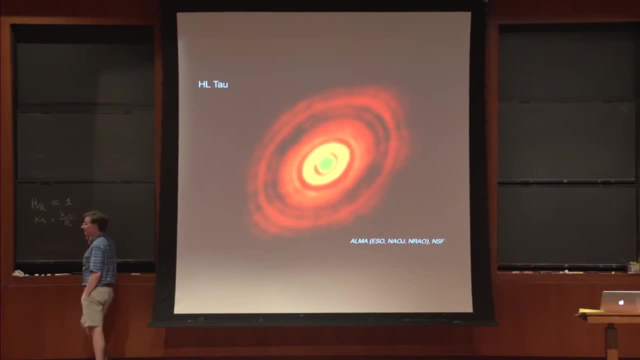 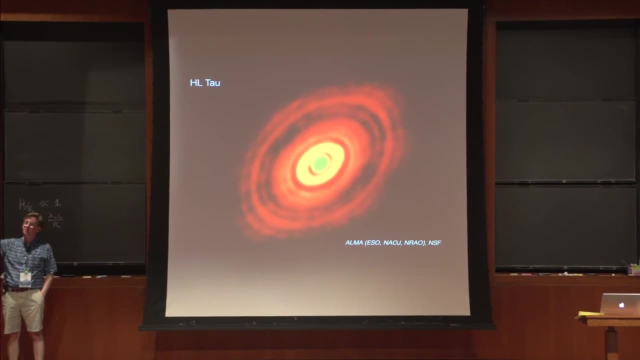 In addition, cold disks like this one. so the temperatures in these protostellar disks are governed by external illumination. So the temperatures are similar to the run of planetary temperatures in the solar system. So at 50 AU the temperature is somewhat less than 100 Kelvin. 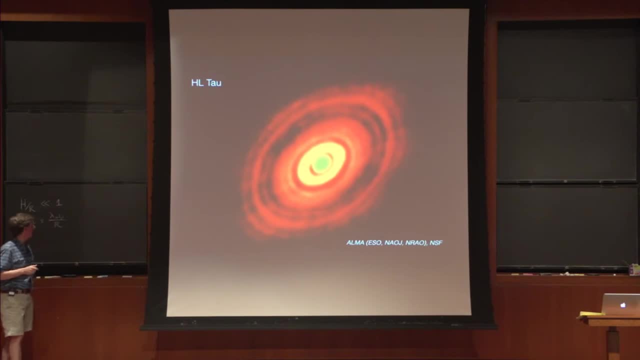 So these are cold disks, possibly self-gravitating. So let me introduce two more dimensionless numbers, Okay, Okay, So one is the magnetic Reynolds number, which allows you to assess the importance of non-ideal effects in the plasma around a young star or in other systems. 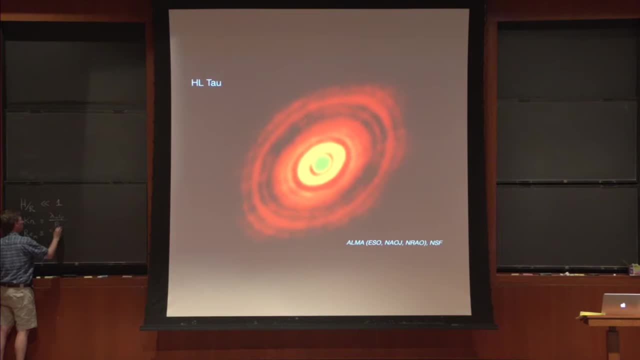 And this is defined as the ratio of a characteristic diffusion coefficient, which is the sound speed multiplied by the scale height. So this is something with the dimensions of a diffusion coefficient divided by the resistivity. So this is the electrical resistivity of the plasma. 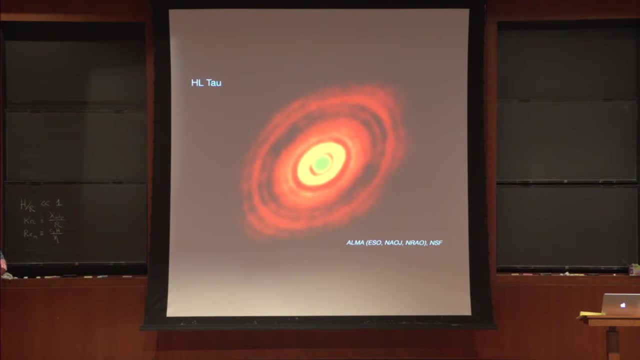 And that's high in these systems because the temperatures are low and the abundance of free electrons, of electrons in the gas phase, is low. Okay, So it turns out that in the regions of this disk, Okay, Okay, So in the regions of this disk that we can resolve with ALMA, it's likely that this 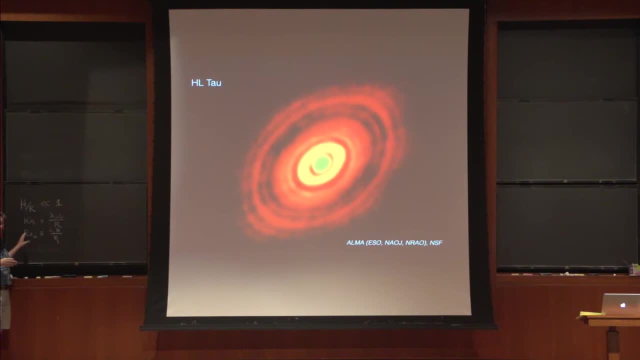 magnetic Reynolds number is substantially less than one, And so large parts of the disk may be decoupled from the magnetic field. Okay, The other important dimensionless number in describing systems like HL tau is the Tumray-Q parameter, Which measures the importance of self-gravity in the disk. 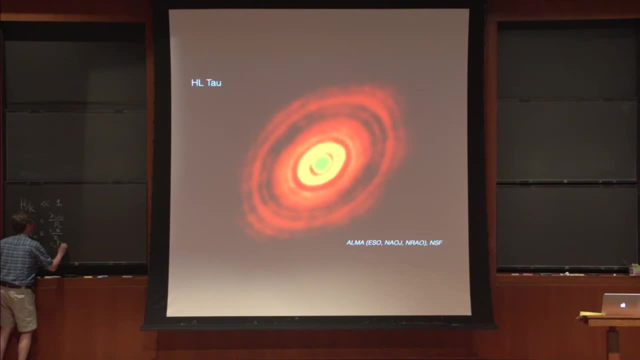 So this in a Keplerian disk is the sound speed multiplied by the orbital rotation frequency, divided by pi times Newton's g, times the surface density sigma of the disk. And when this parameter is less than or of order one, then self-gravity is less than. 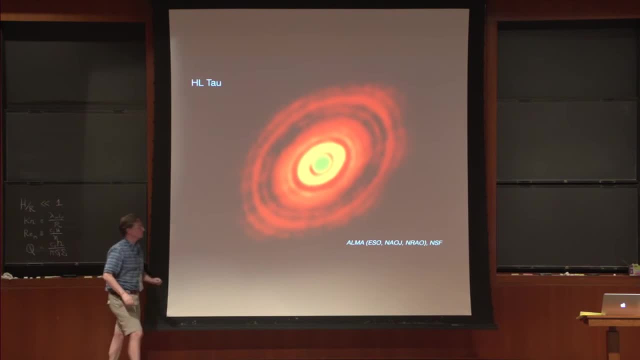 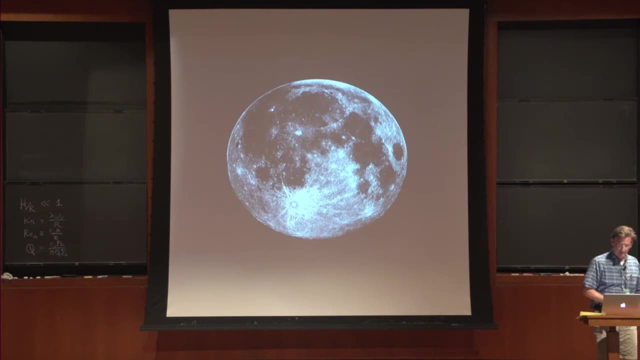 one. So the self-gravity becomes important in the disk. Okay, The final disk. So most of you look at this and don't see an accretion disk, But when I look at this, I do. I'm very interested in the problem of formation of the moon. 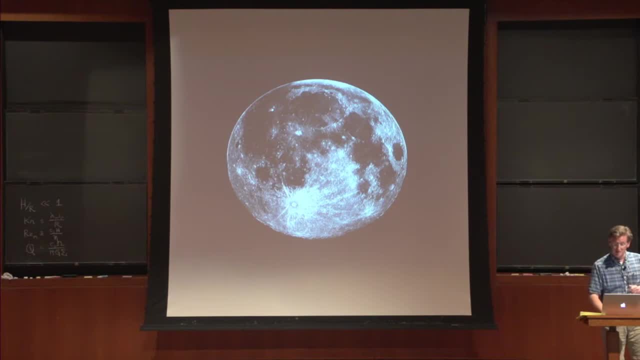 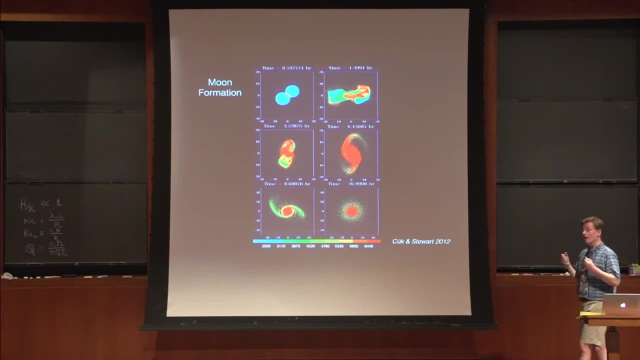 And Okay. So, as some of you probably learned in introductory astronomy, the moon is thought to have formed from a collision between an impactor and the proto-Earth, And this impactor hits the Earth and then lofts material into orbit around the young. 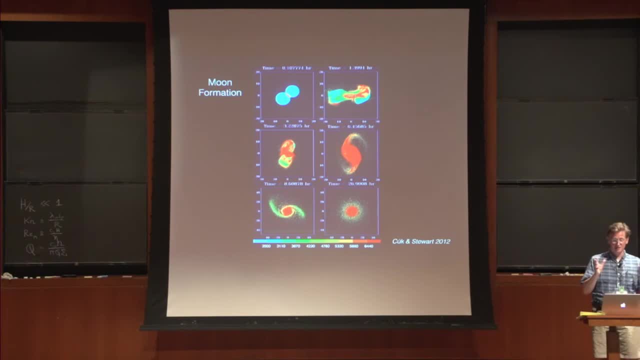 Earth that settles into circular orbits. Okay, And this is an SPH simulation of one of these collisions from Cook and Stewart. This is an unusual model with equal mass impactors And you can see as time goes on, there's something really bad that happens after the collision. 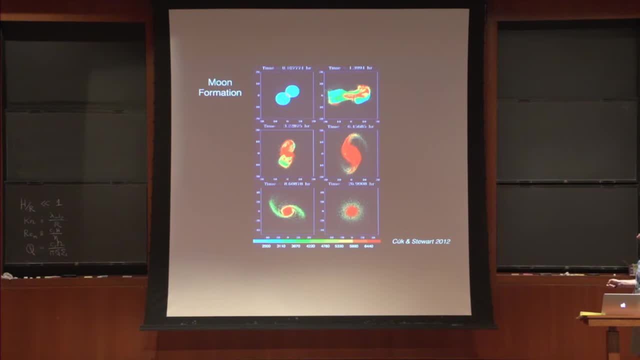 And then things settle down after a few hours and there's a disk of particles that are color-coded here by temperature- So in this case the temperature is around 4,000 Kelvin- that are orbiting the young Earth, And this is another interesting disk system where the magnetic Reynolds number may play. 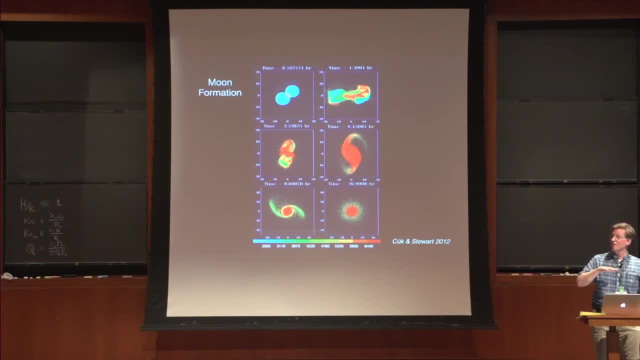 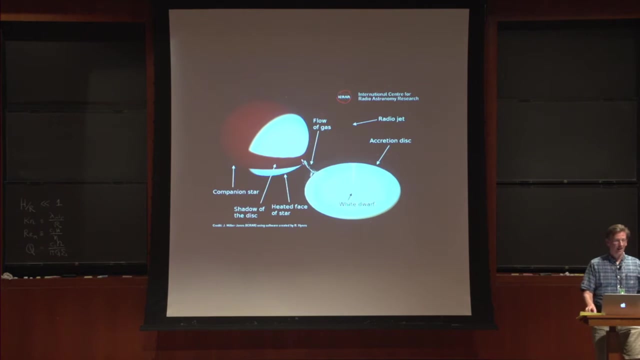 an important role. So initially the disk may have zero coupling to the magnetic field And later in its evolution it may have stronger coupling to the magnetic field. Okay, Sorry, I have one more disk system to go. This is SS Cygni. 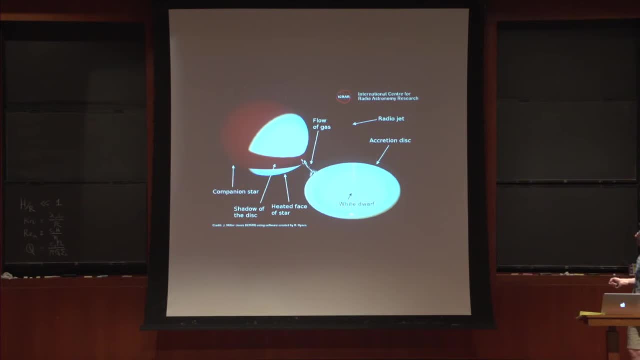 So this is an artist's conception of SS Cygni. SS Cygni is a dwarf nova system. So there's a companion star that is overflowing its Roche lobe and producing an accretion disk around the primary white dwarf, And we now know that this system produces a radio jet. 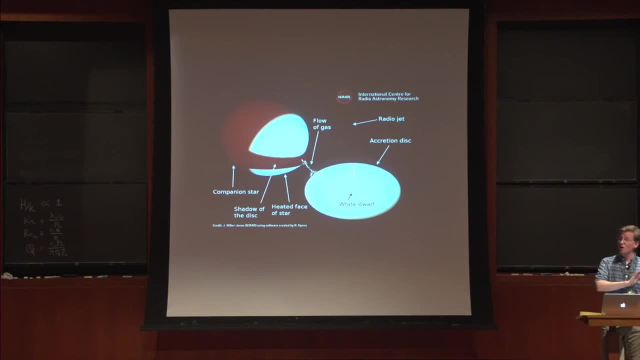 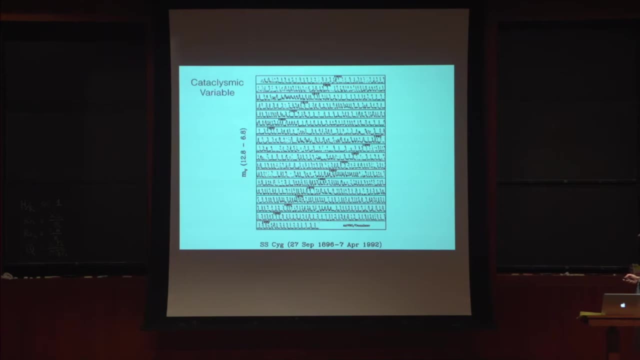 Okay, So this system has been known for more than a century to be variable And this is a light curve from the American Association of Variable Star Observers that goes back to 1900. So you can see this system quiescent in the visible and then every few weeks it goes. 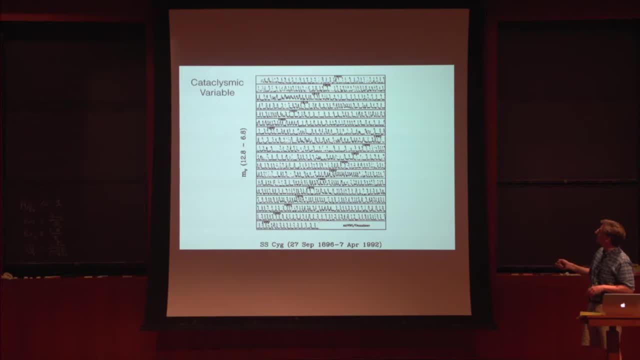 into an outburst and then decays Okay, And this has been going on since William McKinley was president of the United States, And it will continue going on even if Donald Trump becomes president of the United States. So these outbursts are believed to be due to – I've just broken the Trump rule. 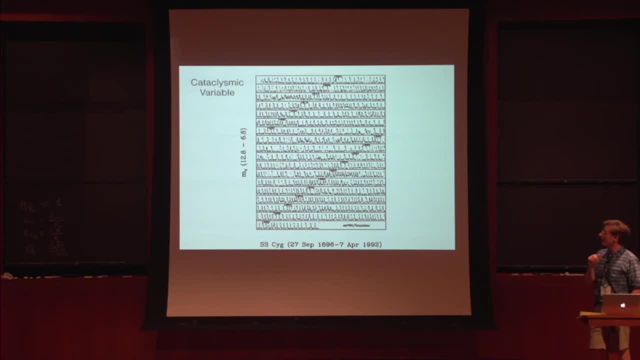 It took me about 20 minutes to mention Donald Trump. Okay, So these outbursts are believed to be due to an instability of the accretion disk. So it wants to accrete at a rate at which there is no steady disk – no stable, steady. 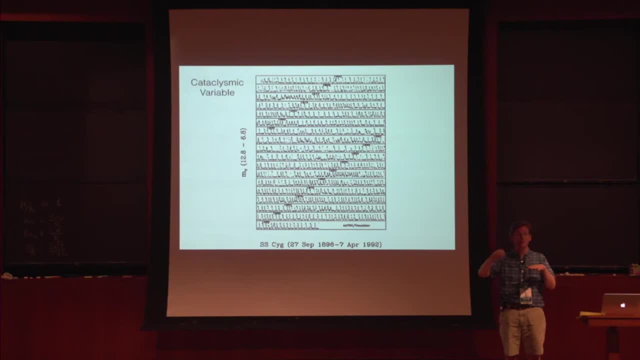 disk solution for accretion from the outer edge of the disk into the surface of the white dwarf And, as a result, it oscillates between an excitation disk- Okay, It oscillates between an excited state where accretion is very rapid, and a quiescent. 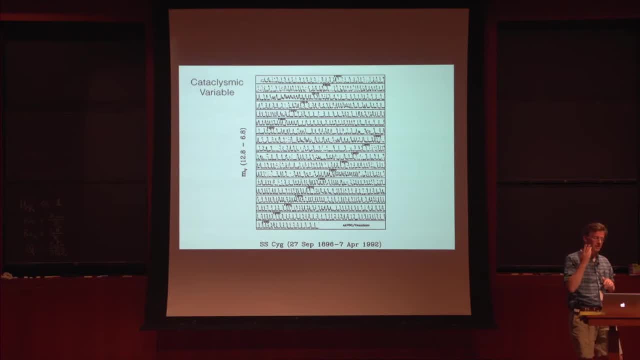 state where accretion is slow, And these are model disk systems in the sense that they change on time scales that we can access easily with observations. We can learn a great deal about these systems from eclipse mapping so we can evaluate the run of temperature. 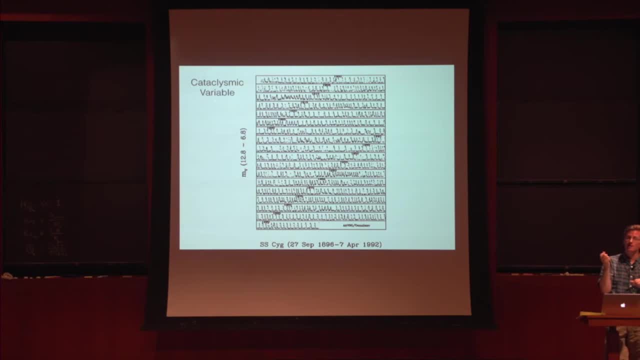 We can learn a great deal about the temperature inside the disk using, for some of these systems, the passage of the secondary in front of the disk. So the time series of brightness of the system as the secondary passes in front of the disk allows one to infer the run of surface brightness of radius. 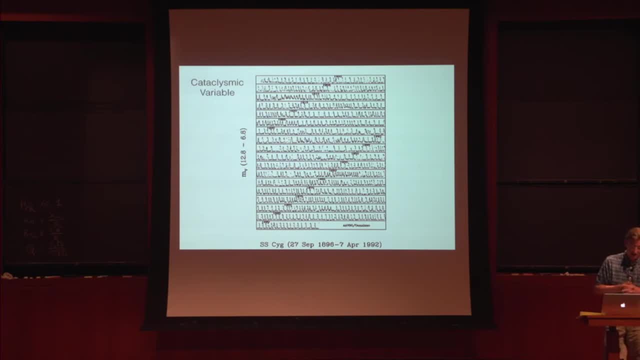 Okay, So to connect this to the – some of the topics discussed here: In computational plasma physics, this system may have a low magnetic Reynolds number when it's in quiescence And it is probably MHD turbulent when it's in outburst. 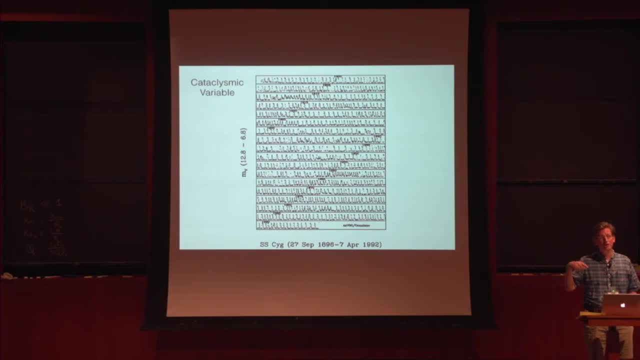 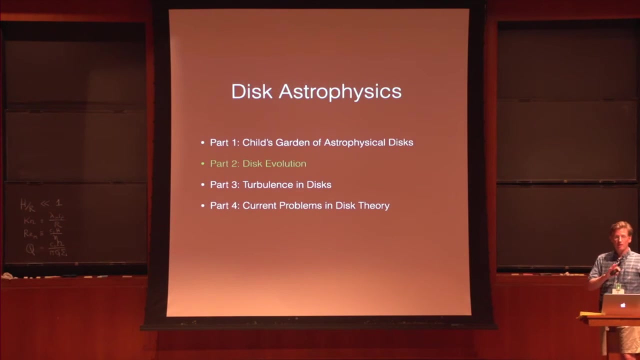 And, as I'll mention later, the convection that occurs in the course of the outburst may enhance the strength of the magnetic field that we believe is present in the disk and lead to enhanced transport of angular momentum. Okay, So that's a very brief overview of disk phenomenology and some interesting problems in accretion. 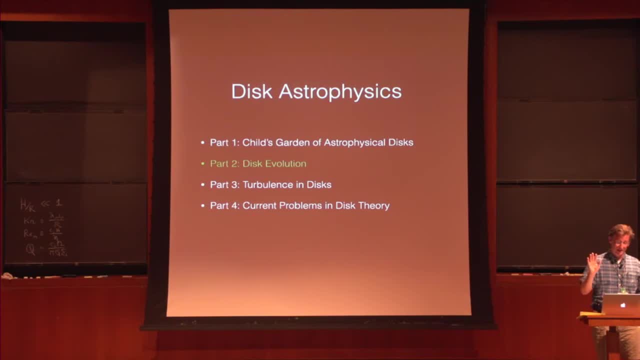 disks. So the takeaway there is that disks are central to many interesting problems in astrophysics. So I'm going to stop there, Thank you. So now I want to go on to talk about disk evolution And this is all about angular momentum. 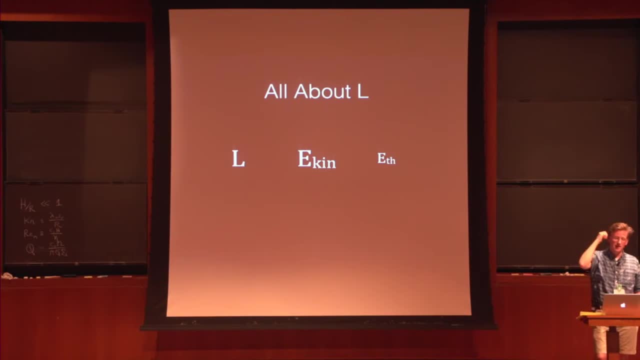 So disks are common in astrophysics because of a common physical process, which is that angular momentum is approximately conserved While – so I'm going to go back to the real world, But the first thing is this: The internal energy of the plasma is easily radiated away. 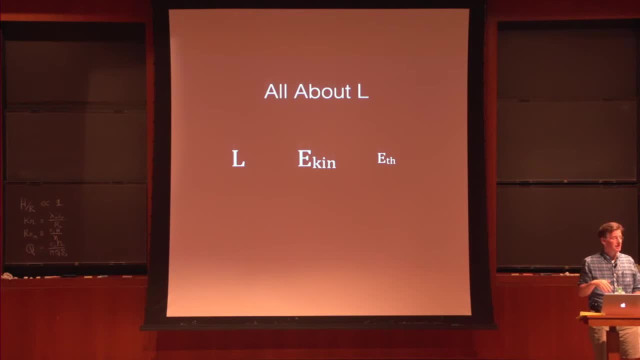 So the time scales for evolution of angular momentum are long and the time scales in many systems for evolution of the internal energy are short, And I have a little animation of this here. So let's imagine that we throw some plasma into orbit around a central object and it 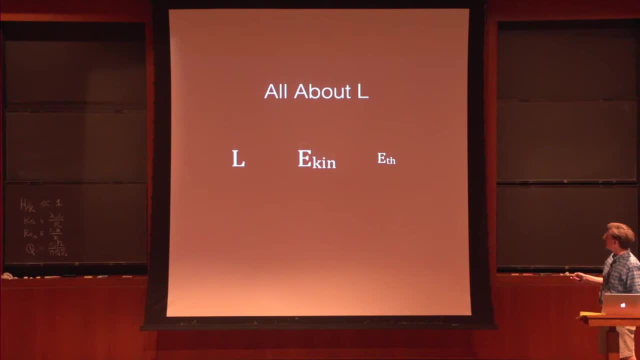 has some angular momentum L and some kinetic energy. Let's imagine that we throw some plasma into orbit around a central object and it has energy and it's cold. so it has a thermal energy which is significantly less than the kinetic energy in the frame of the central object. okay, so here's the 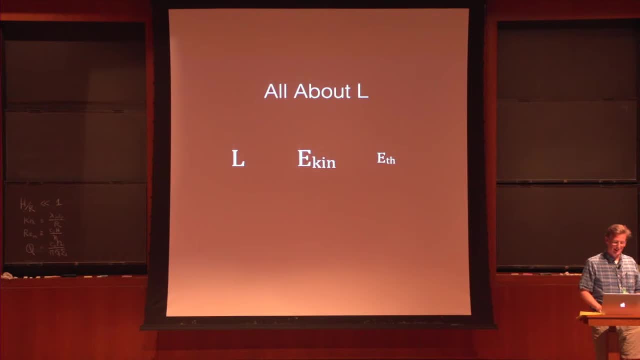 animation. okay, did you see that? so? so there, there are shocks that are produced as the gas settles in to an orbit around the central object, and those shocks change kinetic energy to thermal energy. the kinetic energy is dissipated, then, over time, the thermal energy is radiated away, while the angular momentum is. 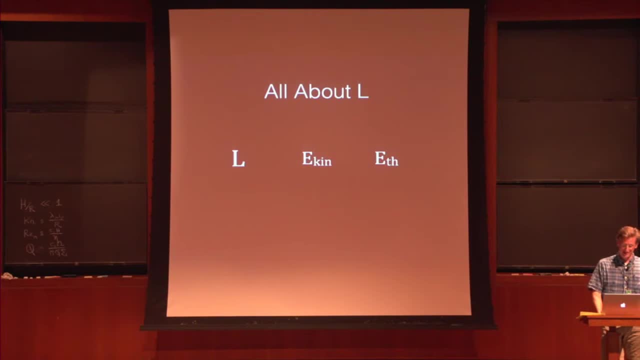 approximately conserved. so it's my next animation, okay. and then, finally, the thermal energy becomes quite small compared to the kinetic energy of the disk in in orbit about the central object and we have a thin disk, okay. so this happens in in many systems in astrophysics, in NGC 4258, perhaps in 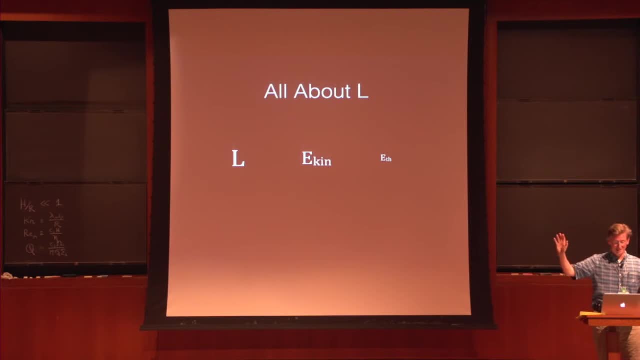 the protolunar disk in in Saturn's rings, in many, many places in astrophysics. okay. so because of this, this disk evolution, understanding disk evolution is all about understanding the evolution of the disk angular momentum. okay, but I'm not going to go into that. so before I go on to that, let me just review some time. 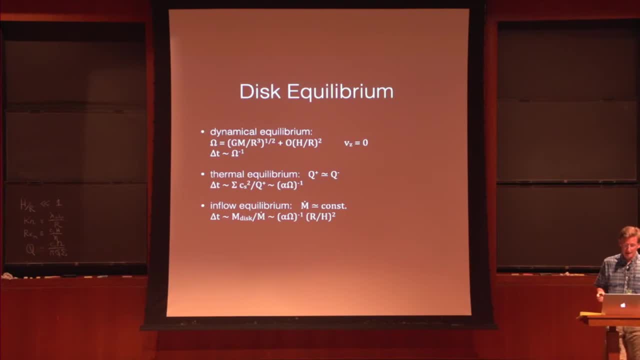 scales for disk equilibrium. so in a thin disk the dynamical equilibrium is reached on a time scale of order, the dynamical time. and the dynamical time is characterized by the orbital frequency, Omega of the of the plasma and orbital about the central object, And that orbital frequency is approximately. 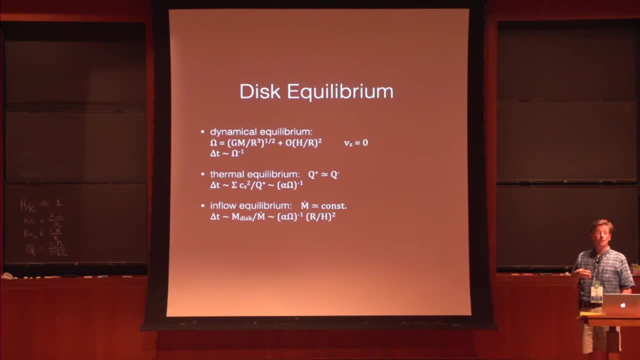 the Keplerian orbital frequency for a disk which is not substantially self-gravitating, plus a correction which is only of order h over r squared, So for a protoplanetary disk, for example, which has h over r of order 1, 10th. 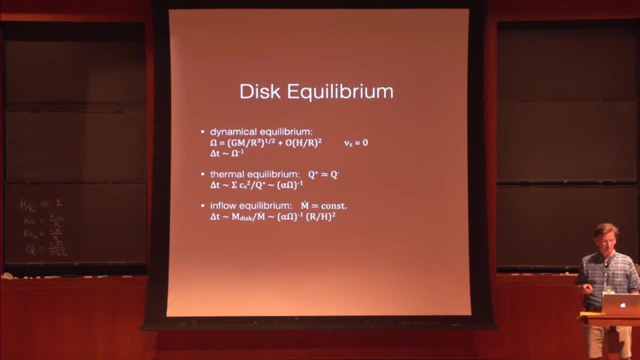 that correction to the orbital frequency is only of order 1%. okay, The disk also settles into hydrostatic equilibrium in the vertical direction, And that allows us to estimate the scale height h that I introduced over there, And I won't derive this, but the scale height. 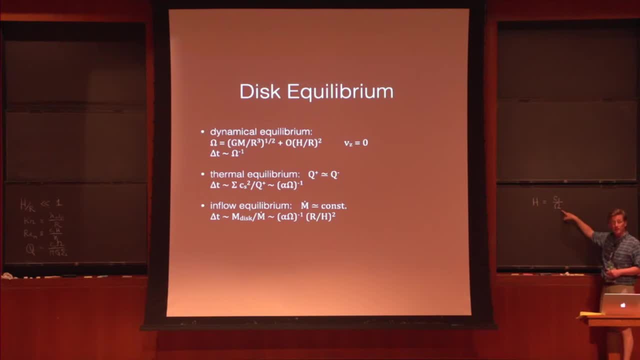 is proportional to the sound speed divided by the rotation frequency. Okay, So this in a gas pressure dominated disk, so a disk like a protoplanetary disk, where the pressure is dominated by the gas pressure, as opposed to a disk close to a black hole. 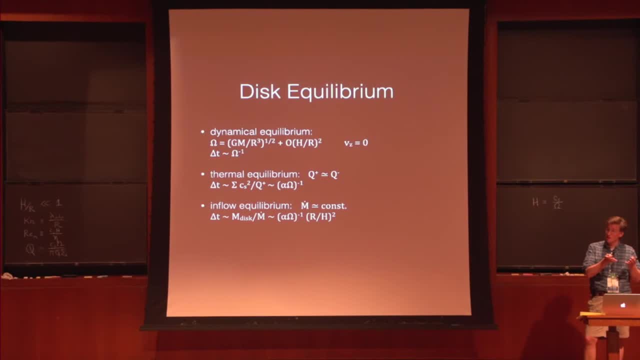 that's accreting rapidly where the pressure is dominated by radiation pressure. Okay then, in gas pressure dominated disks, the sound speed is proportional to this square root of the temperature. Okay, all right, so the dynamical equilibrium is achieved on of order of the dynamical time. 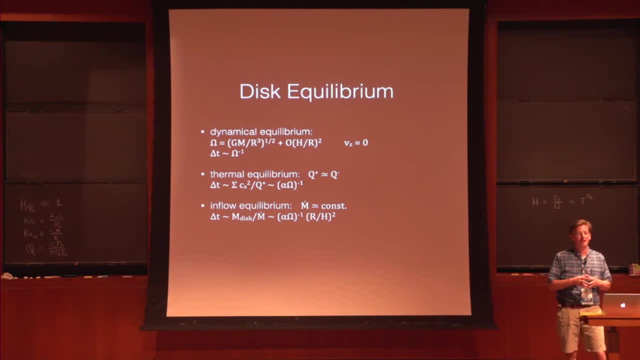 Although let me just give a caveat to that. So it's possible that there are long lived excitations of the disk, so it can be eccentric. So it's possible, instead of having circular orbits around the central object, to have eccentric orbits, although to lowest order in the eccentricity. 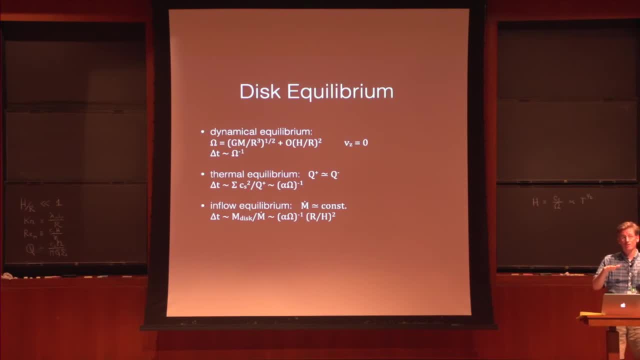 that doesn't change things very much. And then, of course, as we saw in the NGC 4258 disk, it's possible to have tilts and warps of the disk. Okay, so the next piece is thermal equilibrium. So this is entirely analogous to what you learned. 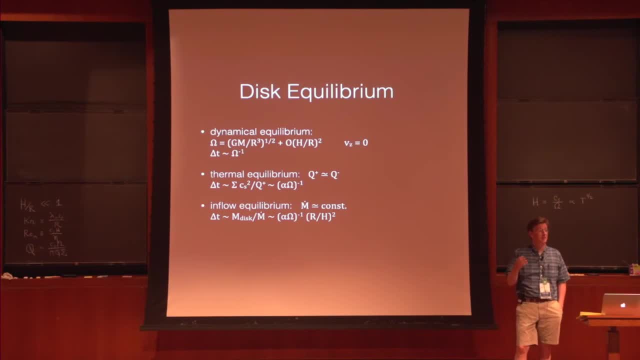 in stellar structure. Okay, so it's the same set of models that apply to, or the same set of equations, basically, that apply to, disk equilibrium. So thermal equilibrium is achieved when the heating rate is balanced by the radiative cooling rate. Okay, so the heating in some disk systems. 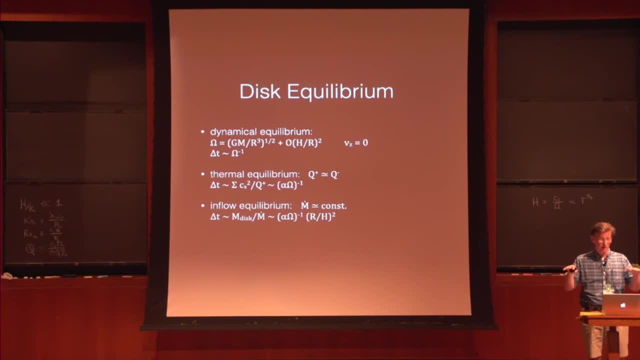 is dominated by internal friction related to dissipation of turbulence And, unlike stars, that is not concentrated at the center of the disk. that dissipation may occur throughout the vertical extent of the disk And the best evidence is that it does, as I'll show you later. 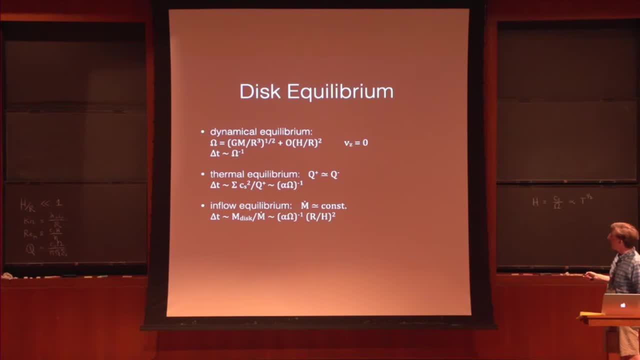 So that is in equilibrium, balanced by the radiative cooling And in optically thick dusk that's just given by sigma-t effective cooling rate. So in an optically thick disk that's just given by sigma-t effective cooling rate to the fourth at the surface of the disk. so just like a star. 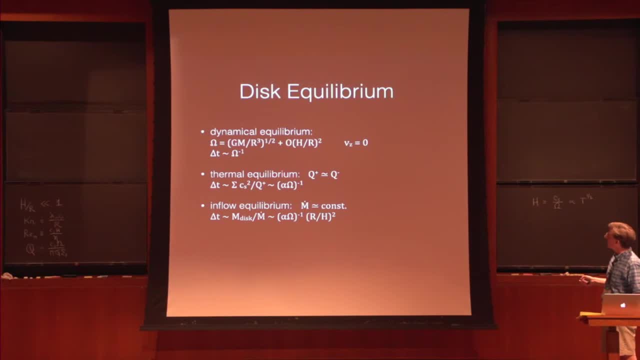 So that equilibrium is achieved on the thermal time scale and we can characterize that according to the rate at which energy is dissipated in the disk. And I'm now going to introduce this alpha parameter, which is very important in disk theory, which describes the intensity of turbulence inside the accretion disk. 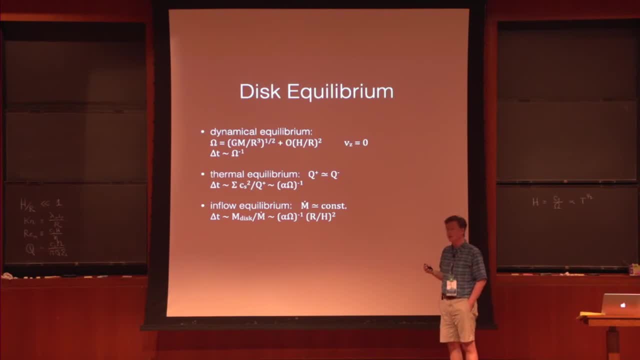 So the heating rate is simply assumed to be proportional to the local dynamical time, And the constant of proportionality is alpha, And so this is almost definitional. So the thermal time scale is of order, the thermal energy content of the disk, which 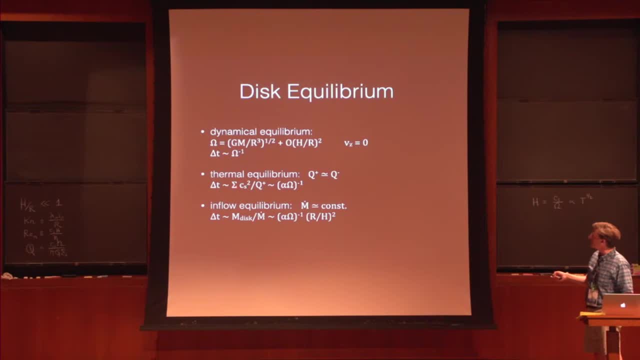 is again. this is the surface density of the disk, So grams per centimeter, Centimeters squared, multiplied by the square of the sound speed, so the temperature, And this is of order alpha, omega minus 1.. So alpha, this parameter which describes the intensity of turbulence in the disk, is believed. 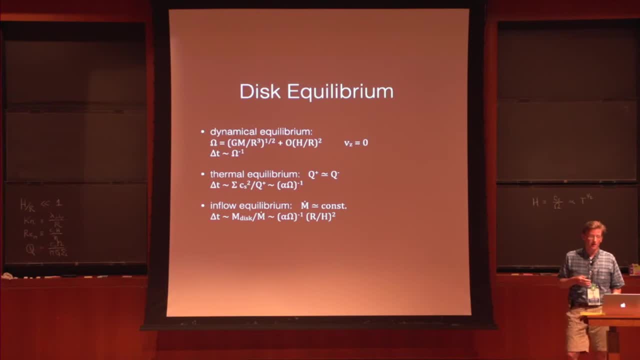 to be somewhere between a tenth and a hundredth in many systems, So this is substantially long. if that is the case, then this is substantially longer than the time scale. So that's the time scale on which the system reaches dynamical equilibrium. 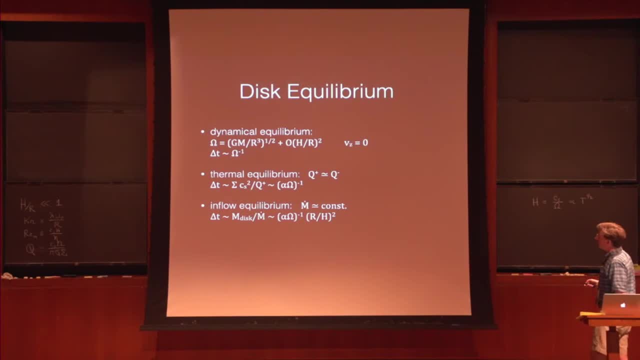 Okay, The final time scale is known as the viscous time scale, And that's the time scale on which inflow equilibrium is reached. So you can imagine feeding mass into a disk at the outer edge and then having it gradually make its way inward toward the central object, at some rate. 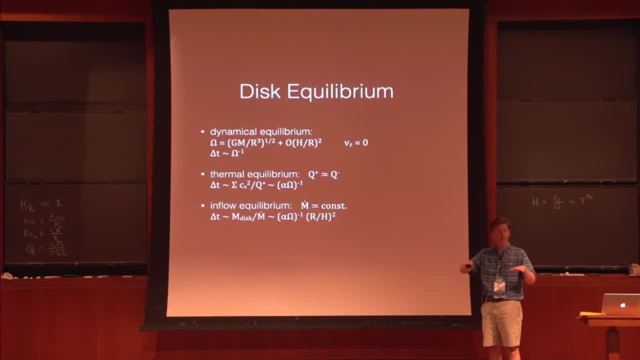 And as time goes on, Okay, It may set up an equilibrium where the inflow rate is constant at every radius. And that happens on this viscous time scale, which turns out to be longer than the thermal time scale, by of order r over h squared. 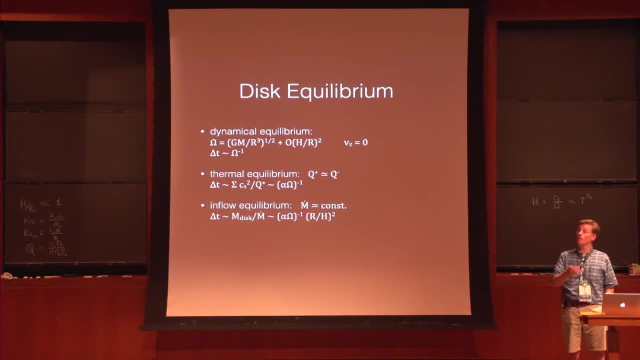 So, again to go back to the example of protoplanetary disks, this might be a factor of a hundred longer. Okay, So that describes disk equilibrium. So the next step is to go on and ask how disks evolve over time. So the analogy here is to stellar structure and stellar evolution. 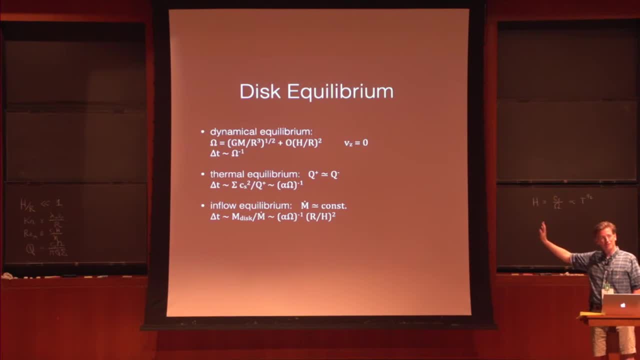 So this is the stellar structure or disk structure model, And then the next step is evolution. And because this is all about angular momentum, Okay, Okay, And angular momentum conservation and angular momentum evolution. the governing equation is derived from an equation that describes the angular momentum flux inside the disk. 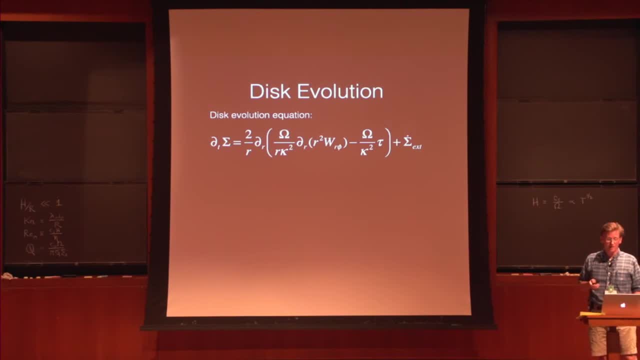 So let me just go through and explain what everything is in this equation. So we start with what's being evolved here. So on the left, Sigma, Omega, Omega. So this is the surface density, grams per centimeter squared in the disk. 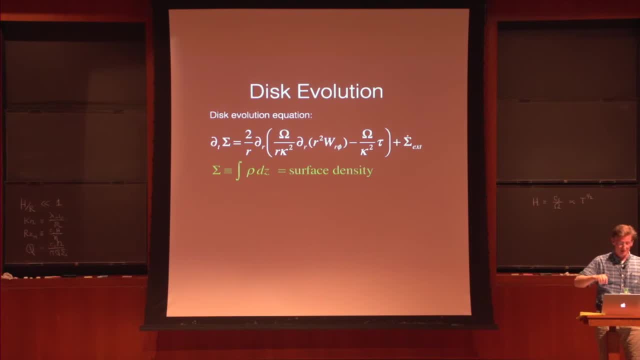 So the column vertically integrated, the density vertically integrated through the disk, Omega is the orbital frequency And kappa is the epiciclic frequency. And so, just to remind you, the epiciclic frequency is the natural radial frequency of oscillation in central potential. 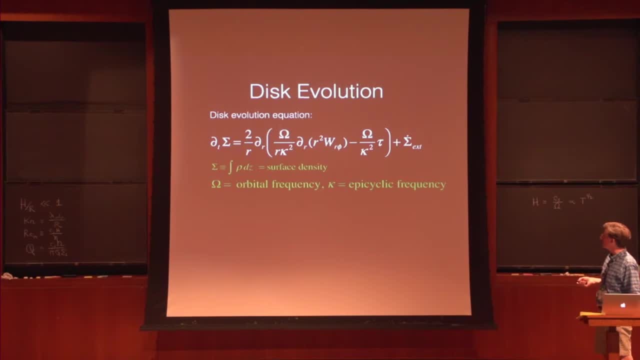 So this is the orbital frequency And the kappa is the epicyclic frequency. Okay, Okay, a cylindrically symmetric potential. So in a Keplerian disk, in a disk around where the potential is dominated by the central object, 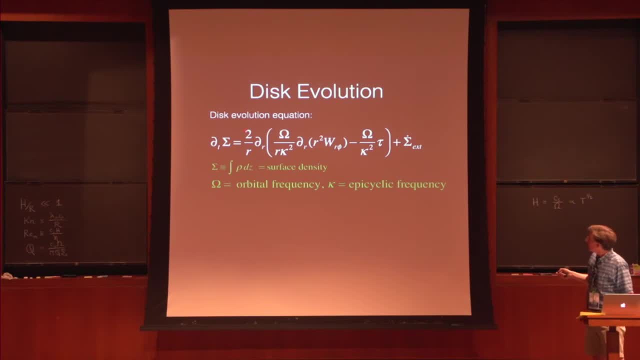 kappa is equal to omega. Okay, r is the cylindrical radius. here W r phi is a shear stress, So this is a quantity that tells you what the radial flux of azimuthal momentum is. So this is a component of the stress tensor. 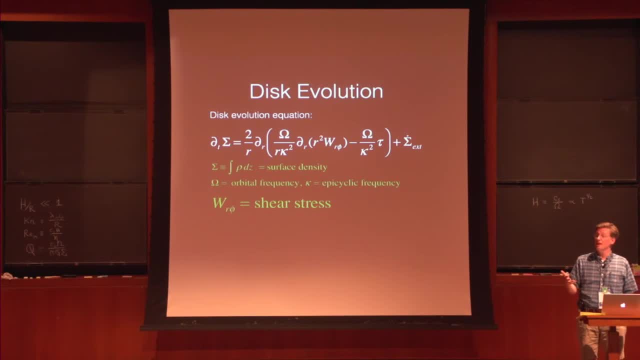 Radial flux of azimuthal momentum, which obviously is connected to the radial flux of angular momentum through a factor r. So that appears under a second derivative here. So this is integrated vertically through the disk. So one calculates this off-diagonal component of the stress tensor. 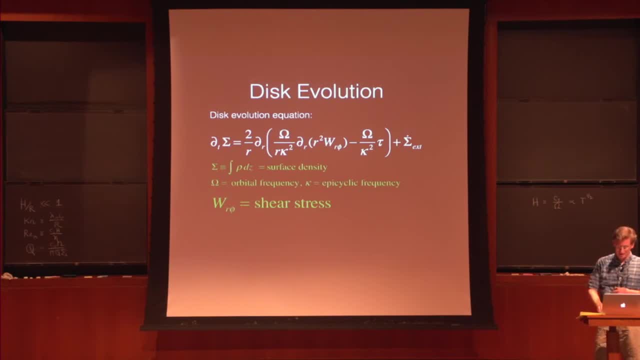 inside the disk and then integrates it vertically. Okay, next up is this parameter, tau here, which is connected to external torques. So external torques can be imposed on the disk. It can lose angular momentum Vertically by direct extraction in a magnetized wind. 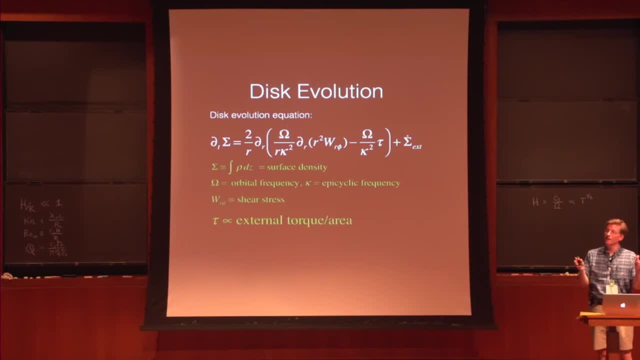 It can have torques applied locally by non-axisymmetric gravitational fields So that all can be captured in this external torque. And then finally, there is mass loss or gain, either through loss of mass in a wind from the surface of the disk or gain of mass through infall from outside. 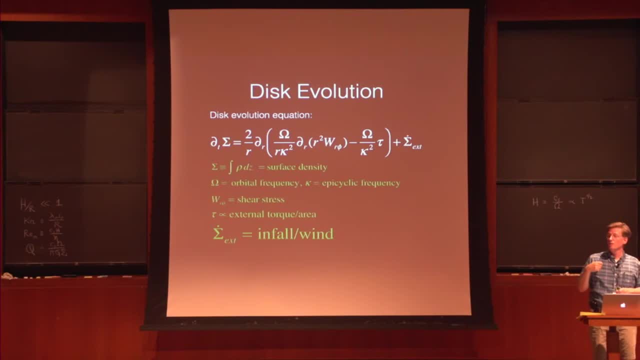 So infall onto the disk might happen in a protoplanetary disk system where there's a remnant envelope around the young star. Winds are observed in systems like SS Cygni in spectral lines. So if you look at this you can see that there's a lot. 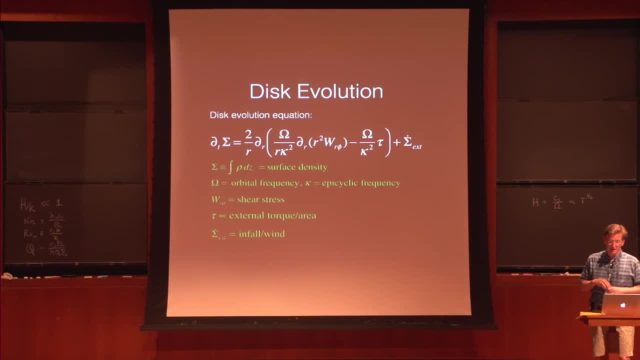 of mass loss from the disk. Okay, So this is the disk evolution equation. The full derivation of this is an exercise for the student. So if you want to work in disk theory, you should do this calculation, And it's actually not that difficult. 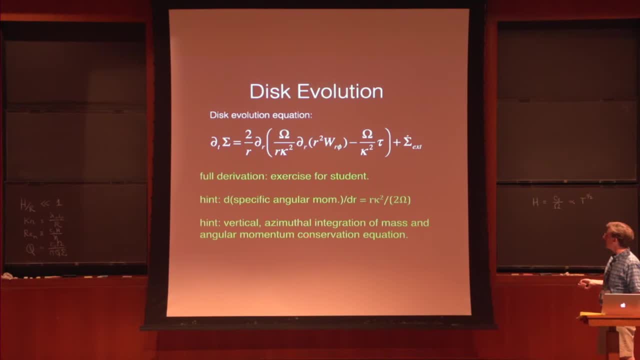 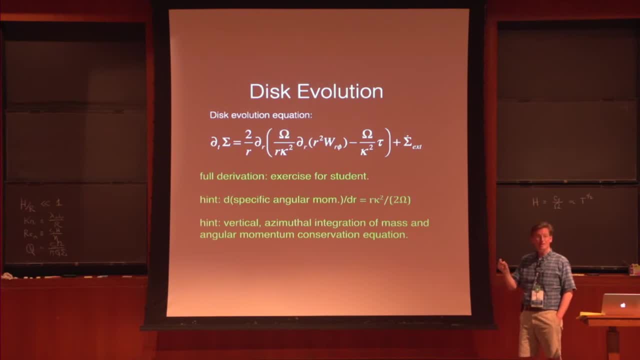 It is orbiting in circular Keplerian orbits. So the angular momentum per unit mass is fixed, And then you use conservation of mass as well, And then the only additional hint I would give here is that this factor kappa, squared r over omega. 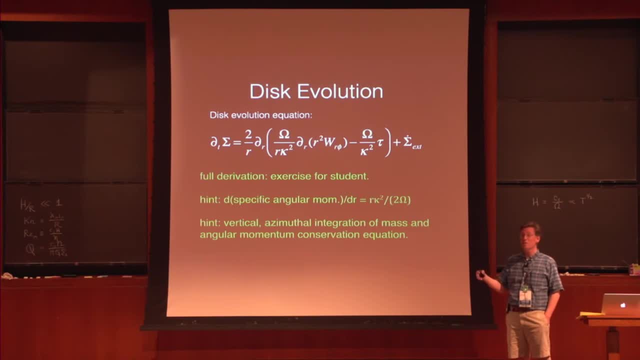 comes just from the radial derivative of the angular momentum per unit mass. Okay, So the big question, the big questions in disk theory are: what gives rise to this shear stress and what gives rise to this external torque? Now this turns out to be possibly a global problem. 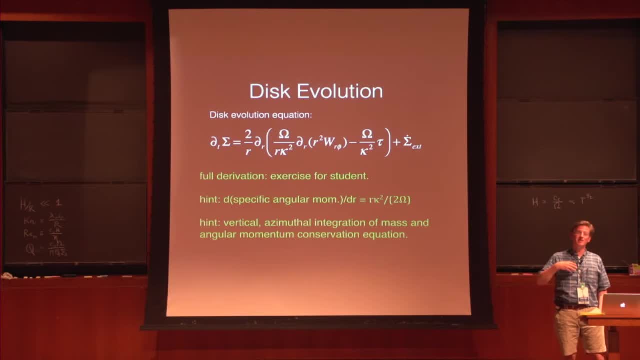 In other words, to understand, let's say, magnetic torques on the disk, you have to understand the global evolution of magnetic fields in and around the disk, And that turns out to be a very difficult problem that is just now becoming accessible. 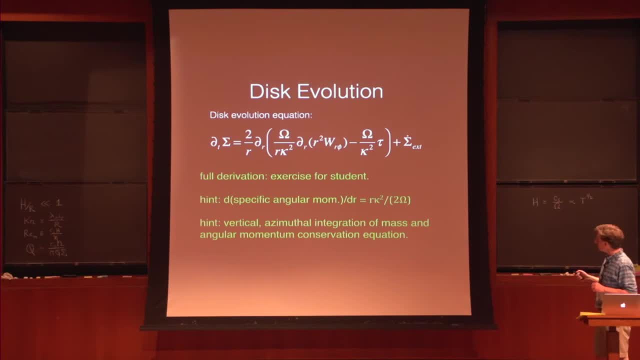 with the largest scale simulation. This may be a little bit easier, in the sense that it may be possible to study the development of turbulence in little patches of the disk. This may be a local problem, And from those local analyses one might be able to derive a model. 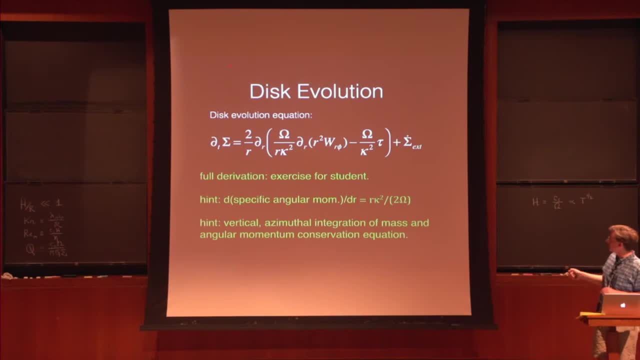 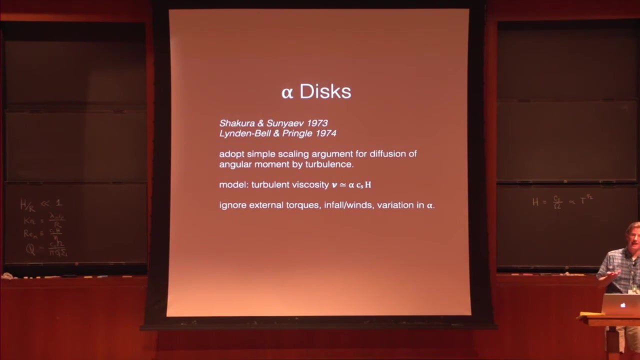 that allows integration of this piece of the disk evolution equation. Okay, So the standard model for disks is the alpha disk model And you really can't understand anything that's happened after alpha disks were introduced in the 1970s without understanding a little bit. 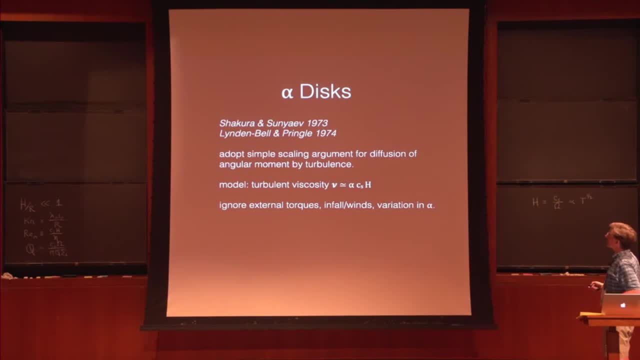 about what alpha disks are. So these guys were introduced in a paper by Shakur and Sunyaev in 1973 and in a paper by Lyndon Bell and Pringle in 1974. And the idea is to adopt a simple scaling argument. 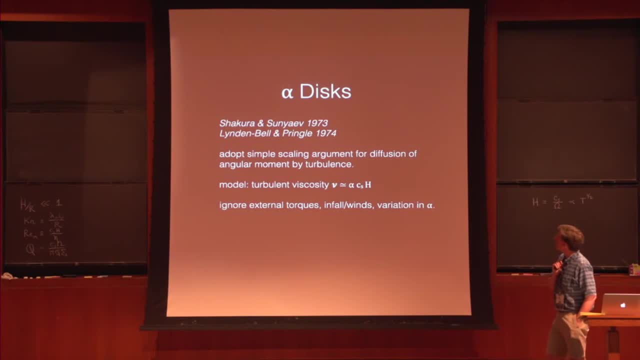 for that shear stress in the disk evolution equation. And one way of thinking about this scaling argument is to imagine that the turbulence can be modeled as the effects of turbulence in the disk can be modeled as a viscosity, But not a microscopic viscosity, but a viscosity with a very large coefficient. 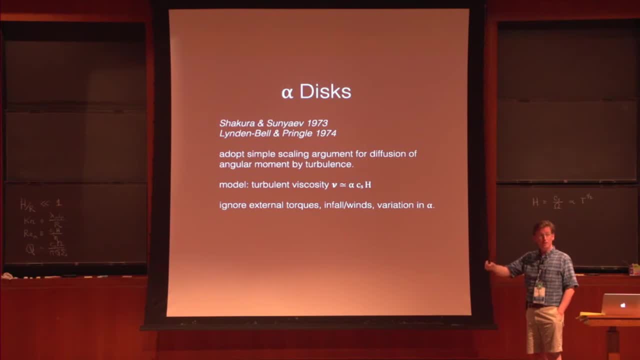 related to the eddy size of the turbulence and the scale of the eddies. So in this model you have a turbulent viscosity nu, which is just this alpha parameter again, which describes the intensity of turbulence multiplied by something with the characteristic dimensions of a viscosity. 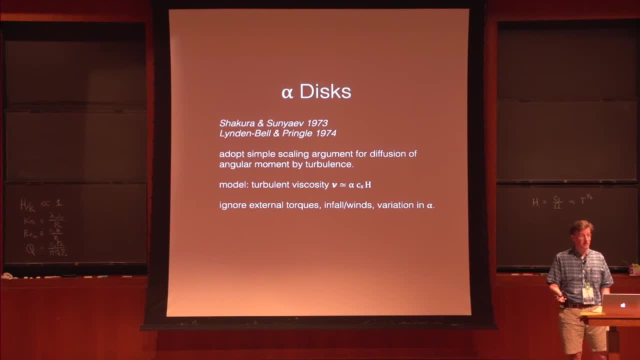 So viscosity has dimensions of a diffusion coefficient which is a length times a velocity, And the natural velocity scale is the sound speed in a thin disk and the natural length times a velocity in a scale is the scale height. So we introduce a turbulent viscosity. 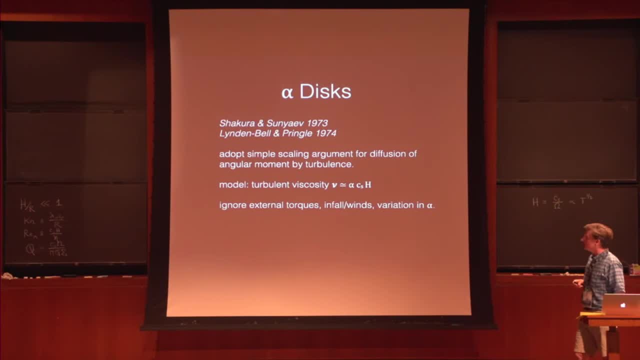 of order: alpha times, cs times h, And then in the classical alpha disk models one ignores the effects of external torques and one ignores infall, winds and possible variations in the alpha parameter. So it's the simplest possible disk evolution model. So we've thrown away most of the terms. 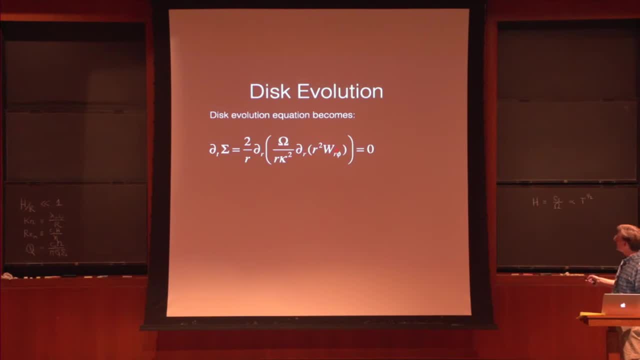 in that disk evolution equation and now we just have one left And you can see there's this shear stress in here which is going to be somehow related to the surface density And that appears under two derivatives, two radial derivatives, And then on the left, 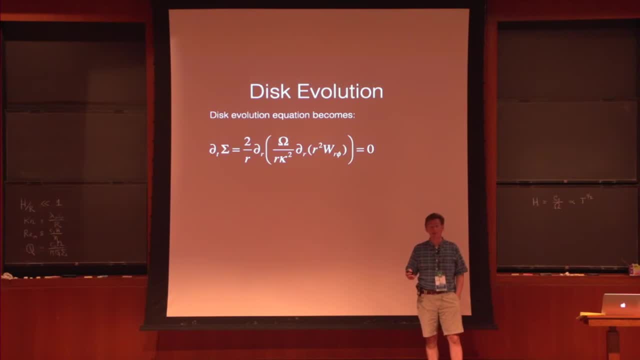 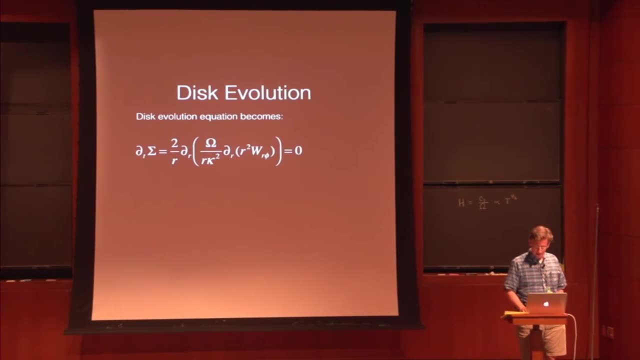 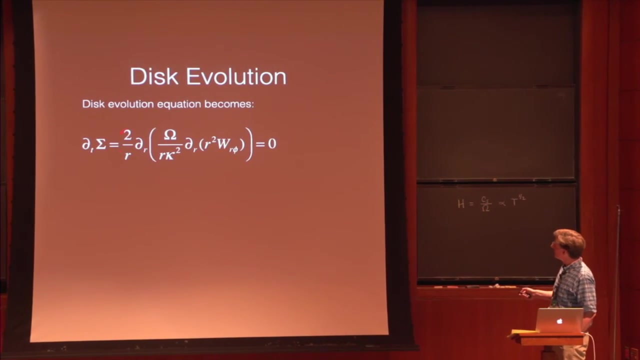 it's related to the time variation of the surface density, So this looks like a diffusion equation. Okay, So in the alpha disk model one assumes that that system- Sorry, I should have said this- One assumes that the disk is in a steady state. 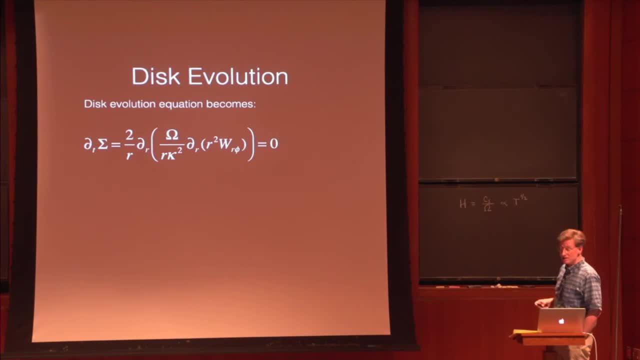 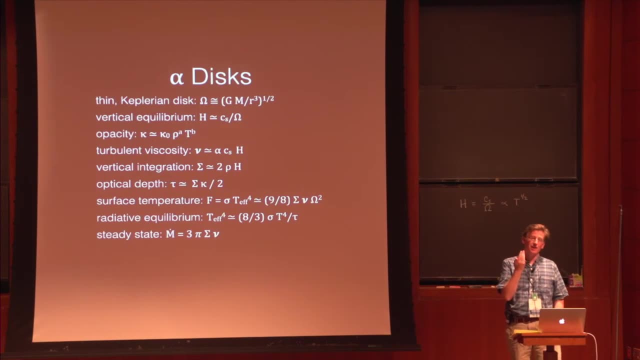 so that the surface density isn't changing and this thing can be set to zero. Okay, so here's a list of what goes into formulating the alpha disk model. So first of all, one assumes a thin Keplerian disk, so the parcels of gas are orbiting as rings. 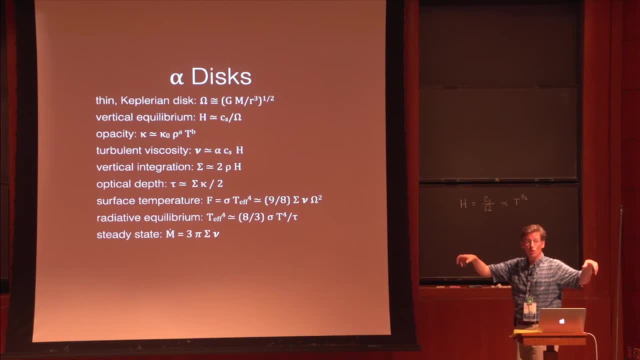 around the central object with orbital frequencies of order, the Keplerian orbital frequency. One also assumes that the disk is in vertical hydrostatic equilibrium and that leads to this relationship between the scale, height and the sound speed and the orbital frequency. So in the frame of the model, 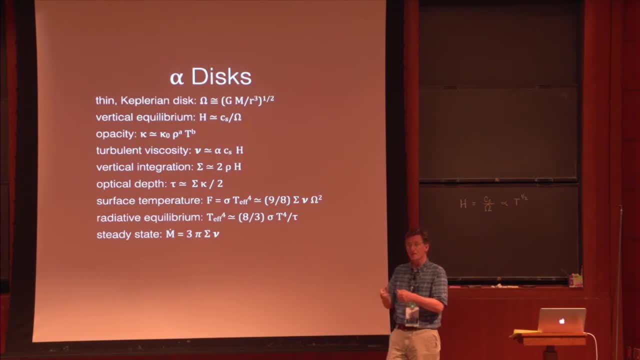 in the frame of the disk. if you go out into the disk and ride with the plasma as it orbits around the central object, you'll see that vertically the disk has a harmonic potential, And so that harmonic potential confines the plasma into the thin disk. 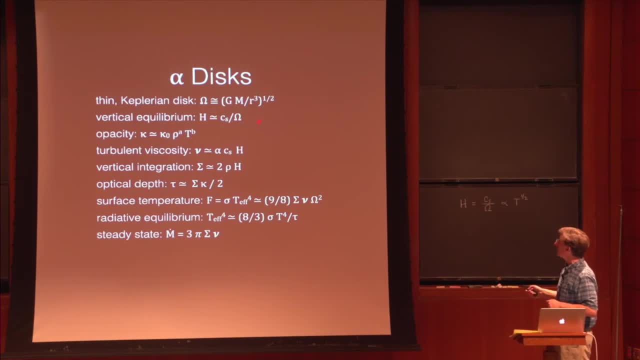 And by solving equation of hydrostatic equilibrium one finds this relationship Okay. The next step is to understand the thermal equilibrium of the disk, And to do that one has to balance the heating, which is related to dissipation of turbulence, against the cooling. 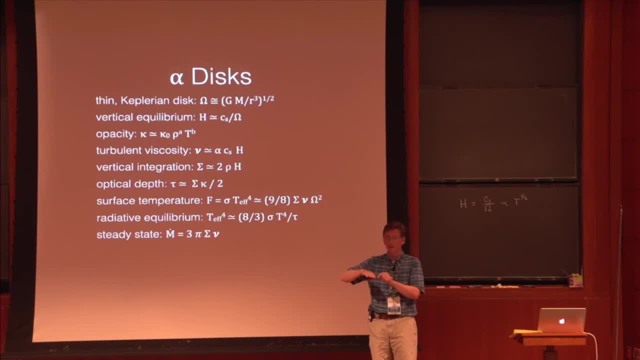 which, in the alpha disk model, is related to vertical diffusion of vertical radiative diffusion of energy. Okay, so in order to do that calculation, one needs an opacity, And the classic thing is to use an approximate opacity where the Roslin mean opacity is assumed to scale. 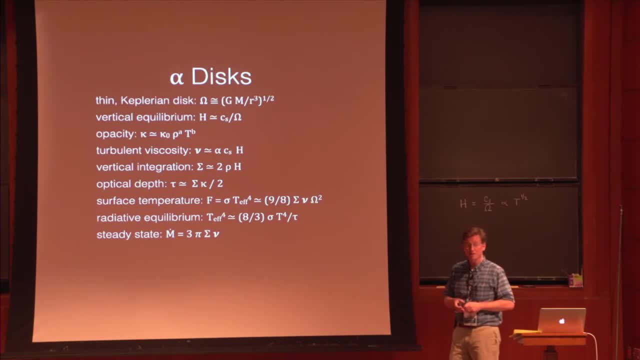 as some power of the density and some power of the temperature. Okay, Then we have the turbulent viscosity which controls the heating rate. in the disk, We have a prescription for vertical integration of the density, So the surface density is approximately related to the volume density. 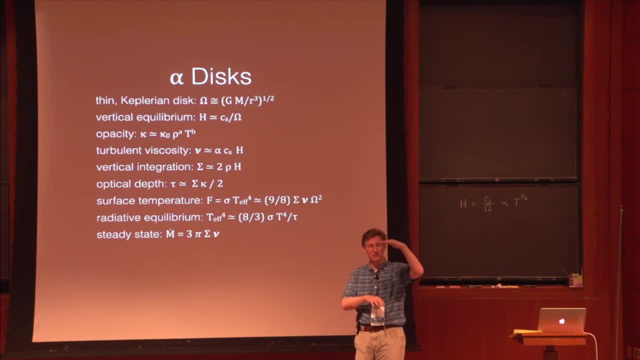 multiplied by two times the scale height. So this is a crude integral. And then an estimate for the optical depth from the surface of the disk to the center of the disk. So surface density times kappa, the opacity is the optical depth to the center of the disk from the surface. 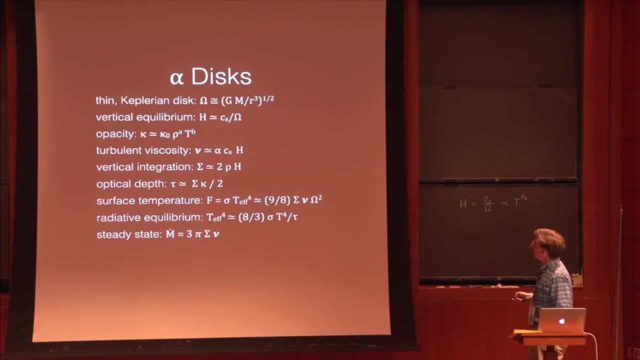 Okay, So to finish the radiative equilibrium, we need the surface temperature. So the effective temperature is assumed to be equal to the total energy dissipated by turbulence inside the disk, And that's related to the viscosity and the shear rate. So this is one of these omegas. 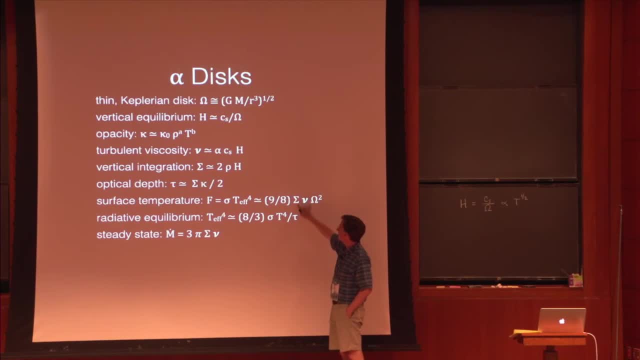 gives you the viscous stress here. sigma nu, omega is the stress multiplied by the rate of strain, which is omega gives you the total rate of dissipation per unit area. So this gives you an estimate for the surface temperature. 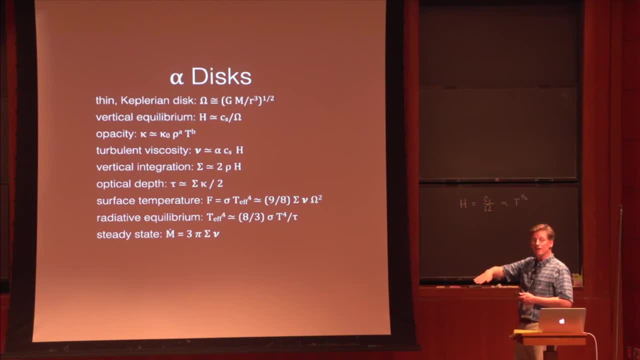 And then radiative equilibrium tells you how the energy diffuses out from close to the midplane of the disk, And that relates the effective temperature at the surface of the disk to the central temperature at the midplane of the disk through a factor of the optical depths. 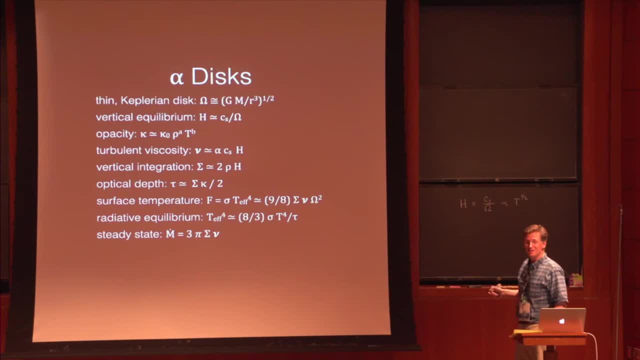 Okay, and there's a wrong factor of sigma in here, So this is not dimensionally correct, But you can mentally cross that out. So T effect to the fourth is approximately T central to the fourth divided by tau. So if the optical depth is large, 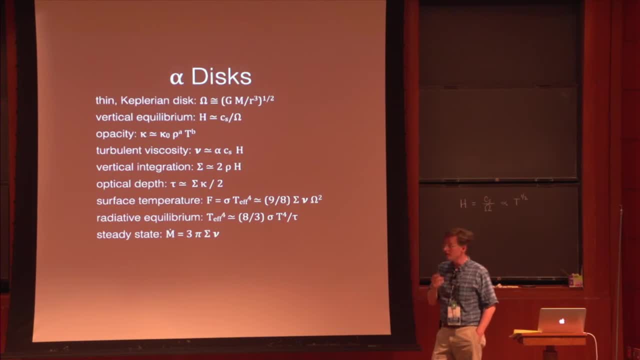 the central temperature of the disk is large compared to the surface temperature. Okay, and finally, in a steady state, one finds that the accretion rate is related to the shear stress by this equation which arises from the disk evolution equation. So this is a consequence of that. 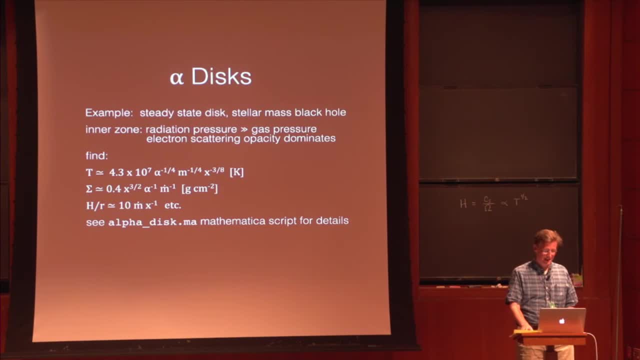 Okay, so that's a lot of estimates that I haven't justified very carefully, But let me show you the outcome. So, as an example, consider a steady state disk around a stellar mass black hole, And in these alpha disk models one divides the disk into zones. 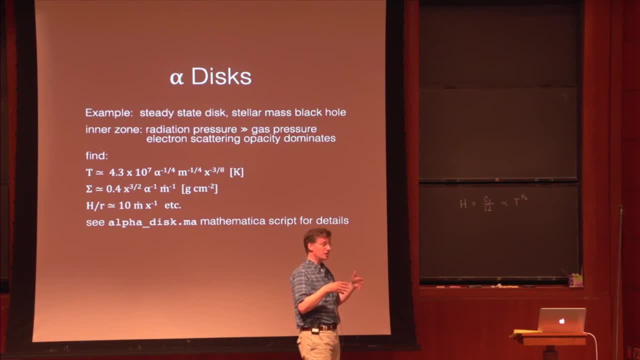 radial zones according to the dominant opacity close to the midplane of the disk, And for a disk which is accreting close to the Eddington rate onto a stellar mass black hole, the innermost zone has radiation pressure much larger than gas pressure. 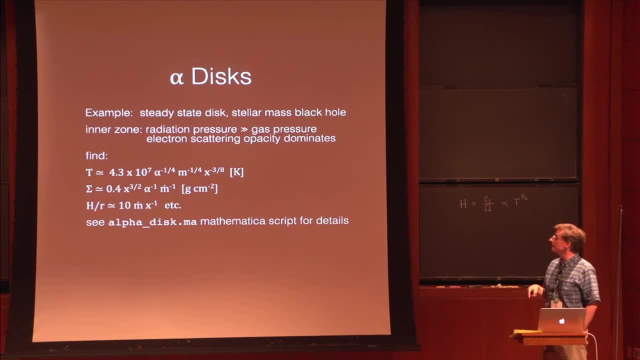 And electron scattering dominates the opacity. Okay, so one finds that the temperature, the central temperature of the disk is 40 million Kelvin. And then there's a scaling here with alpha, with the mass of the central object in units of a solar mass. 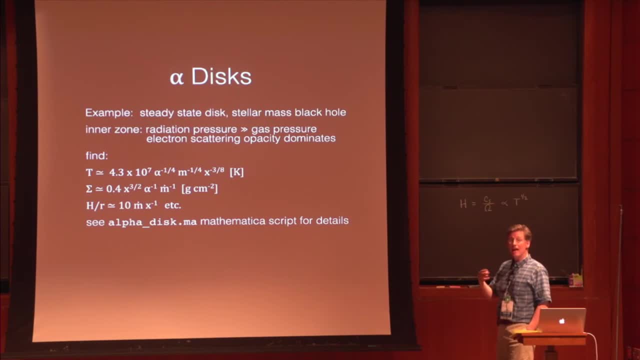 and with the radius x cast in units of gm over c squared. Okay, So this gives the run of central temperature in the inner region of the disk. This gives the run of surface density in the disk, So 0.4 grams per centimeter squared. 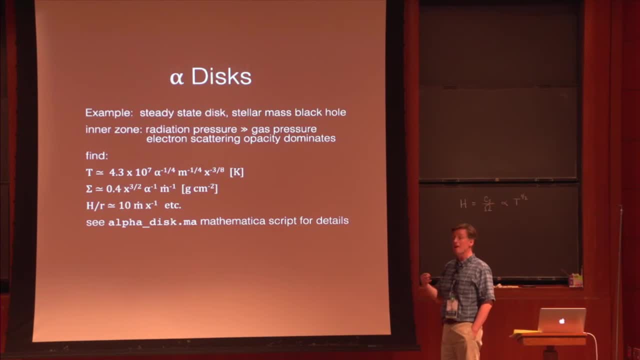 with a scaling in terms of alpha and a scaling in terms of the mass accretion rate in units of the Eddington rate. Okay. And finally, a scaling of h over r with radius. Okay, so what I've done for you. 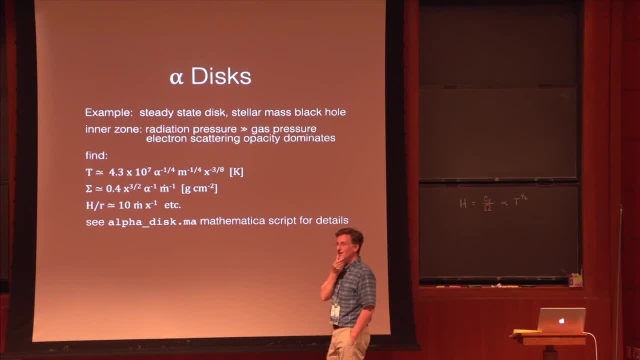 in case you didn't follow all the details of what I just said, is provide you with a Mathematica script that Peter is going to make available, I think on the web. It's already there And you can run this Mathematica script. 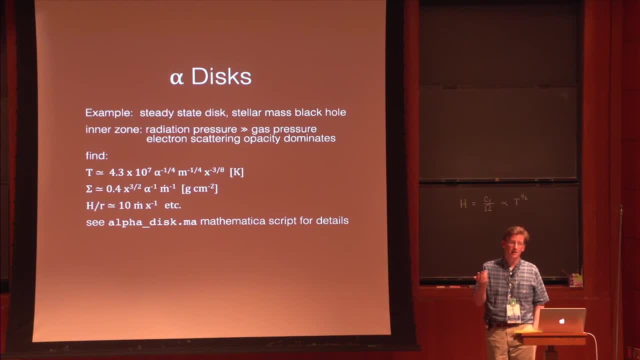 and obtain a general alpha disk solution for any system with any mass, as long as you provide a suitable scaling for the mass of the central object and a suitable scaling for the accretion rate. Okay, So in that you will see explicitly what opacities one might use. 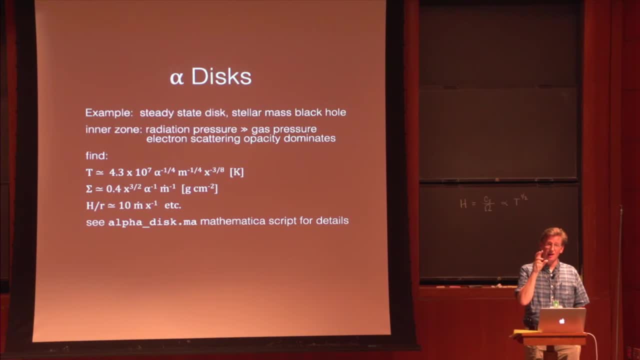 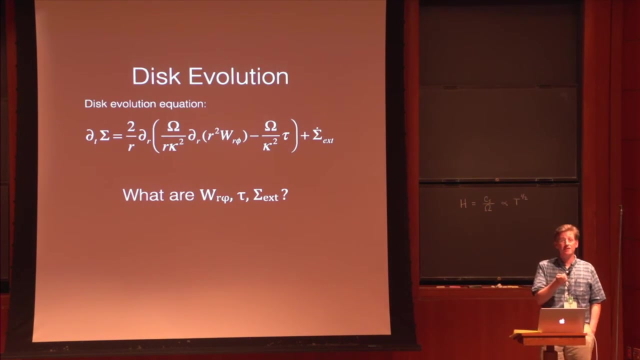 for these disk estimates, and you'll see explicitly the estimates that I've quickly gone through here for equilibrium of the disk, thermal equilibrium and hydrostatic equilibrium. Okay, So back to the disk evolution equation. So, as I said, the big questions here are: 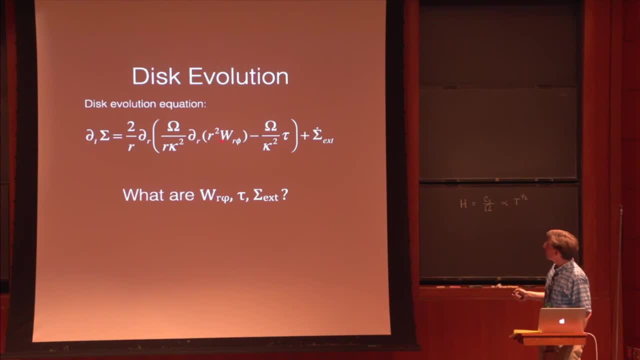 the shear stress, what provides the shear stress in disk, what provides the external torque and what might be the inflow and outflow rates? So part of this is answered through studies, local studies of turbulence in disks. So let me go on. 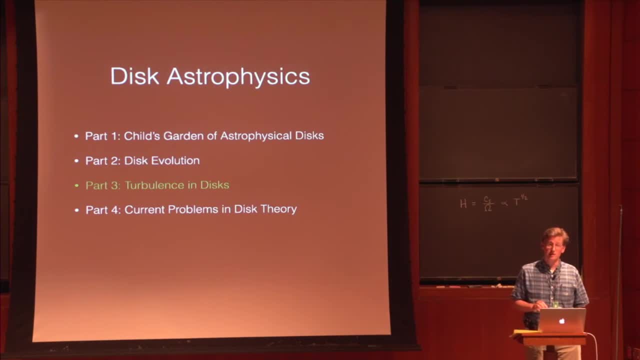 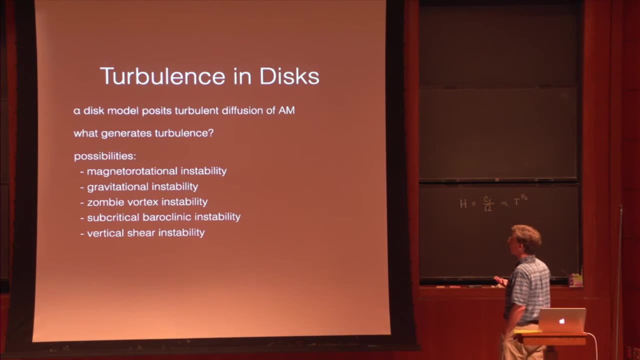 and talk about turbulence in accretion disks. So again, this is important in relation to the classic alpha models, because the alpha disk model posits this: the existence of this turbulent diffusion of angular momentum. and the question is, what generates turbulence? 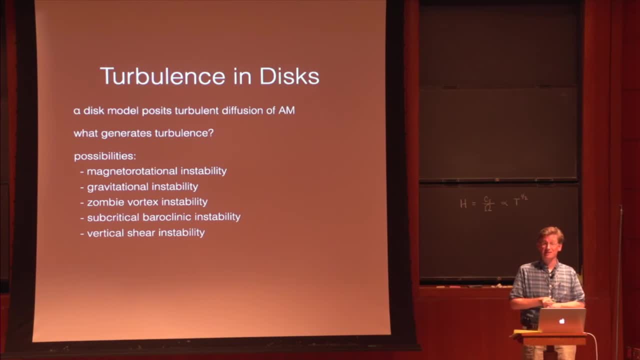 And there are many live possibilities in 2016.. So one possibility is the magnetorotational instability, which I'm going to discuss in some detail next. Another possibility is gravitational instability, So in disks around supermassive black holes in galactic nuclei. 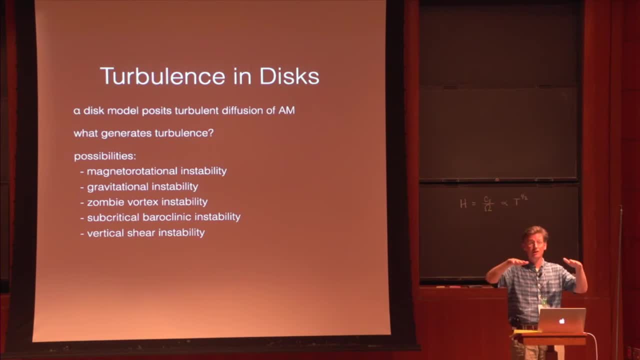 the Tumor Aq parameter which I wrote down over there, drops close to one inevitably as one moves out in the disk for any accretion rate. So gravitational instability is relevant to the outer parts of active galactic nuclei accretion disks. 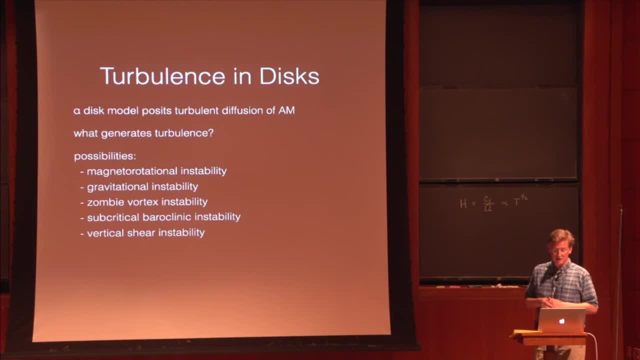 It's also relevant to massive T-Tauri disks or protoplanetary disks. Okay, There are a couple of other possibilities, or three other possibilities which are related to fluid dynamical instabilities which are known to exist in in accretion disks. 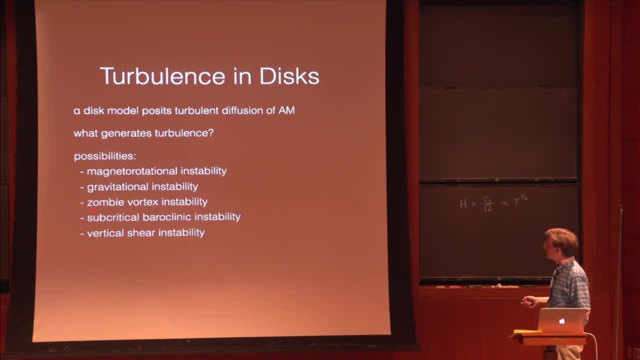 So one is the so-called zombie vortex- instability, And this is work that's come out of Phil Marcus's group at Berkeley, Joe Barranco, Phil Marcus, I think it's. it's still a little bit controversial And there are recent papers. 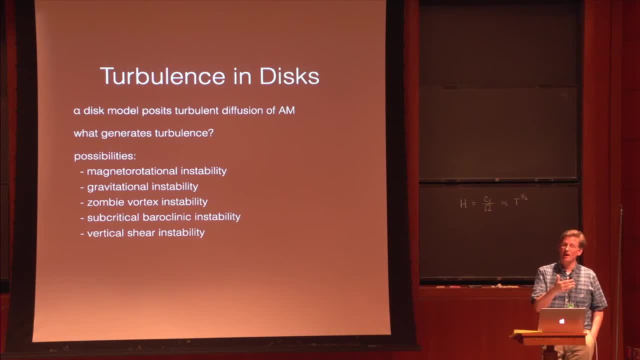 which critique the the robustness of the zombie vortex instability by Geoffroy Le Sueur and and others. Okay, So this is an instability which generates vortices in unmagnetized disks And then it's possible for those vortices 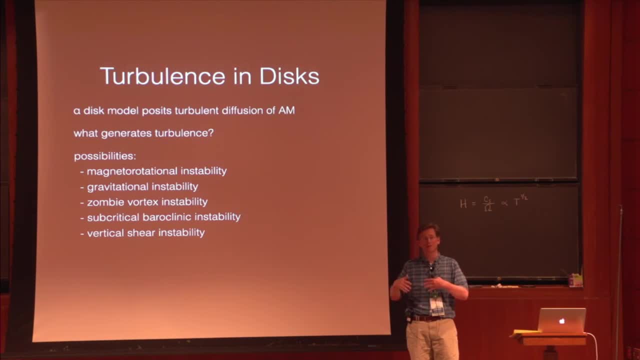 to shed spiral sound waves that carry angular momentum, That exchange angular momentum between radially separated parts of the disk And that might lead to a non-negligible alpha. The vertical shear instability here is connected to the possibility that the orbital frequency varies vertically. 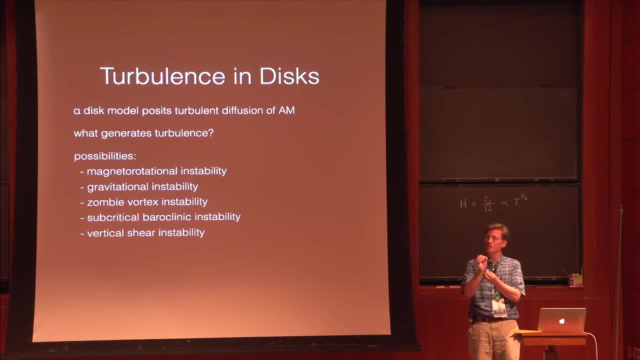 inside the accretion disk And in that situation there's a an instability of incompressible waves that shear like this, with a period comparable to or larger than the orbital frequency, and that that grow and saturate as as sound waves. 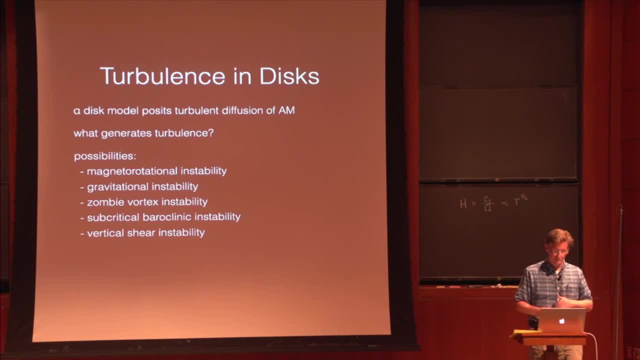 which again can transport angular momentum. And then the subcritical baroclinic instability is an instability that arises out of work by Hubert Klar many years ago and is related somewhat loosely to the baroclinic instability that drives weather on the surface of the Earth. 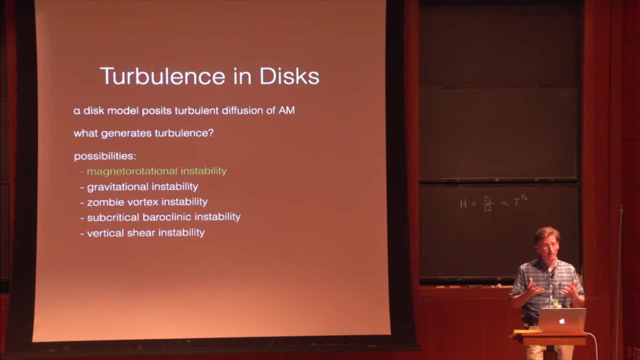 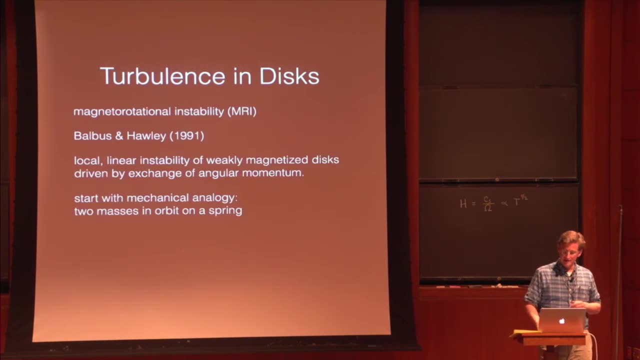 Okay, So I can't cover all these topics, So I'm going to focus on the magnetorotational instability. And the magnetorotational instability was discovered in the context of Couette flow- magnetized Couette flow- in the 1950s. 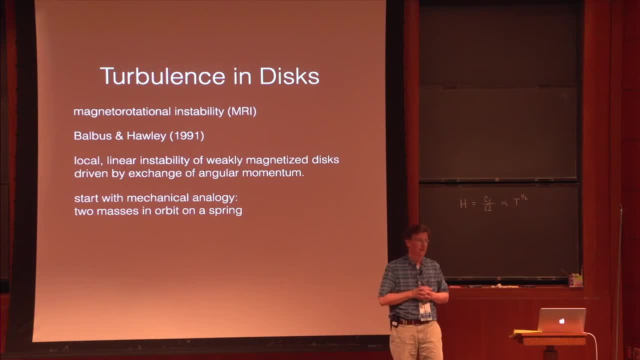 by a Russian scientist named Velikov. So Couette flow is a laboratory, laboratory flow between rotating cylinders. so there's a fluid, there's an inner cylinder, there's an outer cylinder, they rotate at different rates and there's a magnetic field. 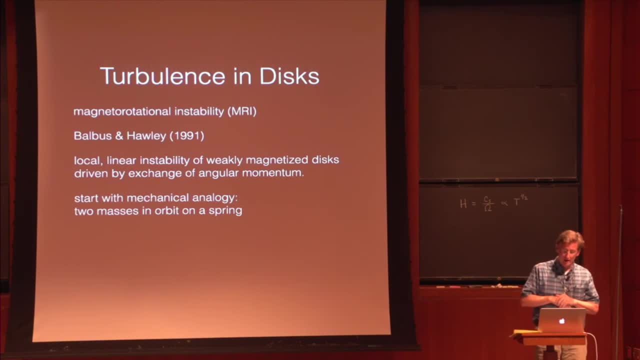 embedded in the Couette flow. So this was known to well, to Velikov, to Chandrasekhar in. so this instability is described in Chandrasekhar's book on hydromagnetic and hydrodynamic stability, But it was not realized. 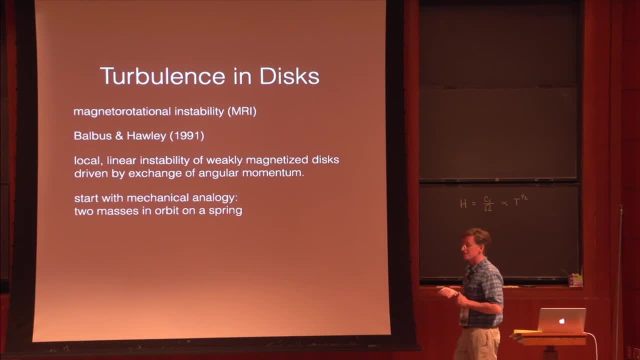 that this instability might occur in accretion disks until the early 1990s when Balbus and Hawley studied this and discovered that there is a local instability of accretion disks. So local here means that the presence of the instability doesn't depend. 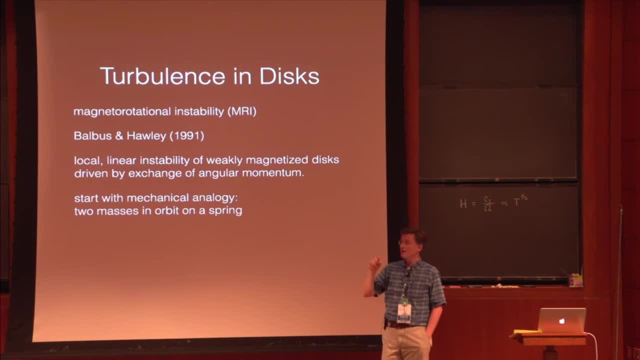 on boundary conditions in the disk. It occurs on a small scale inside the disk. that can be treated and it can be treated in the WKB approximation. It's an instability of weakly magnetized disks, So one doesn't need a strong magnetic field. 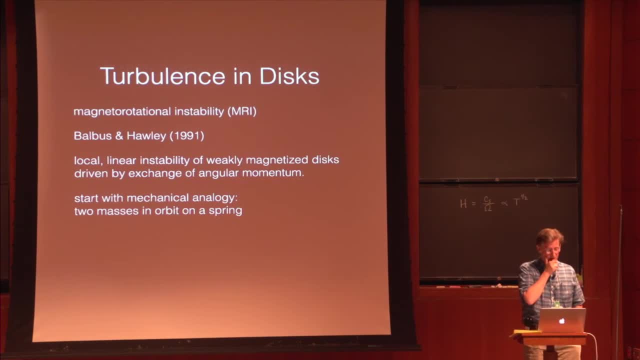 present for the instability to take off, And it turns out that the instability itself is driven by exchange of angular momentum between radially separated fluid elements. So it's ideal for driving turbulence in disks that can lead to angular momentum evolution of the disk. Okay, 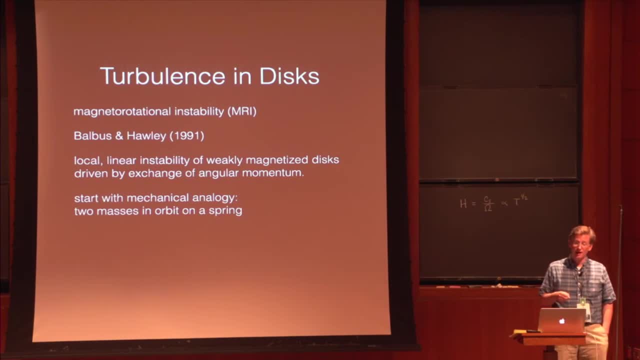 So I'm going to start with a simple and actually finish with a simple mechanical analogy for the magnetorotational instability which involves two masses on a spring. So let me, Can people who are sitting over here see this board? Yeah, Okay. 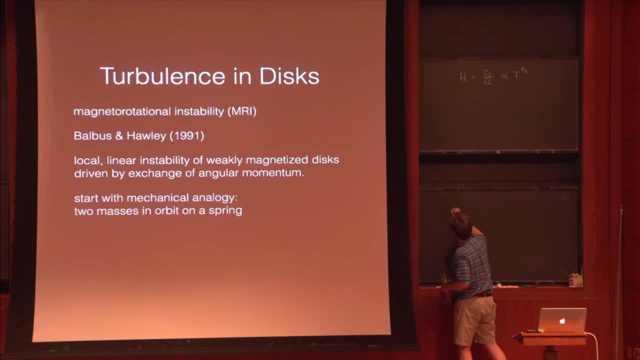 Okay, So the system we imagine is two masses connected by a spring in order to orbit around a central body. And for simplicity, I'll just consider the case where the potential is dominated by the central body, And so the orbital frequency is given by the Kepler. 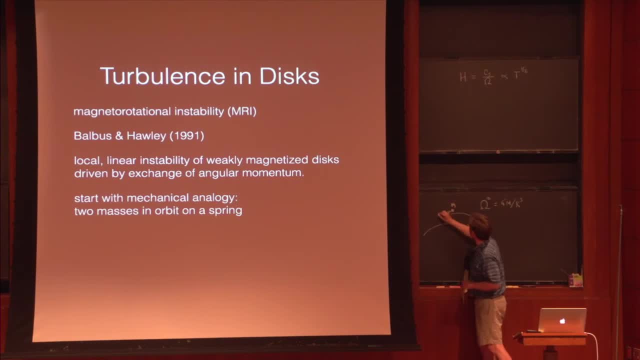 orbital frequency. Okay, So we have two masses and we have a spring that connects them, And then there's a characteristic frequency associated with the mass spring system, which I'll call gamma. Okay, So this simple model, which was first described in a paper, 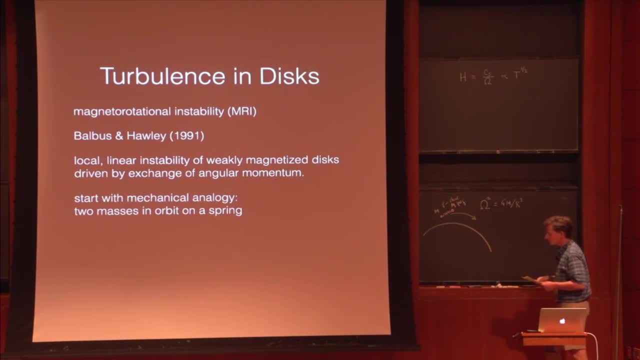 by Balbus and Holley captures essentially all the important features of this magnetohydrodynamic instability, without an extended calculation. Okay, So this is a very simple model. It's a very simple model. It's a very simple model. It's a very simple. 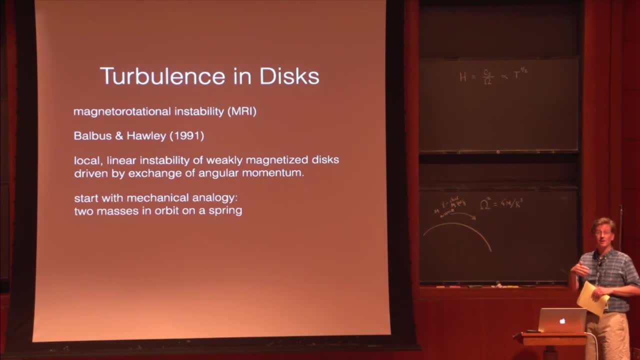 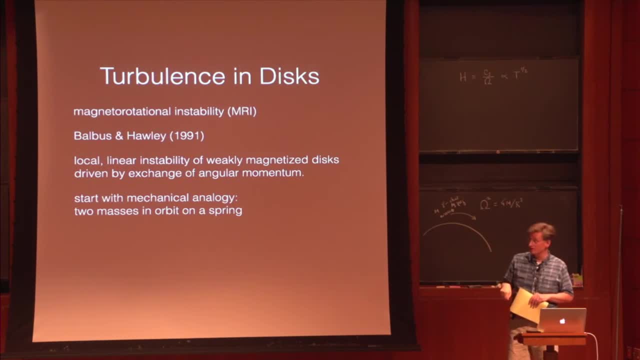 And the spring can be thought of as a magnetic field which connects the fluid elements, Uh, and then the bending of the field lines, uh, produces this restoring force which is modeled by this characteristic, characteristic frequency. I have to start by setting up a co-orbiting frame. 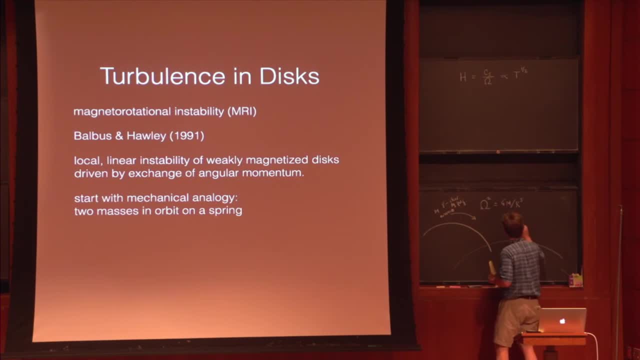 Okay, so let me draw an even bigger version of this here. So I'm going to set up Cartesian coordinates which are co-orbiting with these two masses in a circular orbit around the central object. So I'm going to orient the x direction. 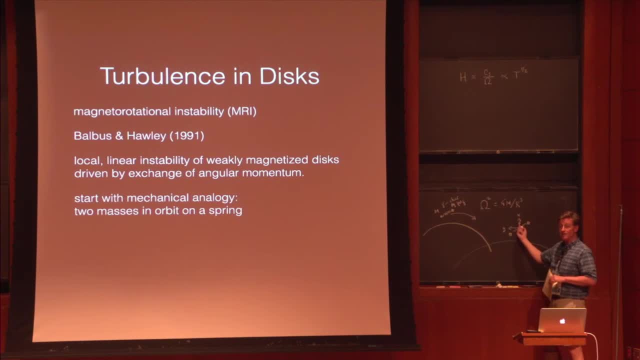 along the radius vector and I'm going to orient the y-axis along the direction of orbital or against the direction of orbital motion. So I can then write down the equations of motion in this local coordinate frame, and these equations, the equations of motion, are known as the Hill equations. 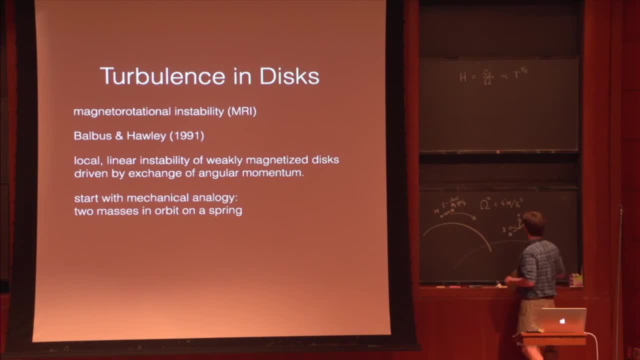 or the local model equations. Okay, so let me do that next. Okay, so the separation of one of the masses from the center of this coordinate system is x. So I'm going to write down the equations of motion in radius and x double dot is equal to minus 2 omega y dot. 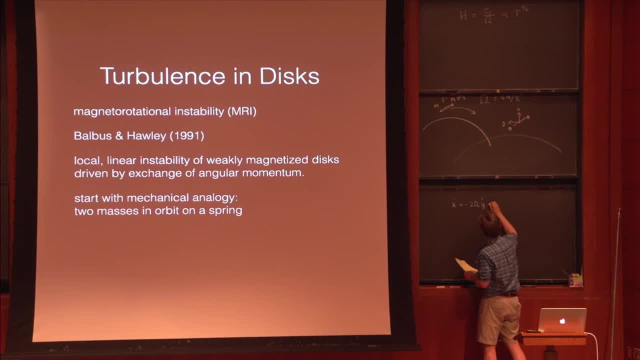 plus 3, omega squared x, minus gamma squared x. Okay, so the fundamental assumption I've made in writing down this first component of the equations of motion is that the separation of these masses is small compared to the local radius, And you can see that this might arise. 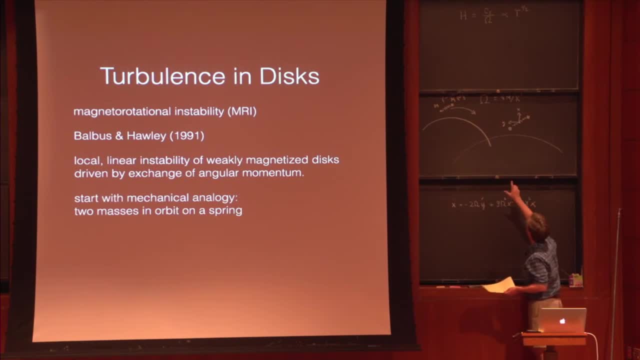 from the Coriolis force in this rotating frame where x is oriented along the radius vector and continues to be oriented along the radius vector as a pair of masses orbits around the central object. Okay, So this is Coriolis. This is the tidal expansion of the effective potential. 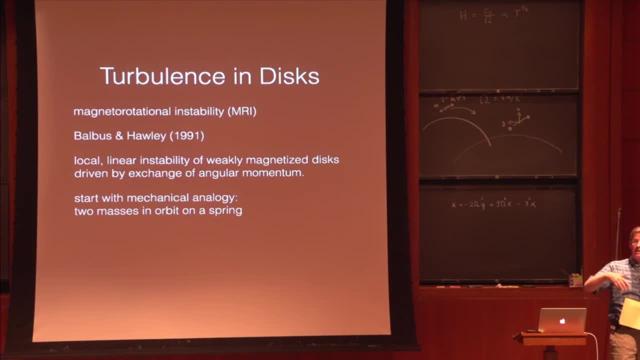 in the rotating frame. Okay, so there's 1 half omega squared. r squared describes the centrifugal component of the potential in the rotating frame. And then there's minus gm over r, which describes the gravitational potential, And combined this is the third component of the Coriolis force. 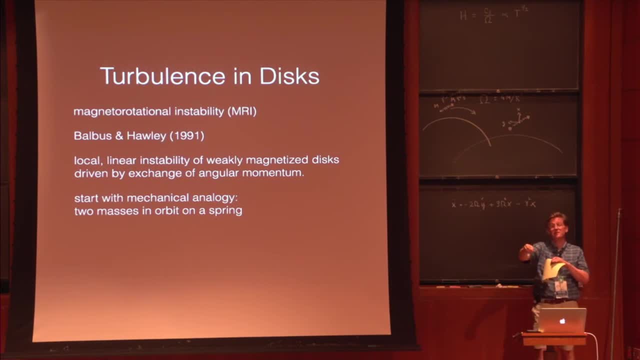 And then expanded in a Taylor series expansion, one finds this term. So this tends to produce separation. in the radial direction, It corresponds to tidal stress. Okay, the second component of the equation of motion in the toroidal direction, in the direction of motion. 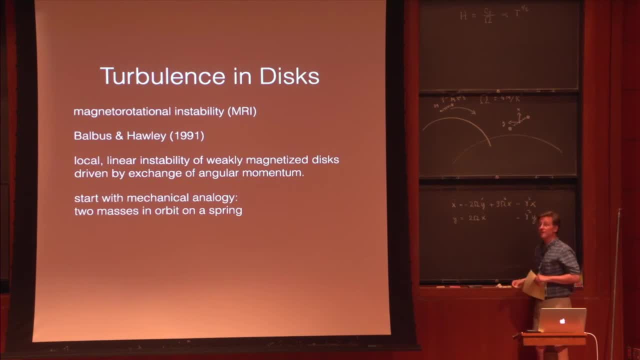 is the other piece of the Coriolis force, Again the spring term. So the spring term wants to restore the masses back to their original position. Okay, So again Coriolis, tidal expansion and spring, which represents the effect of magnetic fields. 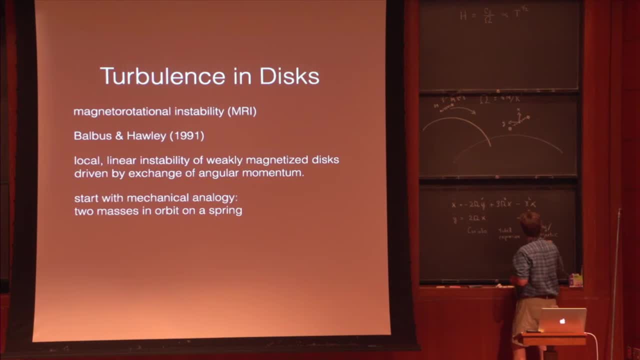 So that's the first component. Okay, So as a first go at this, we can ask what happens if we turn off the spring and say what are the modes of this mechanical system? So we set gamma to zero and then assume that x and y 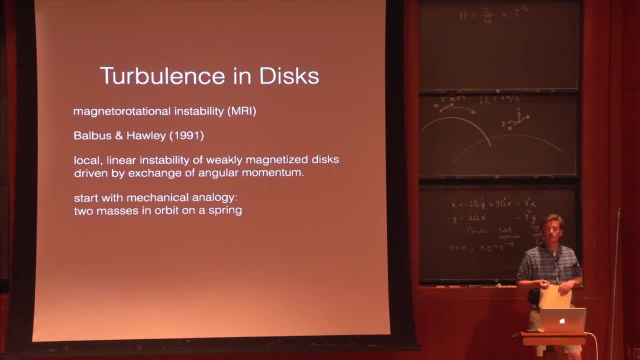 minus i omega t. This is a linear system, So we'll find a relationship between this frequency and the orbital frequency at the end of the day. So let me pull this up. Okay, so this equation becomes: minus omega squared x equals minus 2 omega times, minus i omega y. 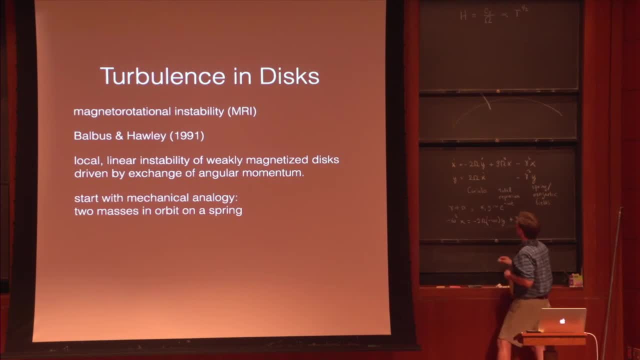 plus 3 omega squared x And the second equation becomes: minus omega squared y equals 2 omega times minus i omega x. Okay, So, So I can solve this equation for x, and I can solve this equation and then insert that into this equation. 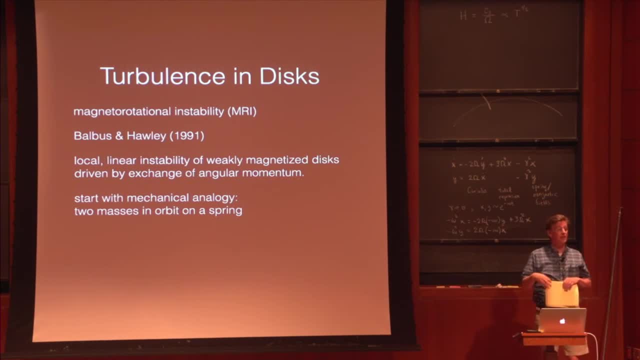 I obtain a linear equation in x, so the x's cancel out and I find a dispersion relation that relates the frequency to the orbital frequency And that gives you: omega squared is The non-trivial mode, is: Omega squared is equal to the orbital frequency. 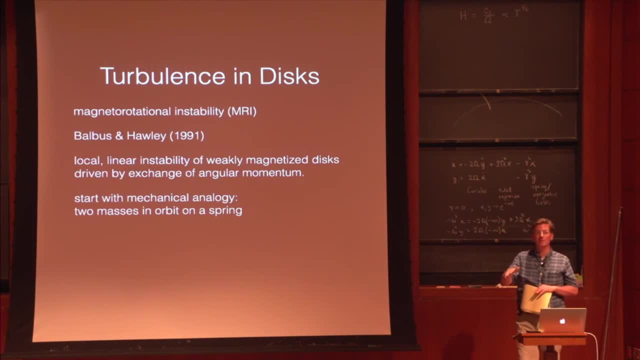 Okay, so this is a very boring result. It tells you that if you perturb the system, it oscillates at the natural frequency in the orbital plane. Okay, so the next step is to turn back on the magnetic fields And you can see exactly what is gonna happen mathematically. 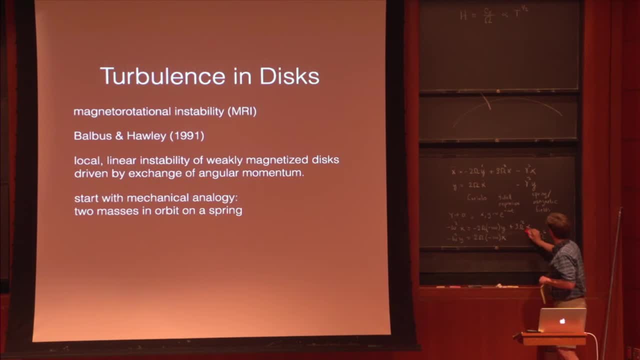 So we'll add on an additional term here: minus gamma squared x, minus gamma squared y, And again we can perform the same simple algebra and solve for the dispersion relation, And that is a good, That's a good answer, Okay. 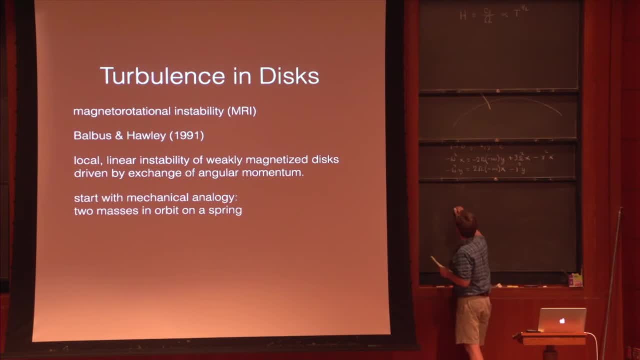 So That's a good, That's a good exercise for the student. The result is the following: Omega fourth minus omega squared. Okay, So this tells you. It turns out That there's an instability, And you can see this by considering the limit. 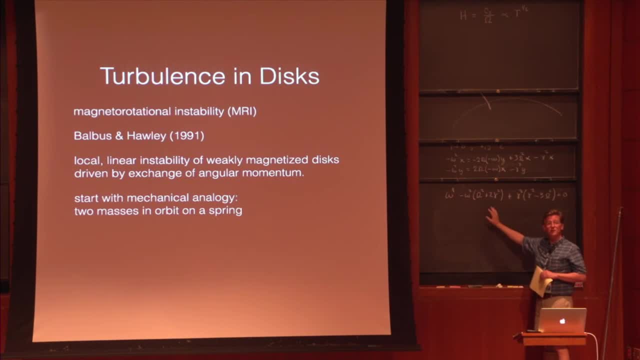 that omega is small. So looking at the marginal stability limit, And then you can see that there is a marginally stable situation when gamma is of order omega Okay. so this term vanishes when gamma squared is three omega squared. So that means there's a zero frequency solution at that point. 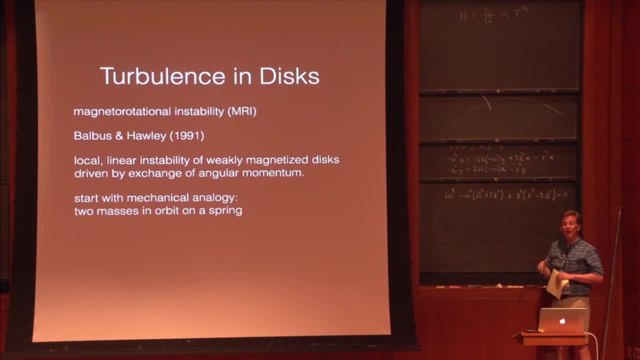 And that there's a transition from stability to instability. Okay, So let me just plot this up. So the single parameter here is the orbital frequency- Sorry, the spring constant squared divided by omega squared, And There's one, two, four. 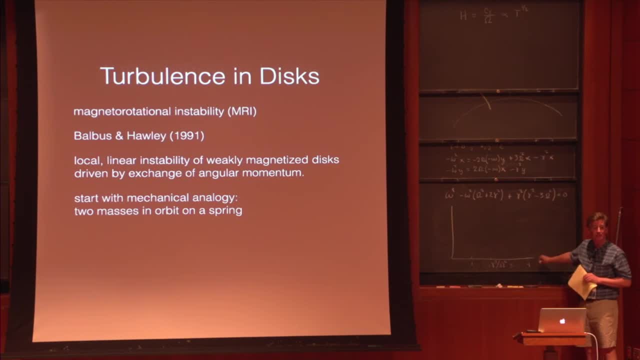 Can you see this in the back, Or am I writing too small? I see some yeses, All right. And then on this axis I can write omega squared over the orbital frequency squared. Okay, And There are two sets of modes here relating the. 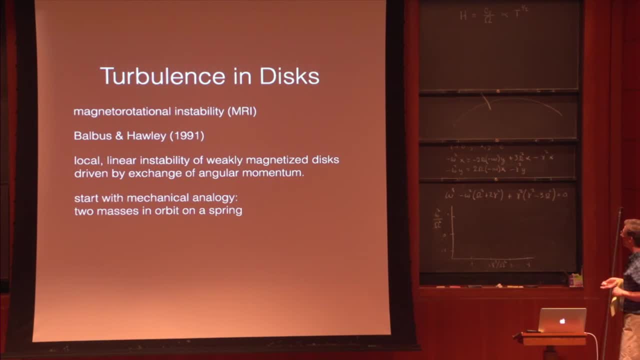 Produced by the two roots of the quadratic equation in omega squared, And one is the spring motion, which is what you would get if you just turned off the orbit. So the spring wants to oscillate at the natural frequency gamma. And then there's a second set of modes. 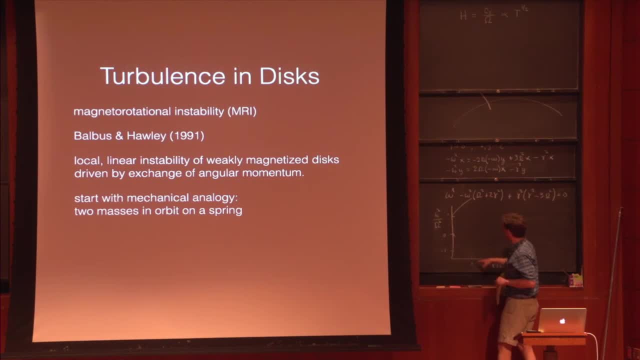 which have zero frequency, when gamma is small And then grow like this. And let's see, I'm Need to redraw this. Okay, So omega squared is negative in this region when gamma squared over omega squared is less than three, as was indicated by my earlier argument. 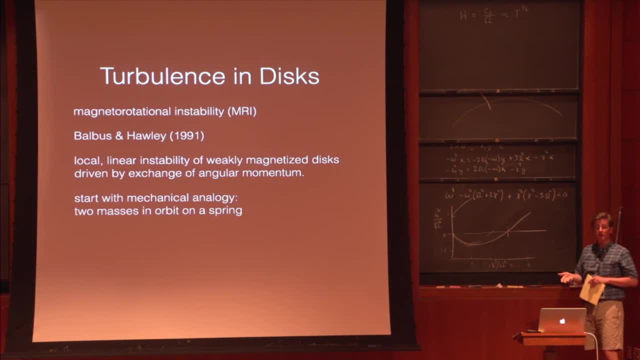 And if omega squared is less than zero, then we know that there's an instability. So there's an exponentially growing mode- An imaginary. There's a growing and a damped pair of modes, And the fastest growing mode can be had from just analyzing the roots of this equation. 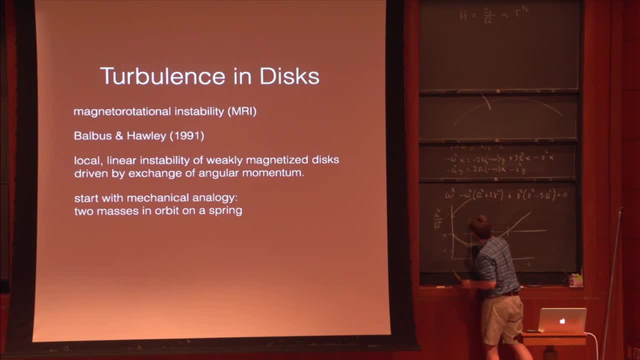 And one finds that this occurs at gamma squared over omega squared Is 15 sixteenths And at that point the minimum in omega squared, which corresponds to the fastest growing mode of the instability, is nine, Nine sixteenths omega squared. 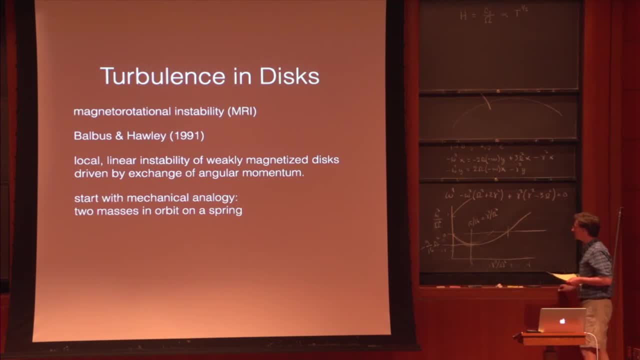 Or minus nine, sixteenths omega squared, Okay. And then, as the spring constant grows stronger, this mode eventually becomes stable. And then, when the spring is very, very strong, it doesn't feel the orbital dynamics at all, It doesn't care about the orbital dynamics. 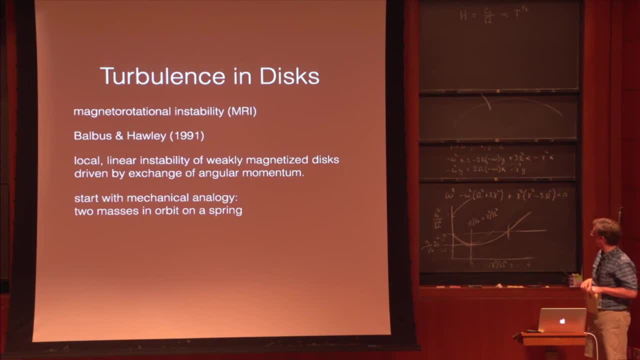 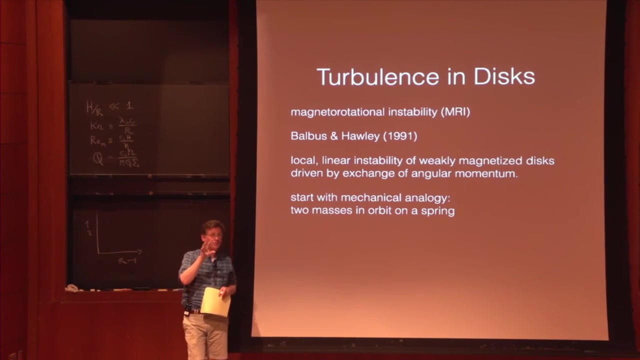 And it just oscillates stably. Okay, So this is directly analogous to the MHD problem, So let me Describe that here. So let's zoom in on the disk and consider a small patch of the disk in the poloidal plane. 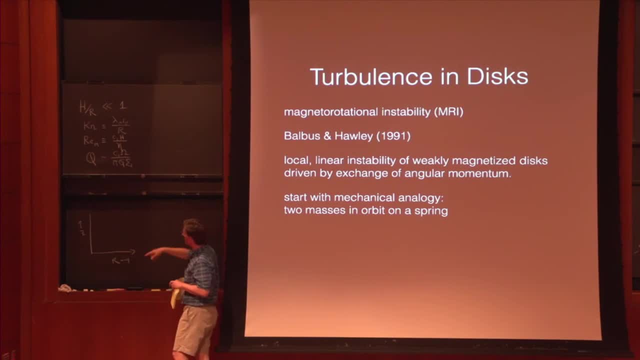 So the radial direction is this way, Vertical direction is this way. We're looking at a cut through the accretion disk And we imagine that the accretion disk is penetrated by a weak magnetic field. This instability corresponds to an oscillation. 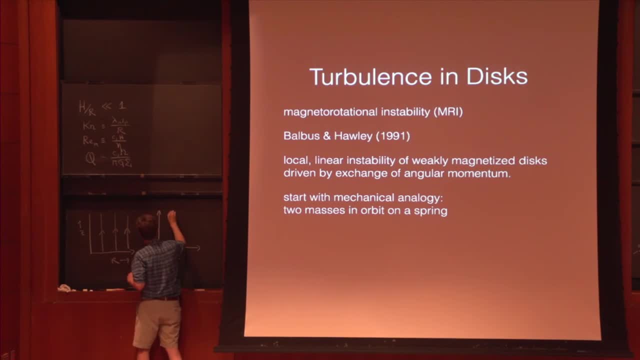 or unstable oscillation that looks like this. So there's one parcel of plasma at this height in the disk which is coupled to another parcel of plasma lower down in the disk by this magnetic field, And the field resists bending And the characteristic frequency of that bending. 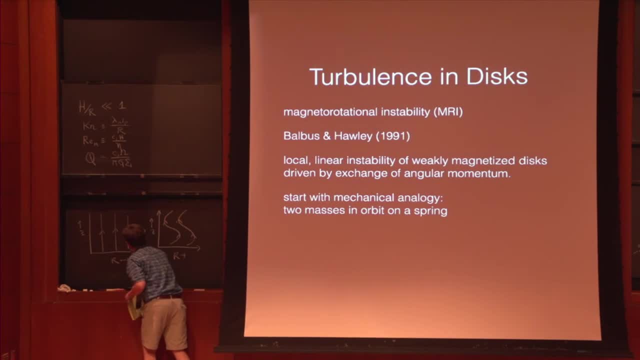 is gamma squared, is k dot vA squared. So k is the vertical wave vector, or it's the wave vector of the perturbation, And vA is the Alfvén speed. So, just to remind you, vA is B. 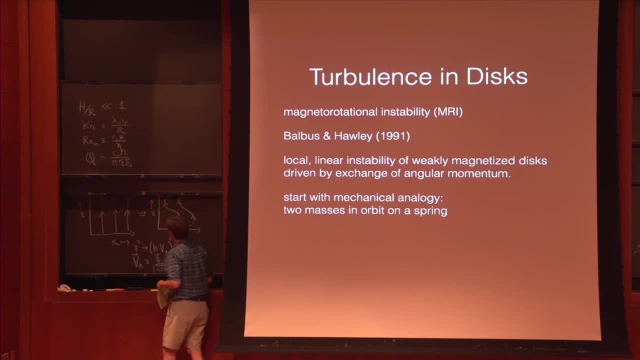 on root 4 pi rho. Okay, So this is the Alfvén frequency, And the Alfvén frequency squared is what substitutes for this spring frequency when one goes from the mechanical problem to the MHD problem. And so everything I've written down over here carries over. 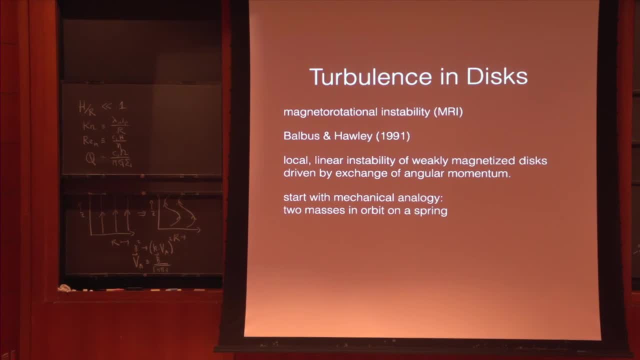 If one simply substitutes k dot vA for gamma, that gives the dispersion relation for a vertically oriented magnetic field- weak magnetic field in an accretion disk. Okay, are there any questions on that? Okay, So let me give a list of facts. 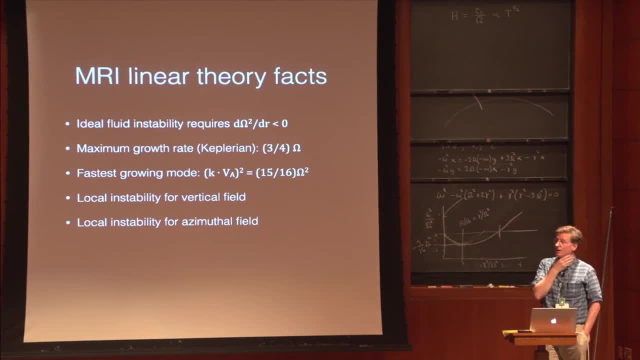 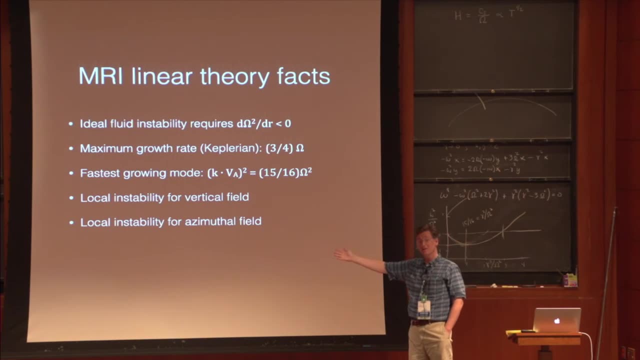 about what's known about the linear theory of this magneto-rotational instability, because obviously this is not a rigorous theory and this only considers a special case where one has a vertical field in the disk. So it turns out that for a general central potential 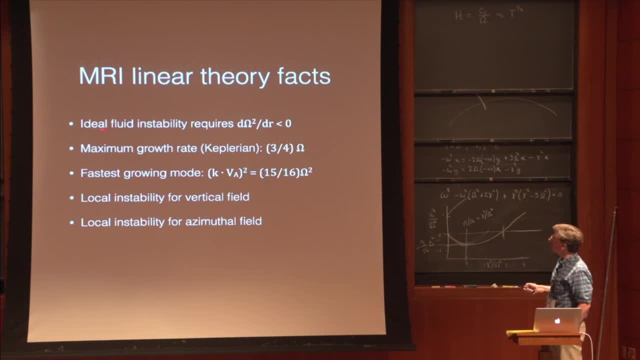 uh instability only requires that d, omega d, d, omega squared dr is less than zero. So there has to be differential rotation and the rotation frequency has to decrease outward Um. The maximum growth rate in a Keplerian disk is, as you could deduce from this: 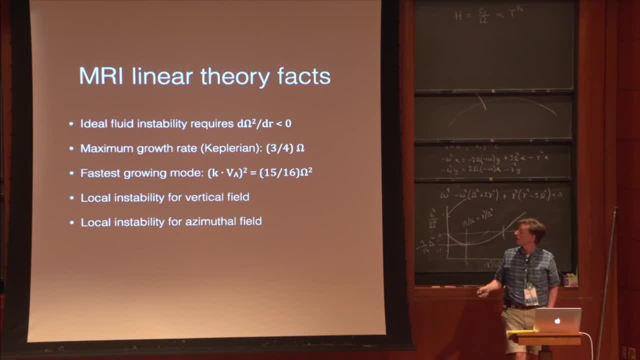 where I said the minimum in the dispersion relation is minus 9, 16ths omega squared is in a Keplerian disk, three-quarters omega. So the maximum growth rate is always the dynamical uh rate And it's obtained by tuning the wavelength. 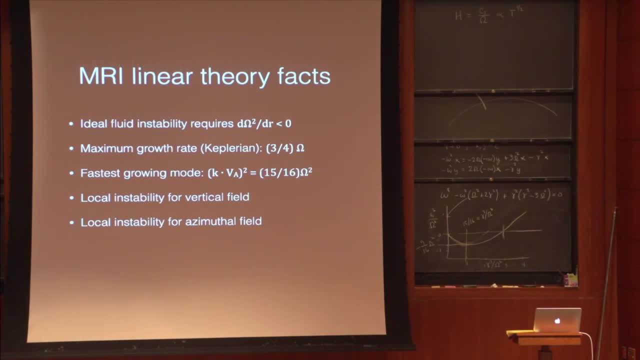 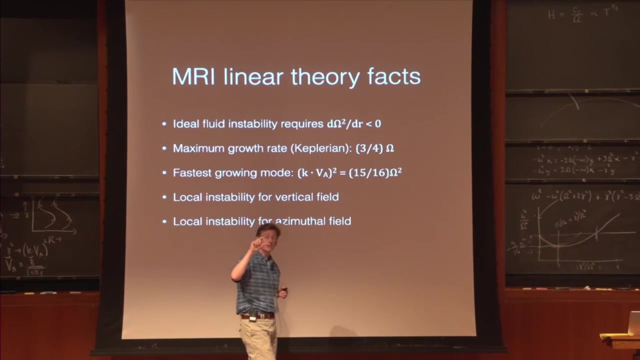 of the unstable mode, uh. so for, so that for a given magnetic field strength, uh, this k dot va is of order omega. So, for example, if the field is very, very weak, then the characteristic wavelength at which one obtains the maximum growth rate. 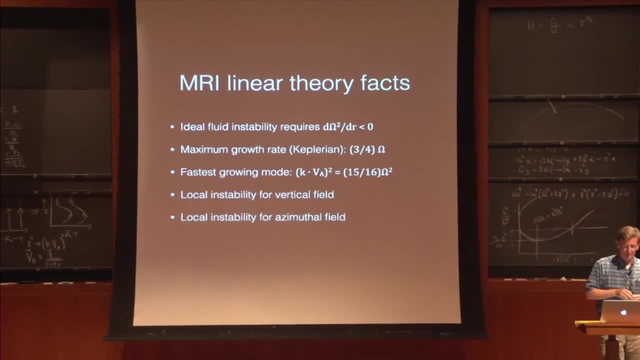 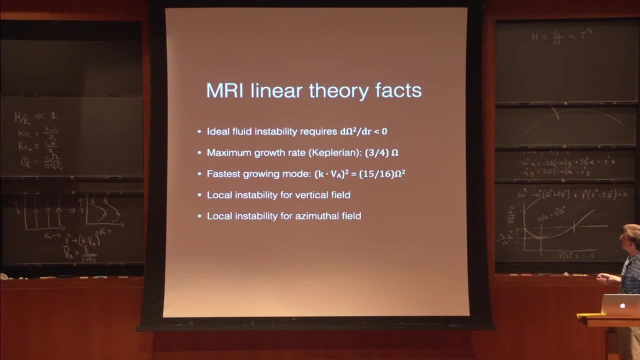 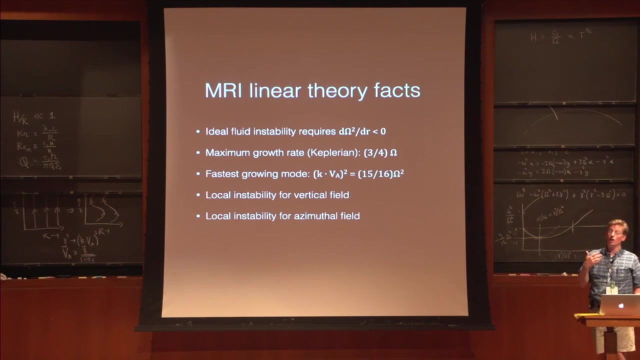 becomes smaller and smaller. Okay, Um, The fastest growing mode, as it says in the next line, is when k dot va squared is 15 16ths omega squared in a Keplerian disk. Uh, We know that there is a local instability. 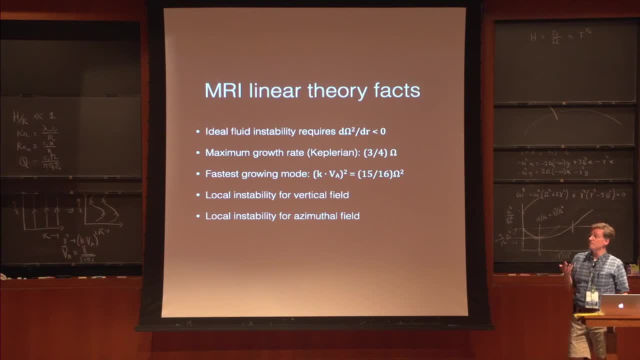 so local here mathematically means uh, an instability that appears in WKB theory, Uh, where the wavelength is small compared to the disk scale height, Um, and we also know that there is a form of local instability present even for a purely toroidal field. 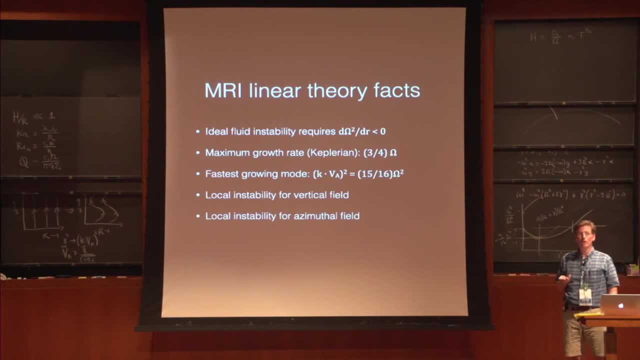 So in that case the linear theory becomes quite a bit more complicated and uh, and the instability manifests as uh, a temporary, uh growth in the magnitude of the perturbation, which eventually stops, But by tuning the parameters. 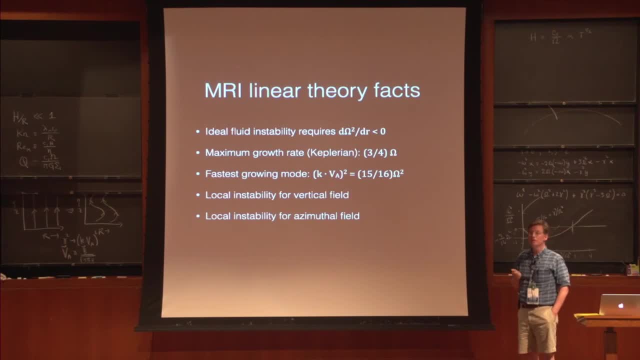 the wave vectors, it's possible to get as large an amplification factor as one wants, uh for any given toroidal field. Okay, So linear theory is great, but it doesn't tell you what happens when uh, the instability goes. 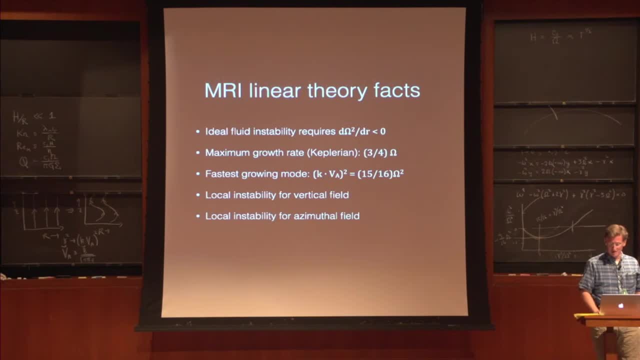 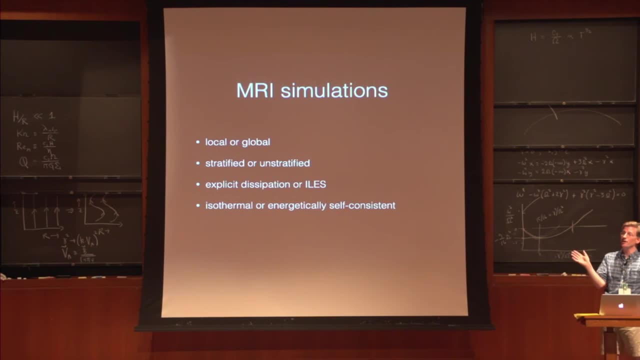 into the nonlinear regime and saturates. So for that, uh, we need simulations. Um, so there's there's lots of work been done on the development of MHD turbulence in disks over the last uh, 20 years, 21 years. 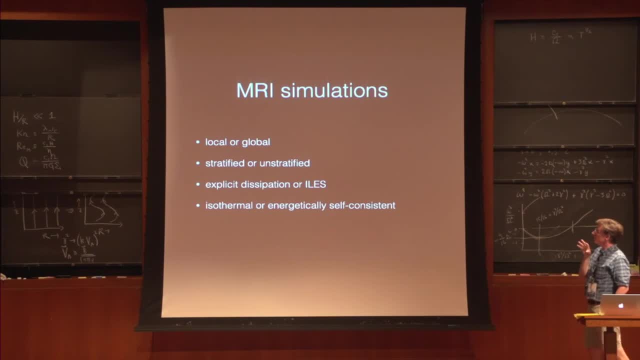 Um so uh, the saturation of the MRI has been investigated in local or global settings. So a local setting is uh one that basically uh follows a patch of plasma as it orbits the central object and uh uses a set of equations. 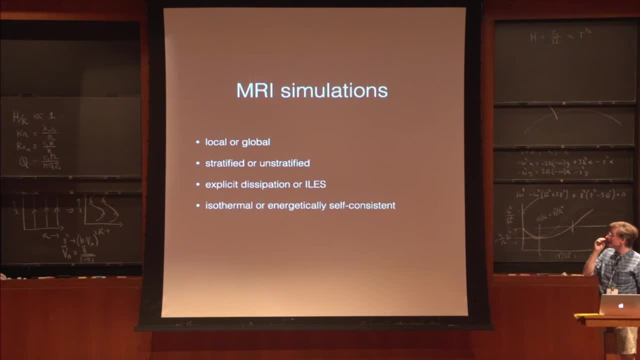 uh, inspired by the Hill equations Uh. whereas global models consider the full evolution of the disk from the central object um outward Um, MRI simulations in literature can be stratified or unstratified. So the uh, the stratified models simply include: 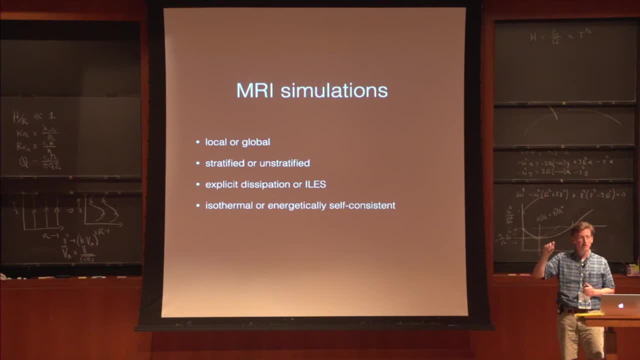 the harmonic uh potential around the uh midplane of the disk and so have uh variations in the density uh with height. The unstratified models turn that off and provide a simpler, cheaper model which may or may not be relevant. 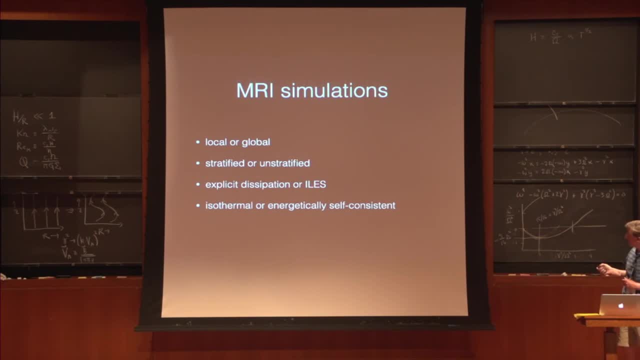 Uh. models have been run with explicit dissipation. So, for example, explicit and small uh. explicit and small viscosity, microscopic viscosity uh and explicit and small ohmic resistivity- Um or uh in the majority of models. 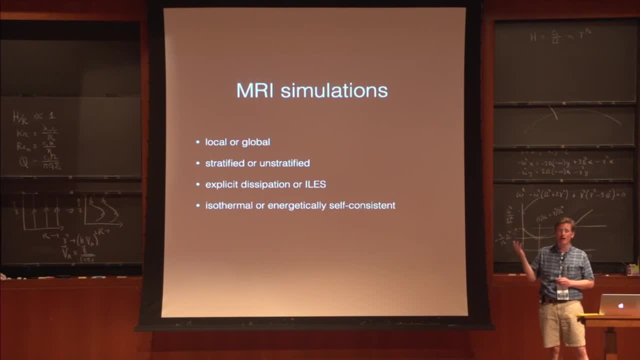 one uses something called IELTS, So I don't know if anyone's talked about IELTS here. No, Okay, So, uh, this amounts to what's called a direct numerical simulation of turbulence. So you simulate the entire, uh. 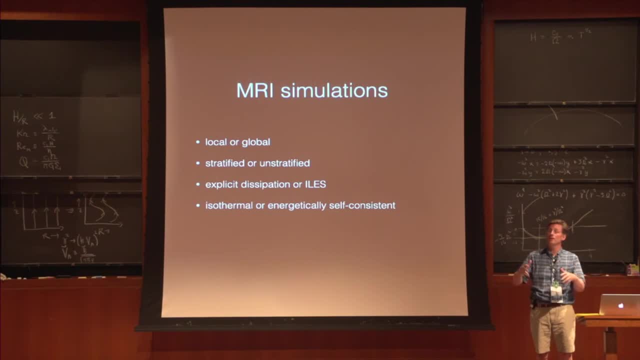 turbulent cascade from the largest scale, uh, where energy's injected scales comparable to the disk scale height- down to the dissipation scale. So you, you follow absolutely everything Uh in an IELTS model. uh, which means an implicit large eddy simulation. 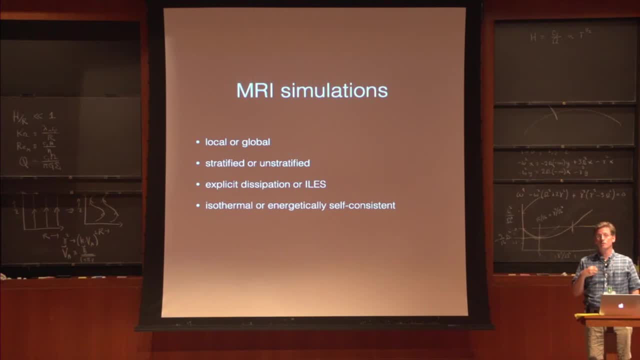 there's a closure uh which provides dissipation, And the closure is provided by your numerical scheme, Um. so most models uh to date have used IELTS And this this may or may not be a problem. We know that the convergence properties 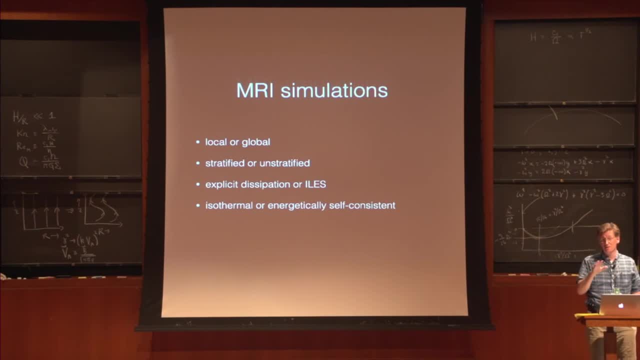 of IELTS and, uh, explicit dissipation models are different, So I'll I'll say a little bit more about that in a minute. Um, okay, And then, uh, people have looked at isothermal disk models, So isothermal just means. 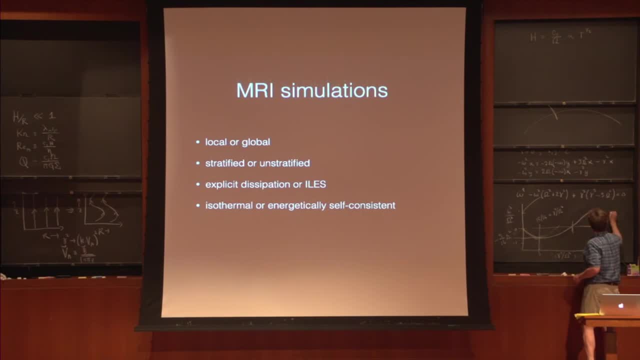 that, uh, one uses this equation of state where sound speed, squared, is a constant. This is the pressure, This is the density. Okay, So this eliminates the energy equation from consideration and gives one a cheap uh model to integrate. Uh, now people are doing energetically self-consistent models. 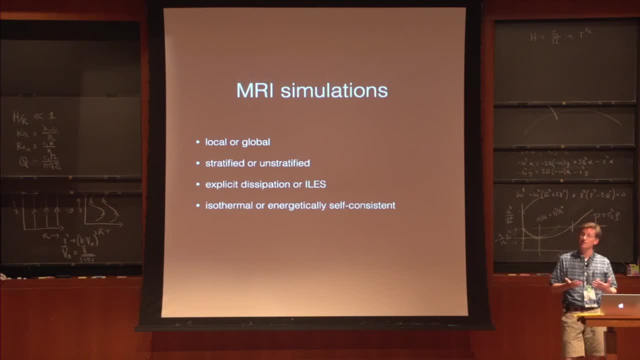 So either models with very little radiation, uh that allow heating, uh from dissipation of turbulence, or uh models which include radiative transport. Okay, So let me show you just a couple of models. So the first one is uh, a global simulation. 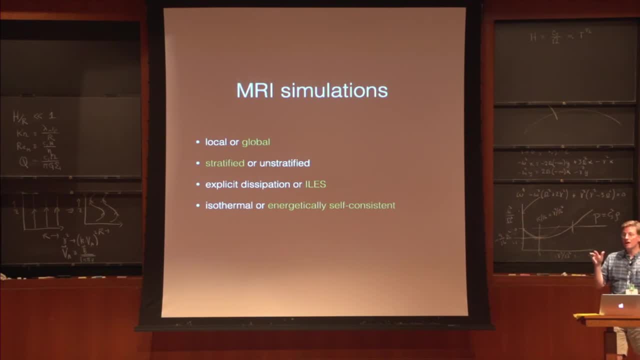 uh, that's stratified. It uses IELTS, So, uh, people sometimes describe this as dissipation on the bare grid. Uh, and it is energetically self-consistent In the sense that in this model, there's uh very little radiation. 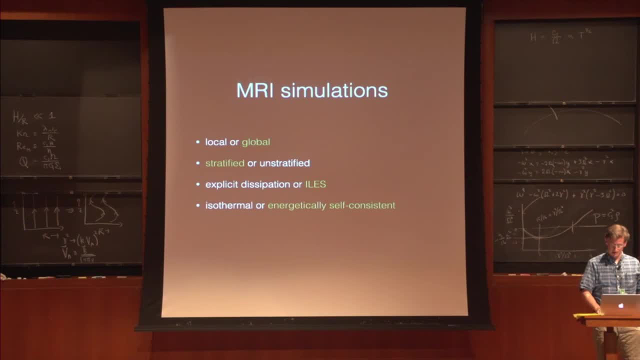 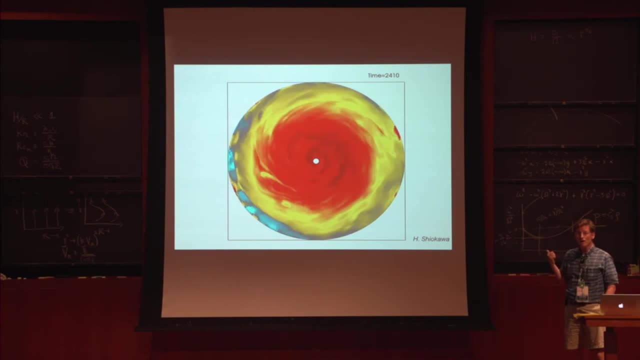 and the entropy of the plasma is allowed to increase. So, uh, this particular model is, uh was run by, uh my student, Hotaka Shikawa, uh, who's now at CFA, And uh it shows the density evolution. 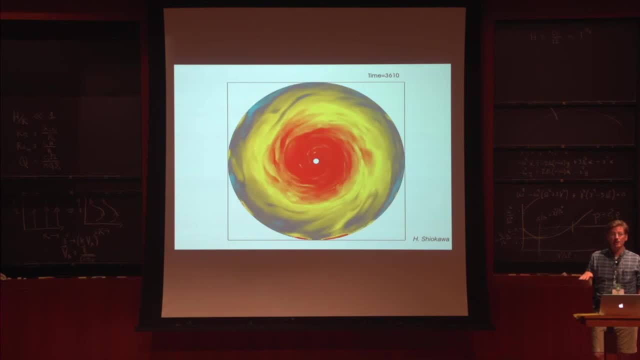 in the midplane of a disk around a rotating black hole. So you can see that, uh, there is sustained turbulence in the system that produces variations in the density in the midplane, and that these variations in the density take the form of trailing spirals. 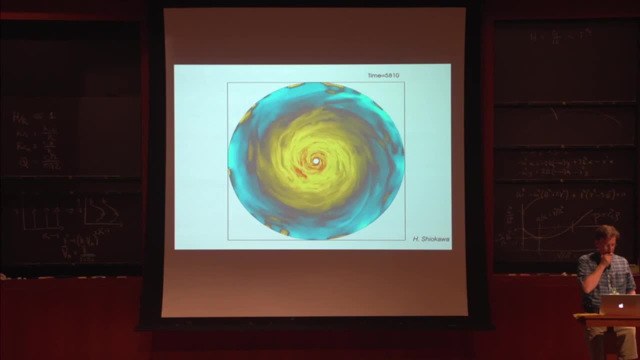 Okay, Um so, uh again. the color here shows a log of the density and this guy more or less reaches inflow equilibrium. In other words, it's been run through the viscous time scale out to a radius of about 20 times. 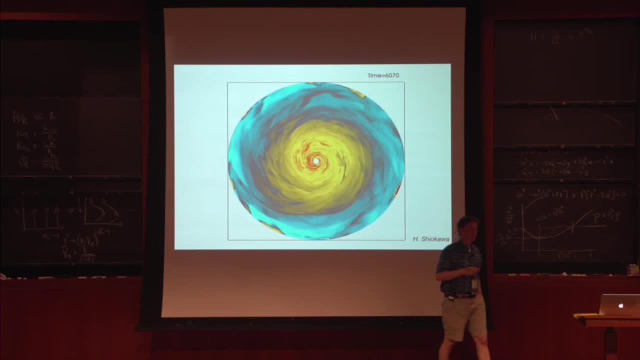 the event horizon radius. Okay, What's the weird? That's the boundary, Uh, so there's an outflow boundary here and, uh, uh, there's some interaction with the boundary. We know that it doesn't make much difference. 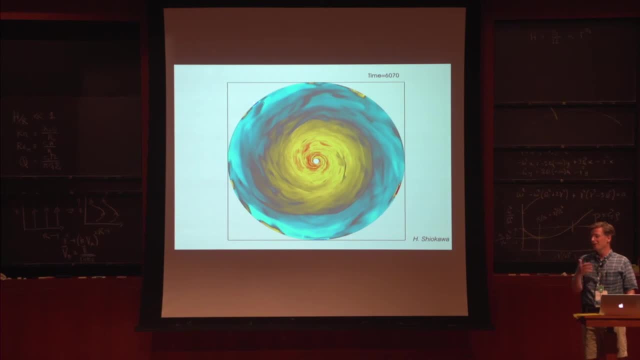 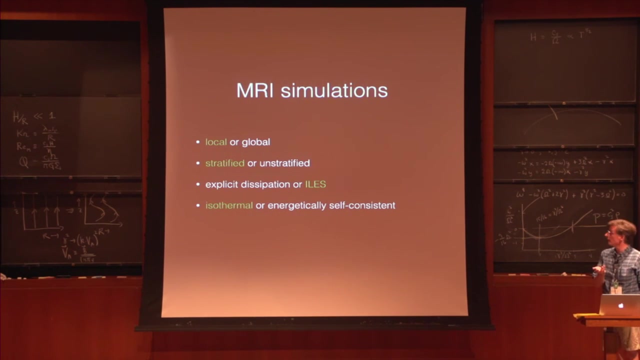 The outcome? because we tried moving the boundary and we get the same result. Um, okay, So, um. so the next simulation I'll show you is, uh, a local model. Uh, so it again. it uses equations of motion. 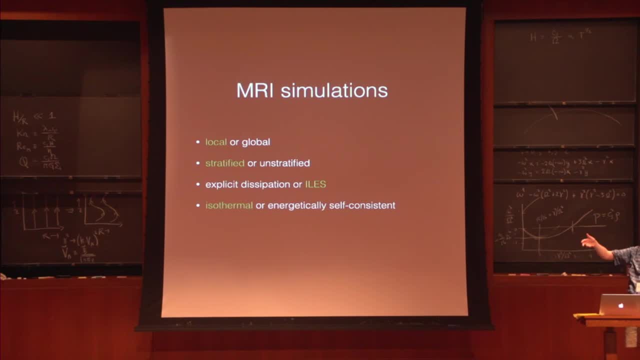 which include, uh, a Coriolis term and a tidal expansion of the effective potential in a co-orbiting frame. So we go into the frame of the plasma as it orbits around the central object. Uh, the model that I'll show you is stratified. 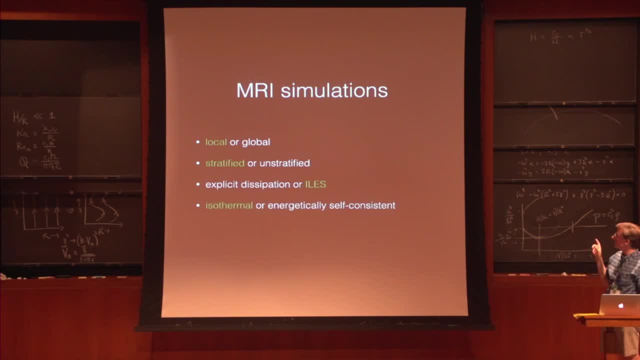 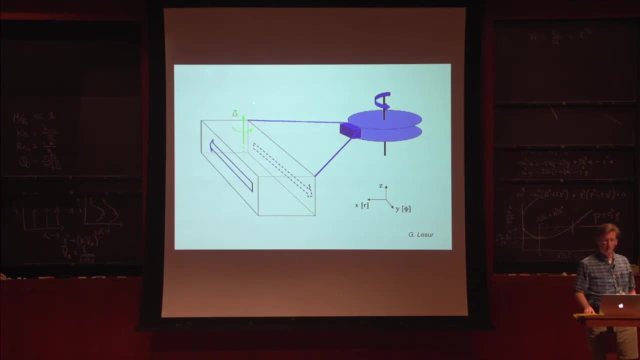 so it includes the vertical gravity. Again, it uses aisles or the bare grid, no explicit dissipation, and this one is isothermal. So so here's a? um a nice graphic from Geoffroy Le Serre. uh, that explains a little bit about what this local model is. 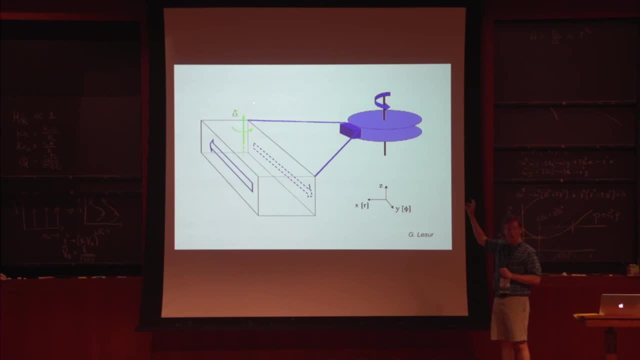 So we we pick a box that's co-orbiting, uh, with the plasma around the central object, and then we use a set of boundary conditions called the shearing box, boundary conditions which allow us to incorporate the differential rotation in the disk. 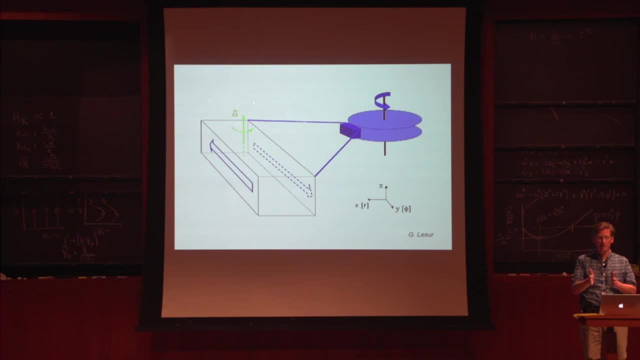 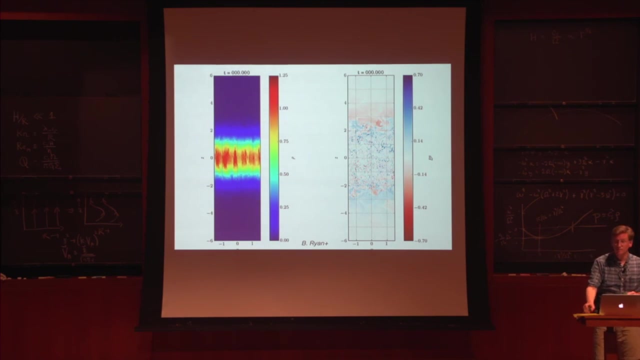 So it's really almost periodic boundary conditions, but the way in which the radial boundaries are connected is time-dependent and shearing, Okay, Okay. so here's, um uh, the evolution of the model. So on the left, uh. 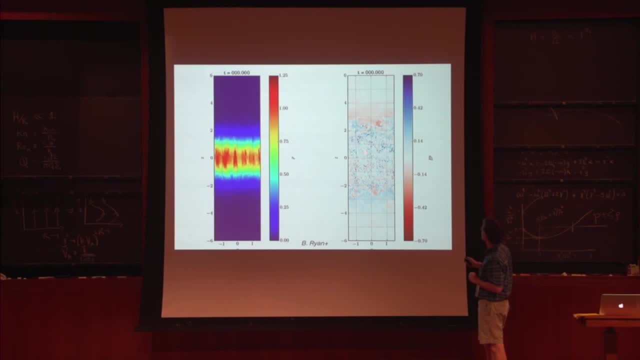 this shows the density, and on the right we see the the y or toroidal component of the magnetic field. And, and these are integrations done by my student, Ben Ryan, recently, this this spring, Okay, so um. 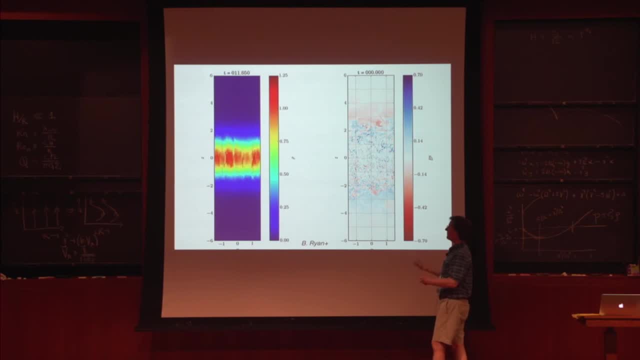 you can see that, uh, there's something going on in this disk. Uh, there is uh turbulence which couples to compressive modes and produces these density waves that run back and forth inside the disk. Um, let me show the uh. 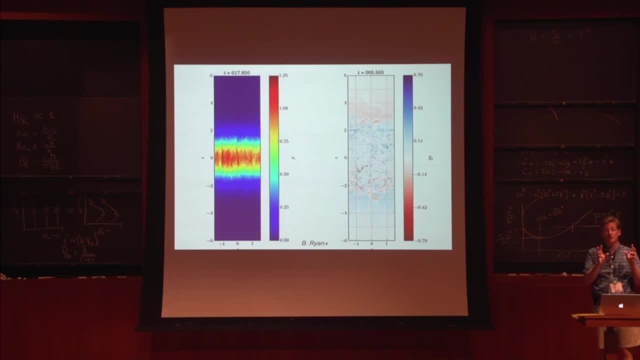 the field. Uh, you can also see that there are small-scale structures in the magnetic field And, uh, uh, these lead to an alpha of order. uh, a few times 10 to the minus 2 when vertically integrated through the disk. 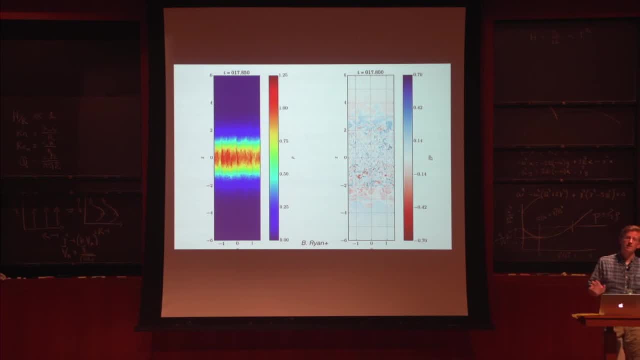 Okay, so these are just examples. There are- I think there are hundreds of papers which have looked at, uh, these, uh, similar models in the literature. Uh, and a few things have been learned from these. Uh, not as much as we'd like. a few things. 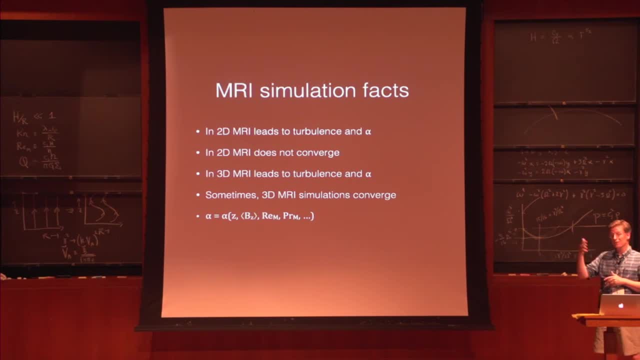 Um, so, going way back in history, the first models that people ran were axi-symmetric models, and we know that, uh, even in axi-symmetry, the MRI leads to a turbulent state and uh, and that that turbulent state. 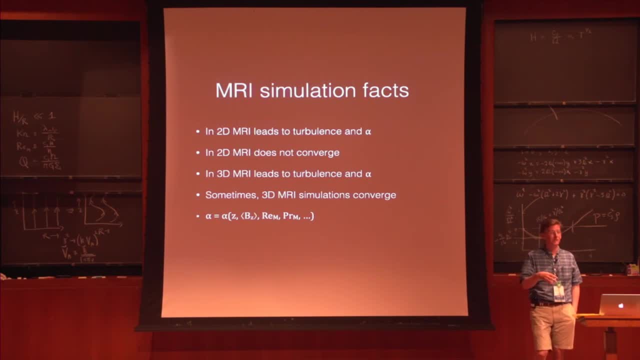 transports angular momentum outward. And that statement that angular momentum goes outward is not a trivial one, because there are some forms of turbulence which transport angular momentum inward. So, uh, so that's interesting. Uh, we know that in 2D the MRI does. uh, 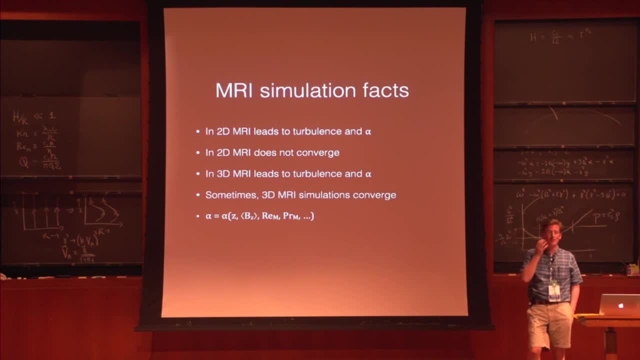 does not converge. In other words, even if you have infinite numerical resources, uh, you will not find a converged value of alpha. Um, we know that, uh, in 3D the MRI leads to turbulence and, again, outward transport. 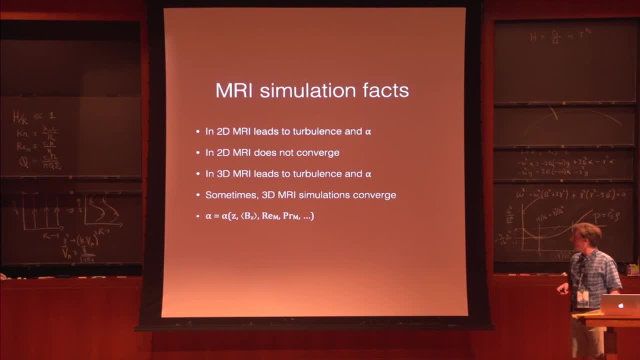 of angular momentum. Uh, and we know that sometimes in 3D the MRI simulations converge. So we know they converge when explicit dissipation is used. Uh, we also know they converge when- uh, in one of these local models. 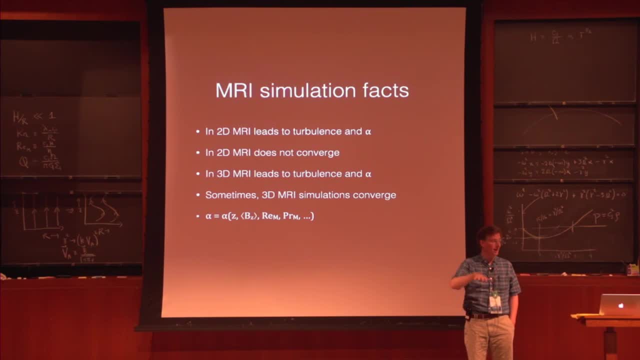 one inserts a vertical magnetic field, uh inside the box uh, or a permanent toroidal field. So in either case the simulation uh converges. We know they don't converge in the unstratified shearing box models. 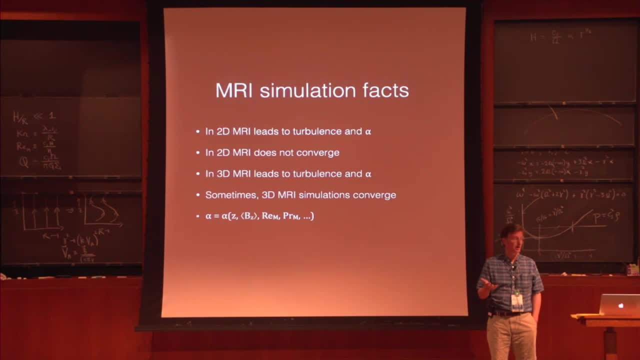 on a bare grid in the IELTS uh problem. We uh there's something discovered by Fremont and Papaloisou Uh. we know, uh that there are issues with convergence for IELTS models in the unstratified shearing boxes. 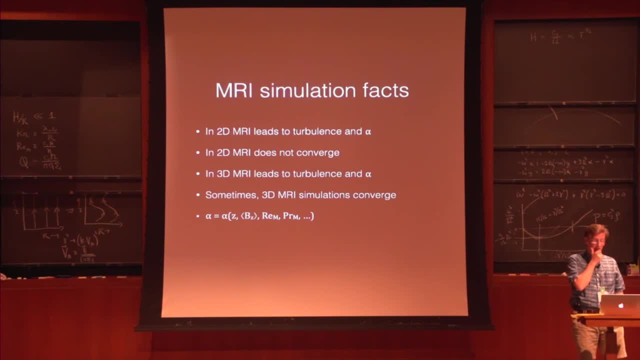 And we also know uh that in the global models that have been run to date the characteristic scales of the turbulence are not very well resolved. So one can measure a correlation length for uh density and magnetic field structures and those correlation lengths 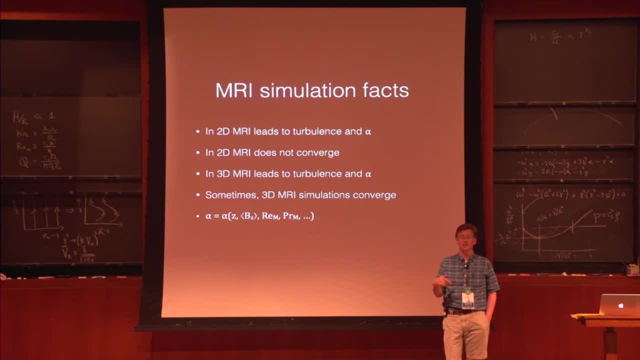 tend to be, uh, tend to change as the grid scales change, as the resolution changes, So, uh, so the news there is mixed. Uh, we've also learned that the intensity of the turbulence depends on several things. Uh, so, in particular, 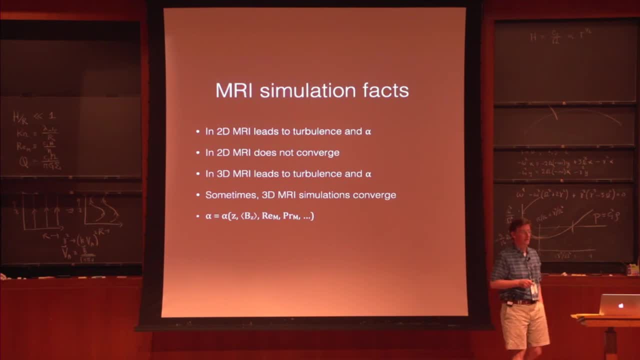 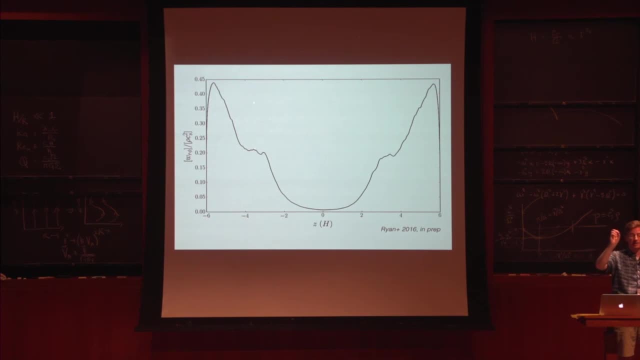 we've learned that it depends on height in the disk. So let me show you, uh, the run of alpha, which is the, in this case, is the ratio of the shear stress to the local pressure. Okay, so this is the run of shear stress. 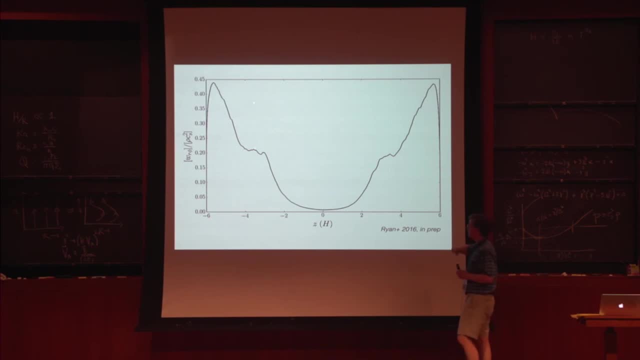 to local pressure in the one of the local models that I showed you as a function of height through the disk, in units of the scale height, And you can see that, uh, at the midplane here alpha is about 0.01,. 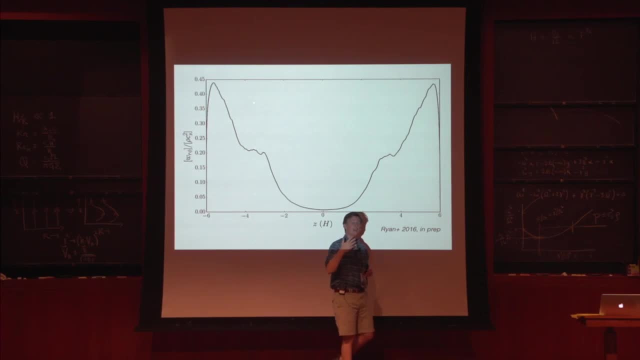 and then, as one goes up away from the midplane, alpha increases And uh, a couple of scale heights above the midplane. it's a few tenths. So this is quite interesting and was not envisioned, I think, in the original um alpha models. 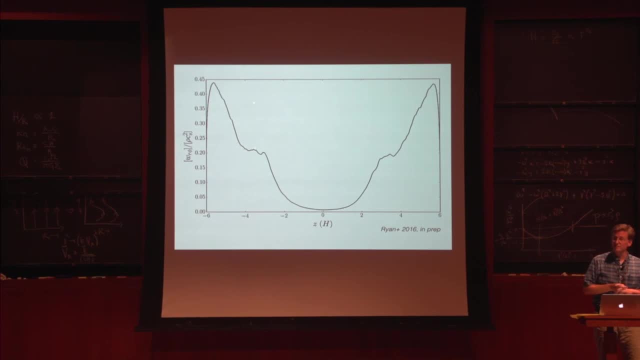 from the 1970s Question: Yeah, Is that H a like simulation unit or is that the actual like temperature scale height or pressure scale height? Um, well, so I think those are the same thing here. 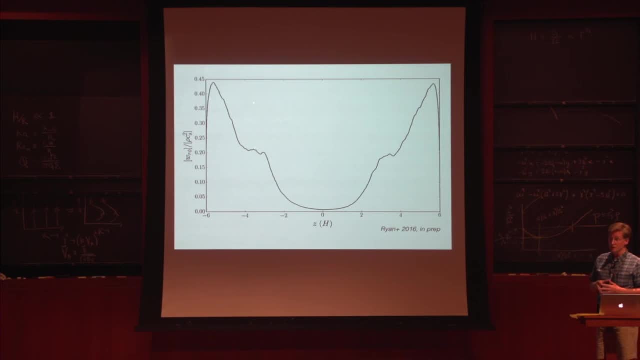 So it's. it's Cs, the sound speed divided by omega, And in this simulation, uh, the equation of state is isothermal. so that may be what you're, yeah, Um, so this is an isothermal model. 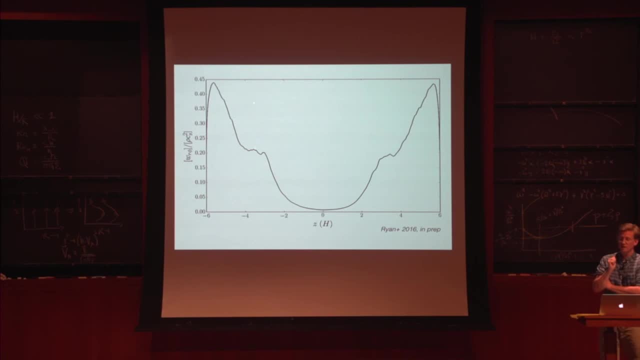 so they're the same. What's R in this case? Sorry, what's Uh R? So like H over R, So so that H over R does not appear as a parameter in the local model. So you've sort of expanded it away. 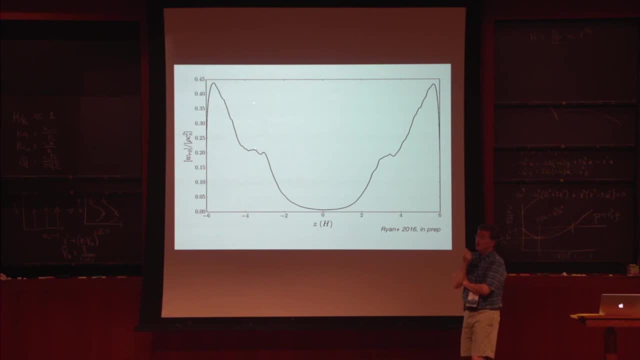 Uh and uh. because you've done that, the local model becomes very simple. There's no curvature present. Uh, everything is rectilinear. Uh uh, Cartesian Schrodinger box. Okay, so we also know that, in addition to depending on height in the disk, 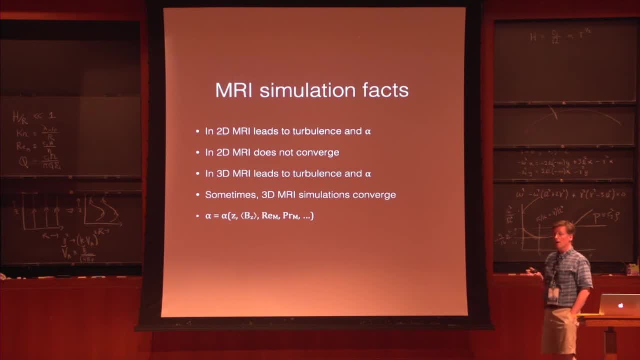 alpha depends on the magnitude of the vertical magnetic field that threads the disk. Um. so this uh, the sense of this dependence is that as one increases the strength of the vertical magnetic field, the intensity of the turbulence increases. Um, and this, this may be connected.